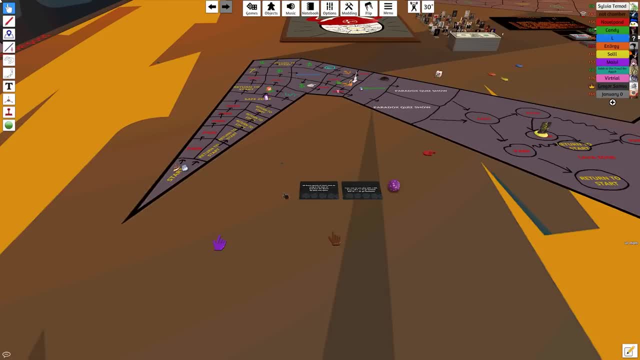 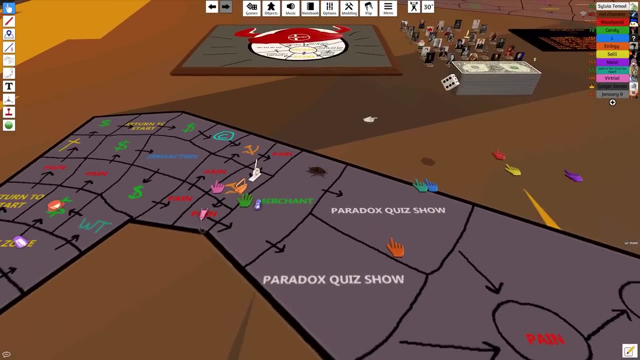 Because I didn't tell any of the players the rules either. I gathered together a whopping 10 people to play this game and I told them absolutely nothing. The plan was actually to just have them roll the dice and play the game, and when anything came up, I explained how it would work. 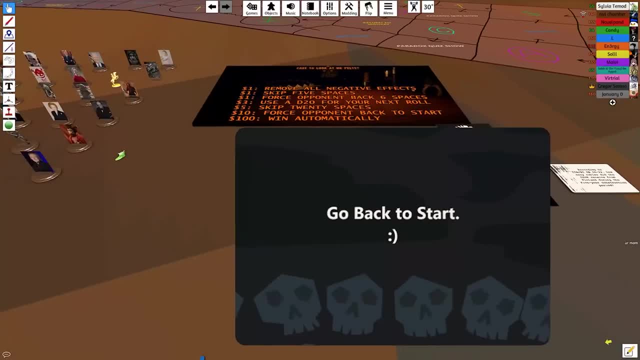 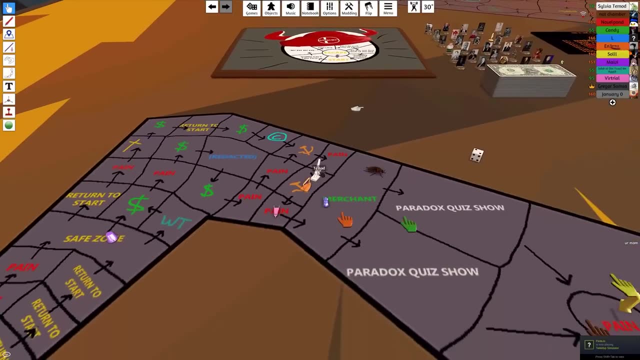 That means I also have a good explanation for all of the mechanics, like what cards you draw and what extra boards you go to, just embedded in the video by default. so I'll leave the rules out of the intro and you can pick them up as we go. 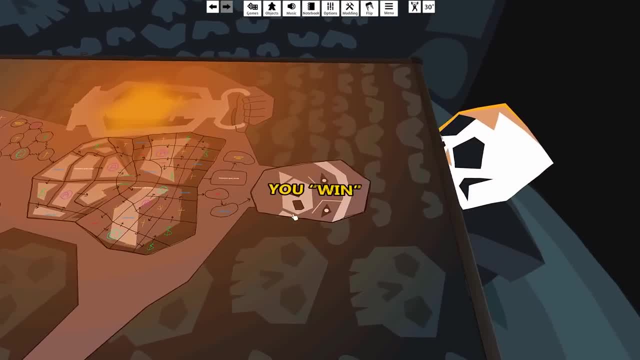 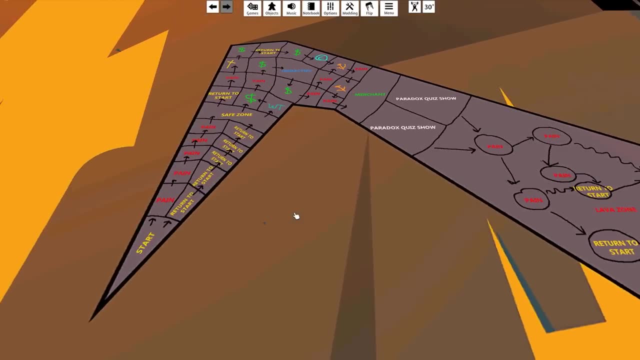 All you might want to do is- That's pretty obvious- Your goal is to get to the end. You roll the dice and you move your piece in the direction of the arrows. Simple enough. I should mention, though, that three of these 10 players did participate in a test beta game. 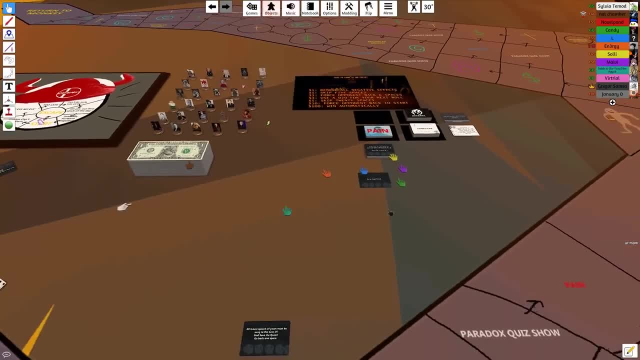 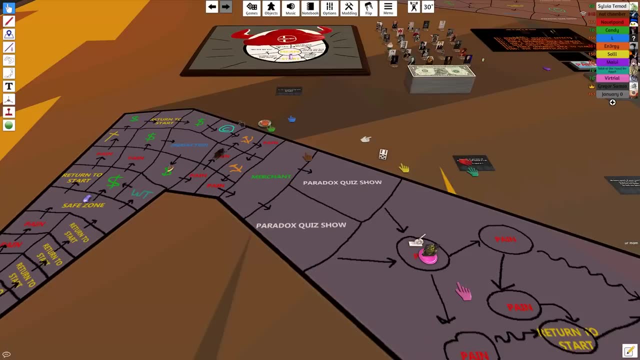 Because, as I suspected, the game was very unbalanced and actually impossible to complete. Thankfully that one test run allowed me to refine this into a playable experience. This did mean a few people knew what was in store, but they didn't bother warning anyone else anyway. 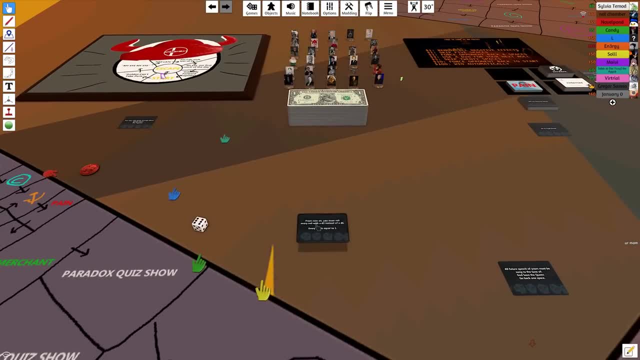 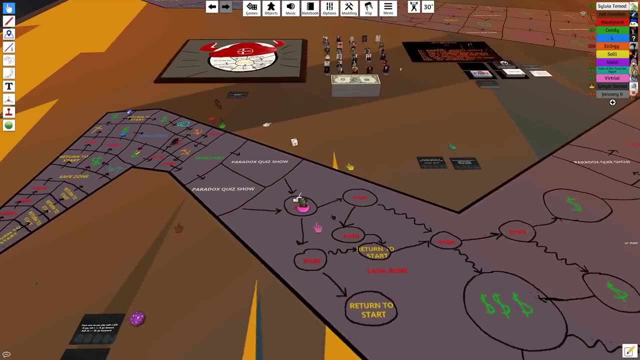 I should also, As always, warn you about microphone quality, which will become pretty apparent at times. It's actually not anywhere near as bad as it usually is, given that there's like a dozen people on this call, But occasionally those people who live down a well and are using an antique radio as a 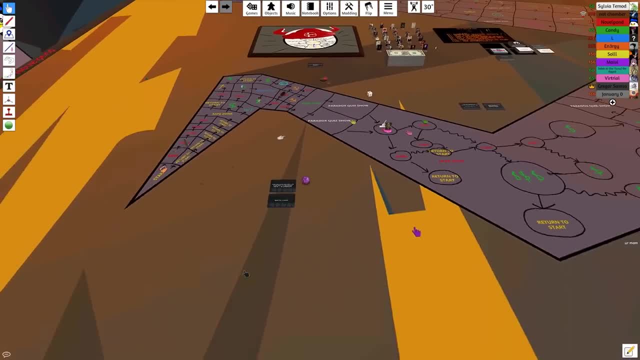 mic on Discord will seep through. With that, however, I think we're pretty much good to go. Let's get this circus started. Yes, but we're actually forcing maybe to play because she's hungover. That's the point. 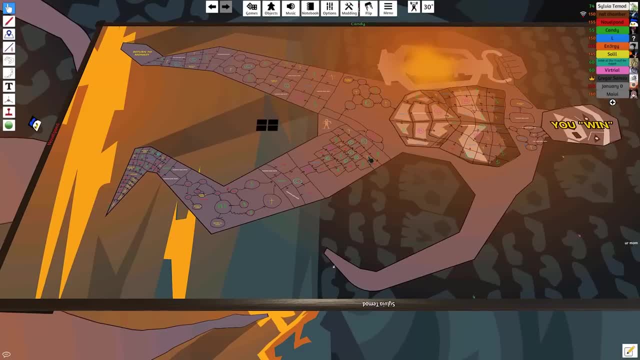 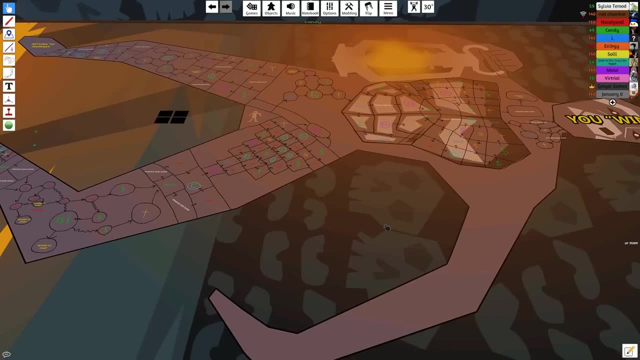 The entire point of the video is to make, maybe do things while hungover. That's the point. That's why we're doing it today. Shall we begin? Yeah, listen, the fuck up. All right, sit down. You may notice there is absolutely nothing on this board other than the board itself. 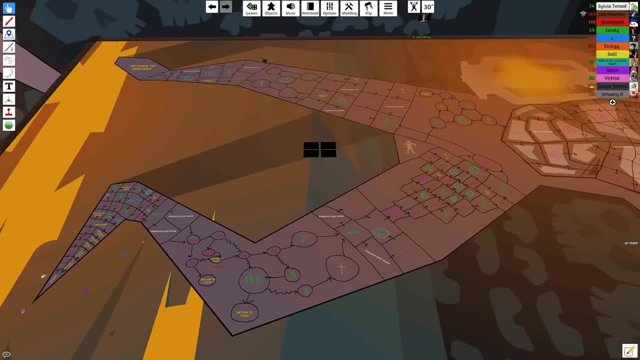 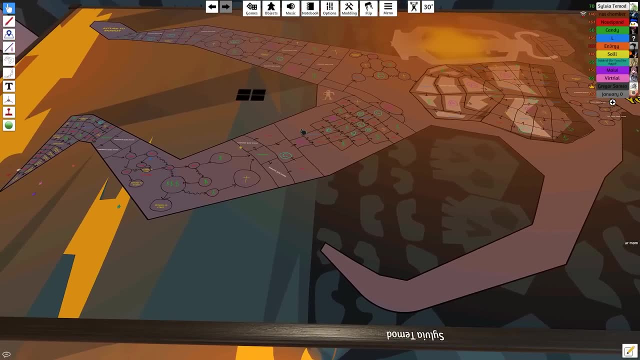 There is no cards, There's no piece, There's no pieces, There's nothing at all. This is because I have everything saved as an object that I can drag into the game And, as we go, I'm going to introduce mechanics as things happen. 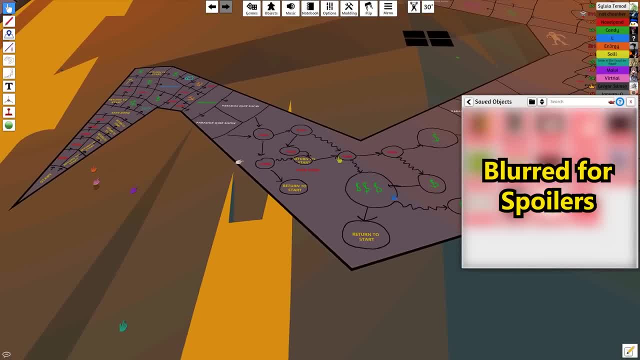 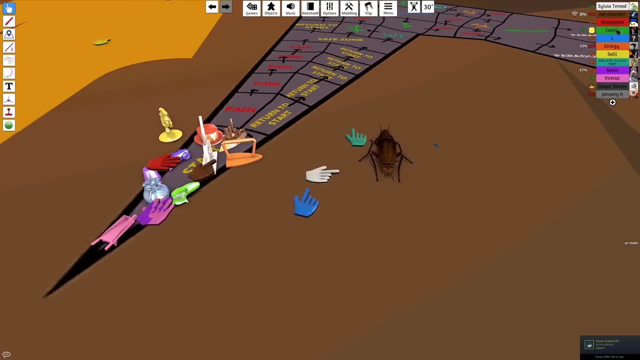 So first we're going to need to pick a piece for you, So let me just drag those in. Oh, candy, candy, Spawn in the piece you used yesterday for me. There's candy. There he is. Can we put the top hat on the cockroach? 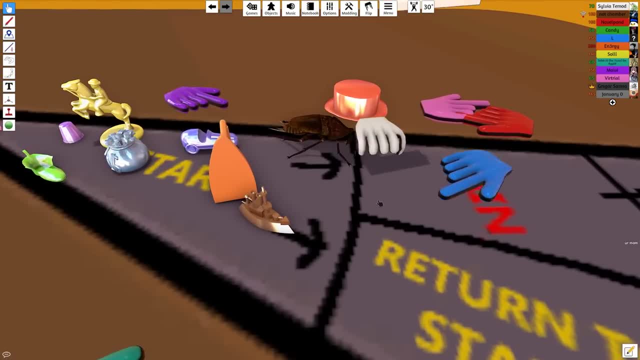 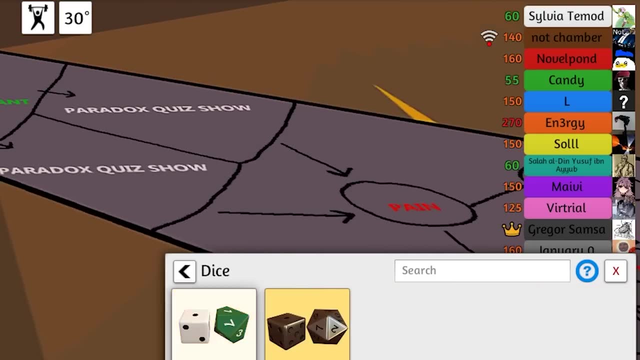 Look, it's the Smithing Britt. Oh yeah, Look, there he is in the flesh, or the exoskeleton. I guess I'm going to spawn in. We're going to just go in order from top, which means Tmod goes first. 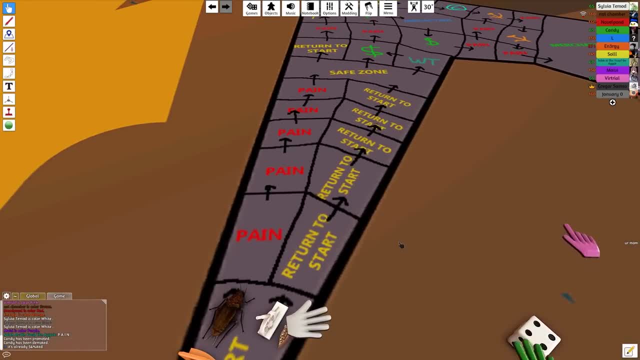 Four, Just like that. There you go. There you go Four. So you have two paths to pick. It's up to you. Pain You'd like pain? All right. Time to bring in the pain card, All right. 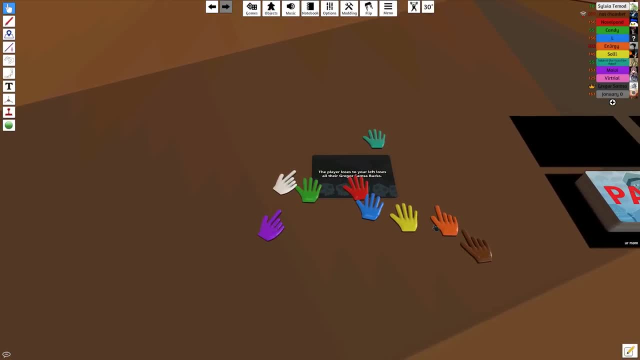 Now I will draw, Let's see. Oh shame. Well, that's introducing a mechanic we haven't gotten to yet, which is the Gregor Samza buck. I hate this, Right. Well, we haven't done that yet. 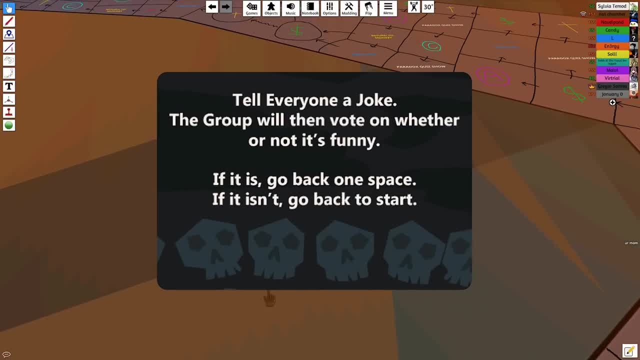 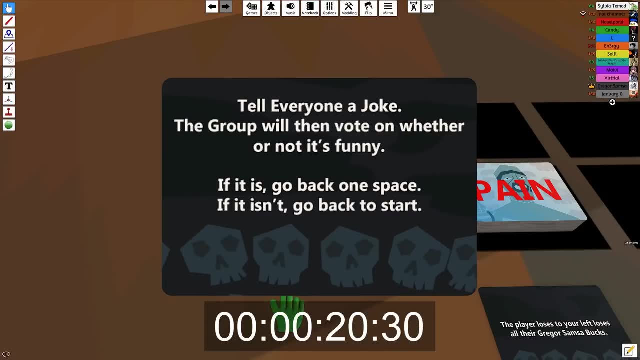 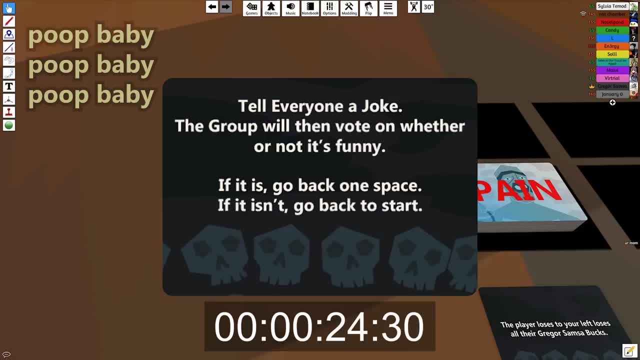 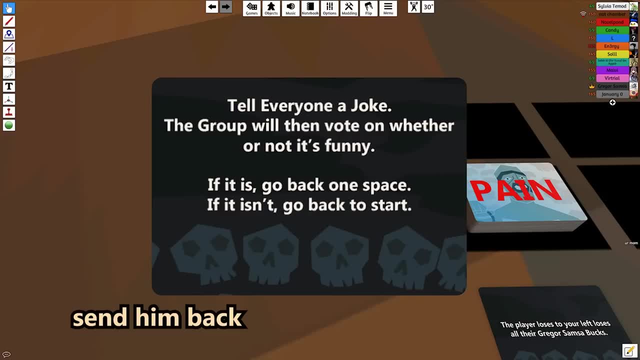 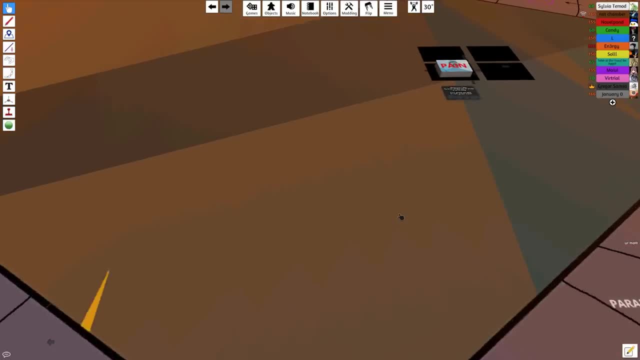 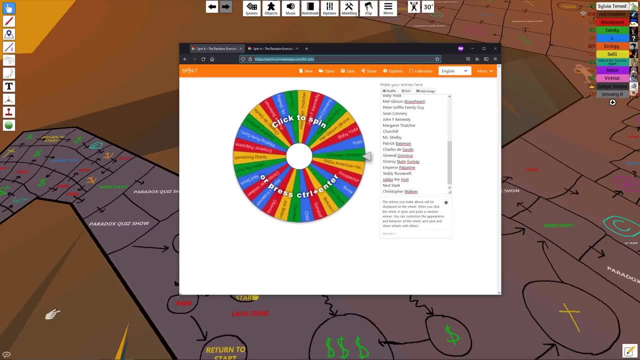 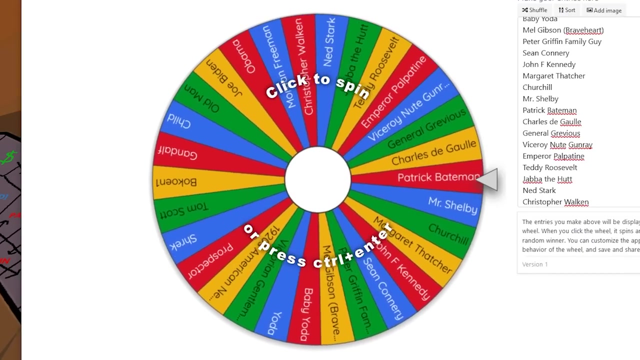 Send him back. You know what? I'll have it back. Let's pull this card off and see what you get. Oh, We get to introduce the character wheel. All right, listen, I have a wheel of funny characters. If you have to spin the character wheel, you then have to until your status has changed. 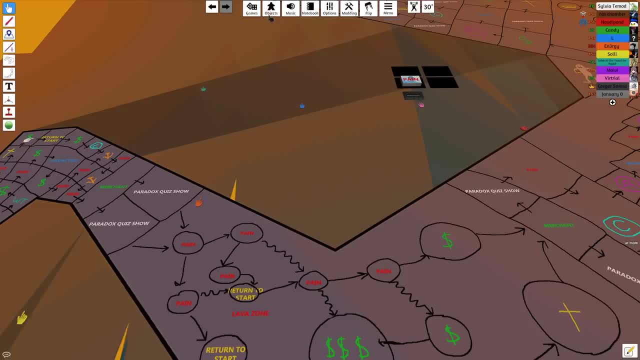 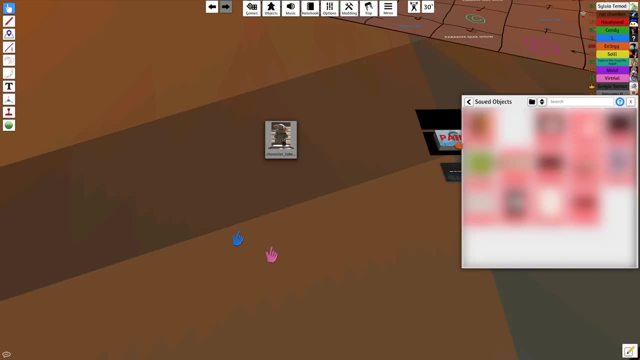 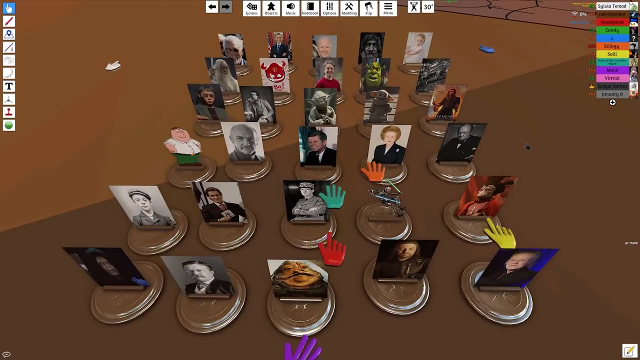 impersonate the character Oh Mike, Also before We also have a new thing that was aliśmy, Oh my Today from the beta testers: uh, your, your character. your token is going to be replaced with one of these. you will, you will be impersonating one of these funny characters for the rest of the time. 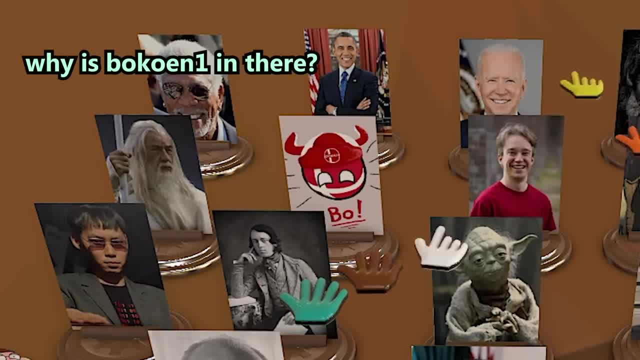 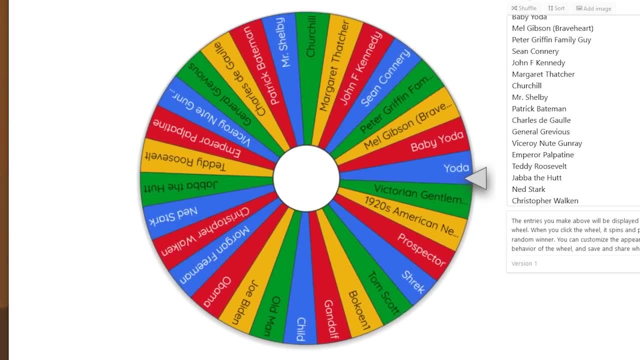 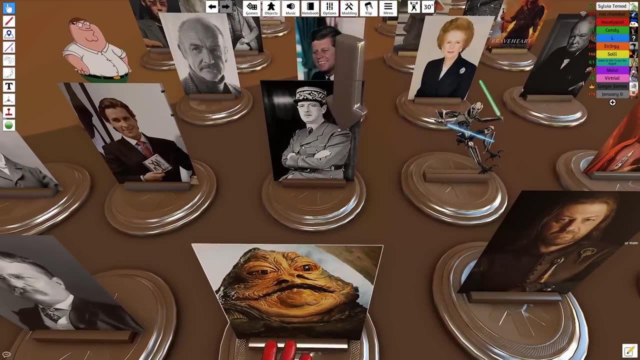 he's right there next to tom scott and joe biden. oh, oh, very unfortunate candy. you've rolled yoda. why is charles de gaulle here? what do you mean? who speaks french? charles de gaulle's a funny character. charles de gaulle on right. charles de gaulle right in between general grievous and patrick. 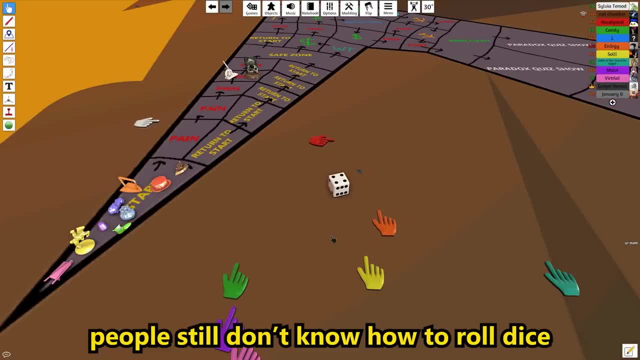 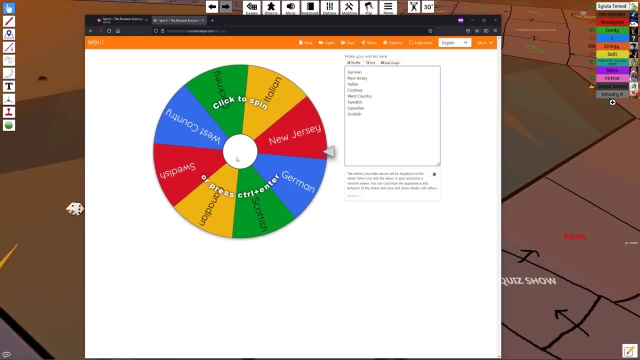 baitman, click and drag, click and drag and then press bar. oh, now we get the uh, the accent. well, now, no, here's the thing we decided was that character wheel and accent wheel, uh, surplant each other. so if you have to spin either of them after already having one, your new one replaces it. 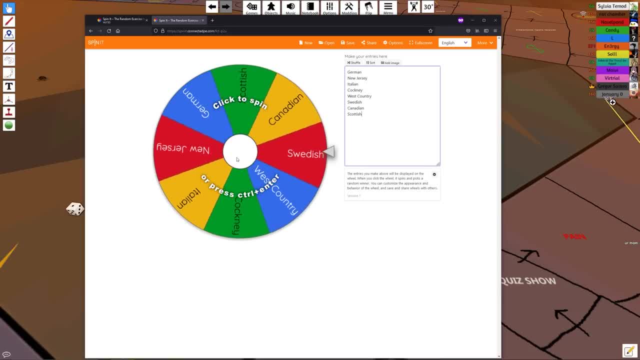 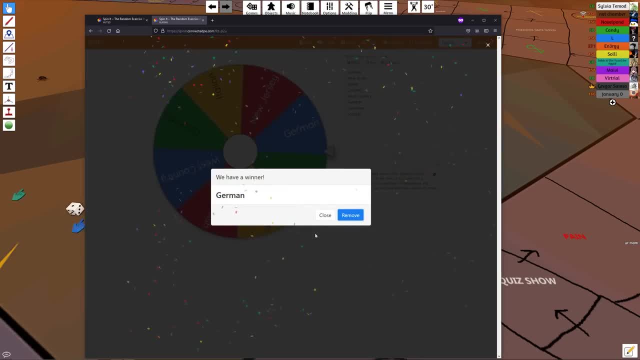 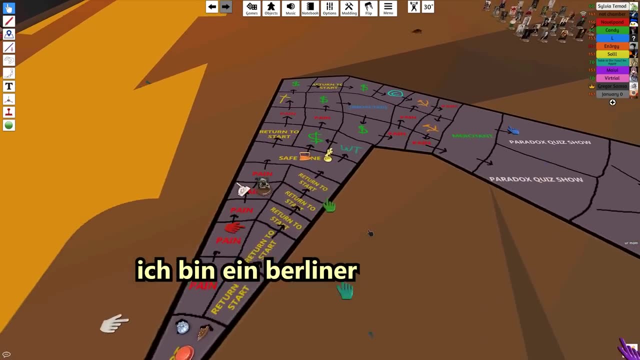 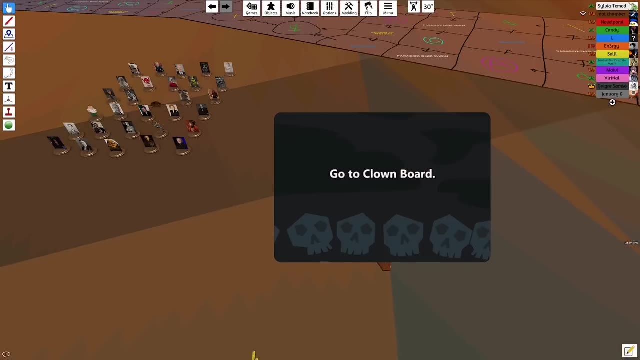 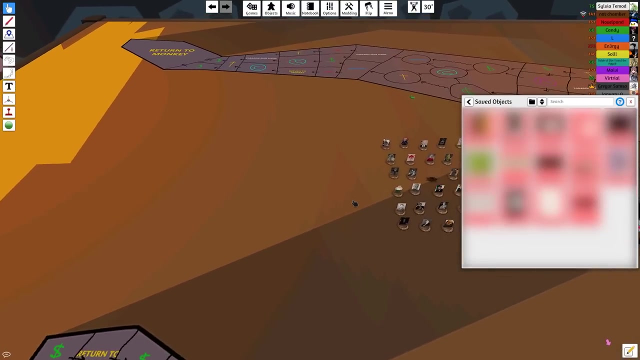 basically just can't speak. oh, congratulations, teddy. you will now be speaking in a funny german accent. okay, you know what pain it is. i'm scared. oh, unlucky, unlucky baby, it's time to go to the clown board. you're going to the clown board until you can get to the escape circle. 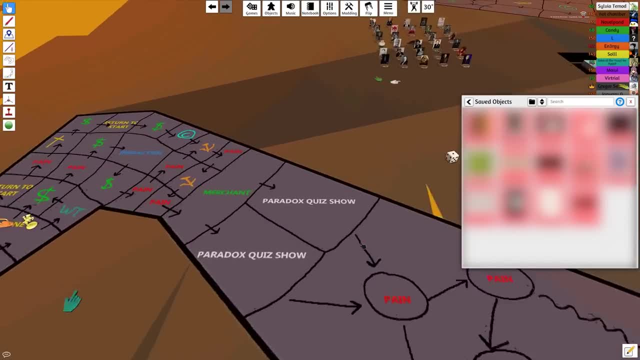 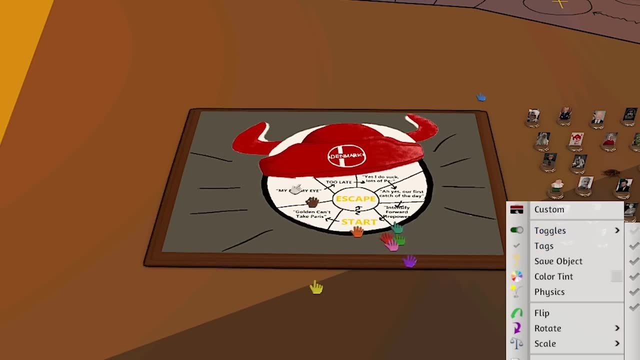 uh, when you get to the escape circle on the con board, you get to go back to the start of the- uh, actual board. let me just pull in. let me just pull in the con board for us. this is beautiful. now i also have to explain. you see this squiggly line here. 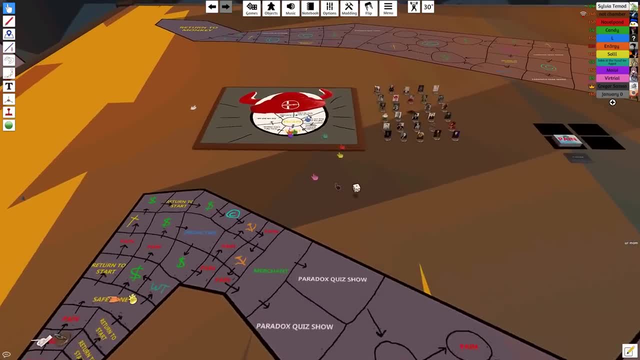 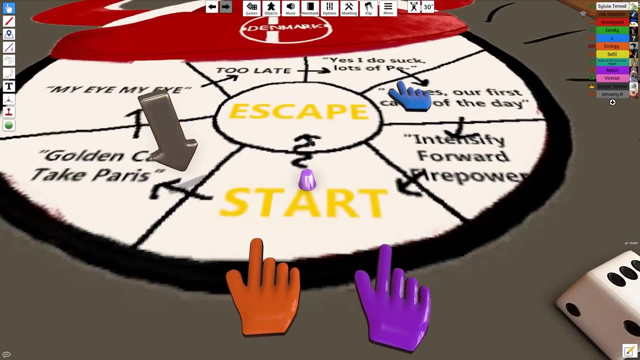 a squiggly line is only a way you can go. if you land on the square, keep going round and round until you can land on start. then you can either pick to keep following that or you can go that way. oh my god, are there multiple clown boards? yes, in other words, you can go to the escape circle. 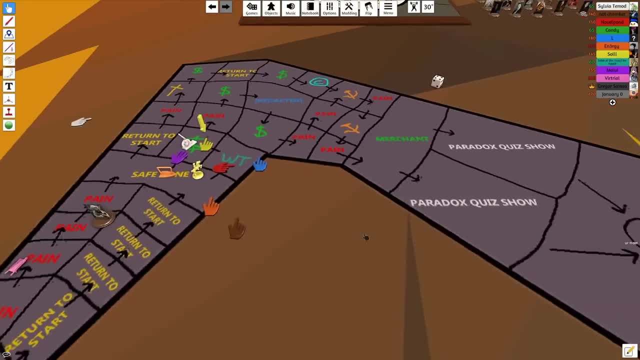 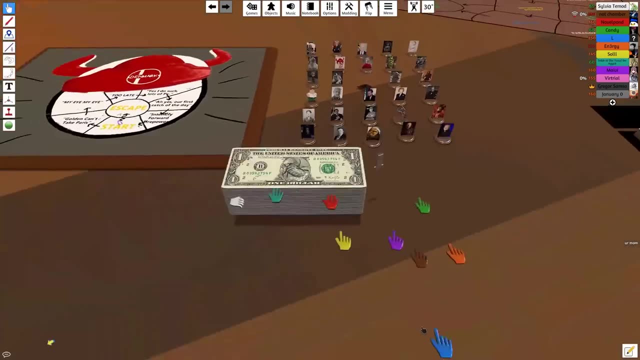 you're going round and round in circles until you land on start again. ah, it's time for you to get your first gregor sam's a buck. let me just pull those in. oh, gregor sam's a buck. there it is signed by kafka himself. i like the fact that this note isn't legal tender, for all that's public i put. 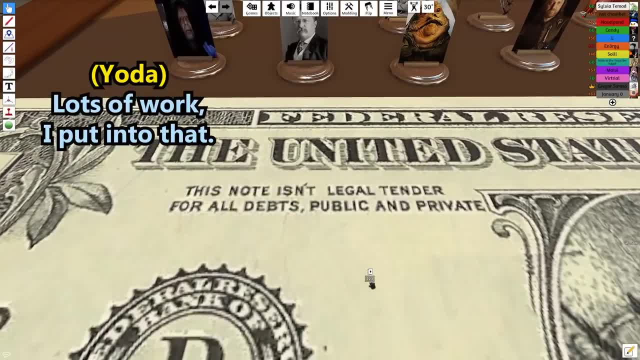 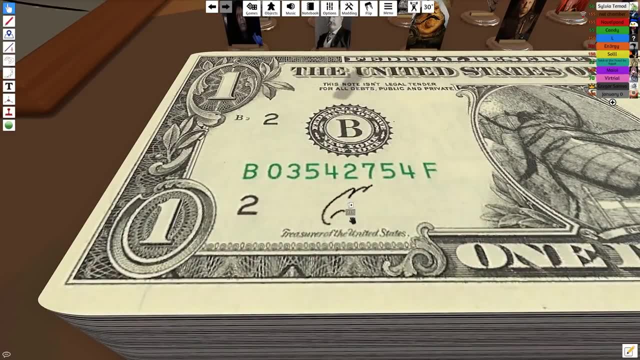 into that. can? he made this? you'll notice he actually sent me an updated version with the correct apostrophe on that text. i also forget who who's the who's the other guy- the treasurer of the united states. what signature was that? again, i'll see. oh, it's good. 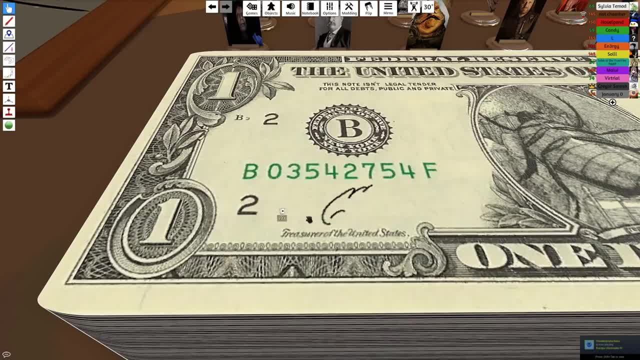 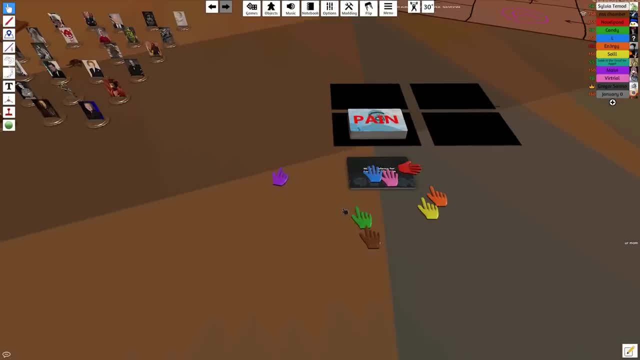 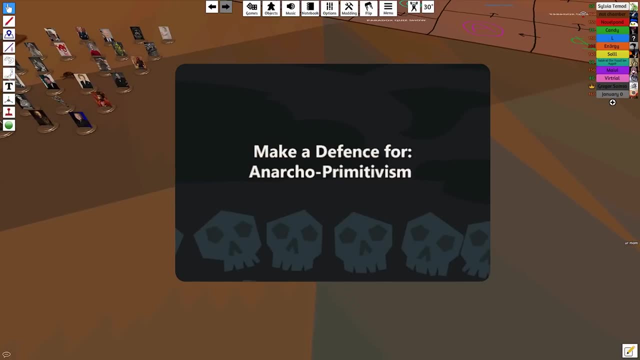 i am on pain. i'm in pain. all right, you need to make a defense for uh, anarcho-primitivism now, and if it you don't defend it, well enough, you go back to start. my main defense is: i fucking hate money. i just i hate, i hate legal tender. can we just like go back to bananas and rocks he wants? 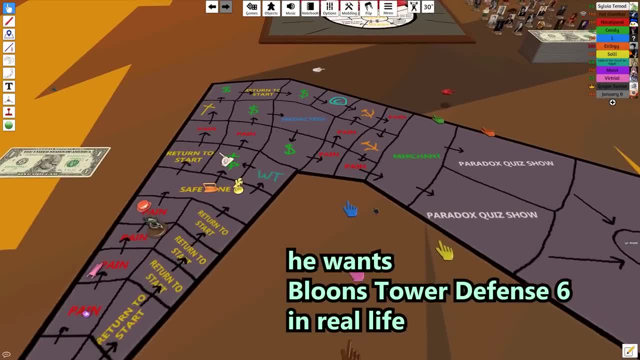 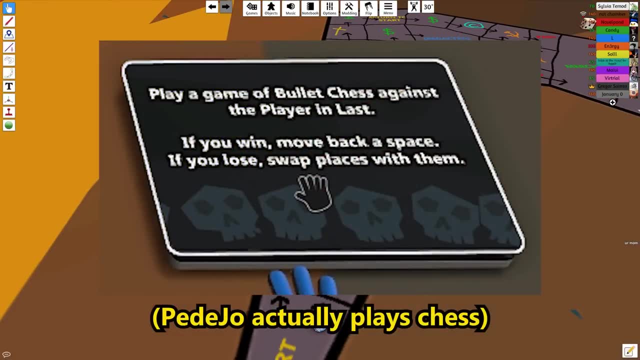 bloons tower defense six, and really i do. we're gonna go for pain, okay, oh, that's really unfortunate. to get that against pettish, though you have to play bullet chess against teddy, oh yes, play against me. oh no, chamber because chambers. and last he's on the clown board. 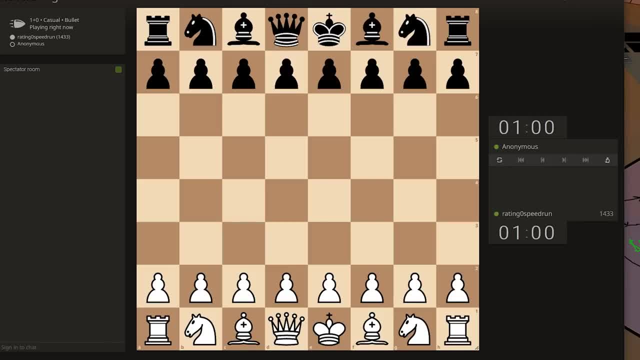 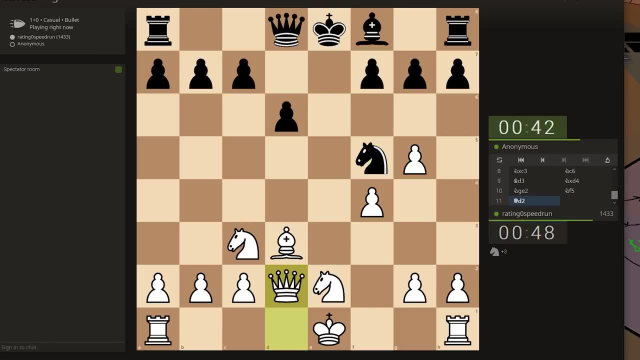 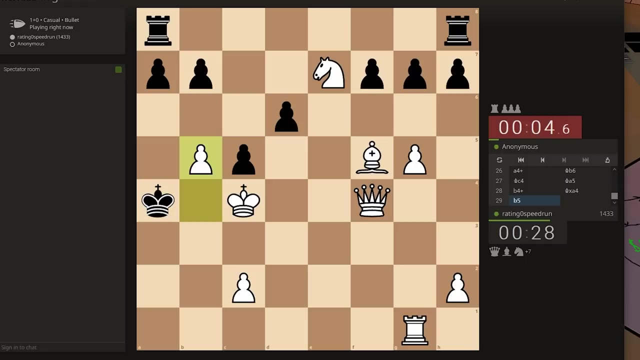 yeah, i think if pettish somehow loses he'll be sent to the clown board. that's true, oh my god. yes, i like the silence. it's pretty good, we're watching. i'm just moving my horse. as you can see black, black off flagged. all right, so that means pettish. oh, what real surprise there that the 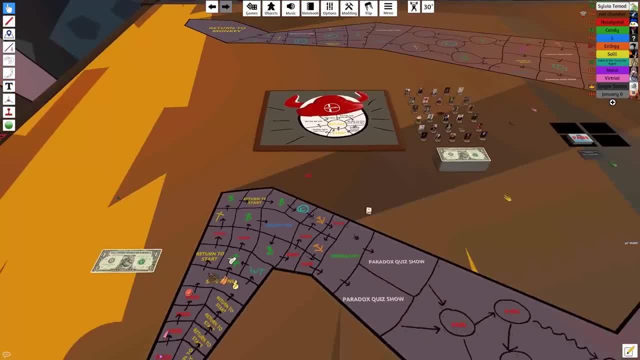 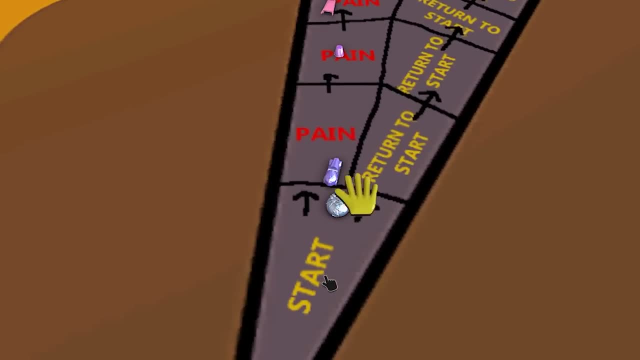 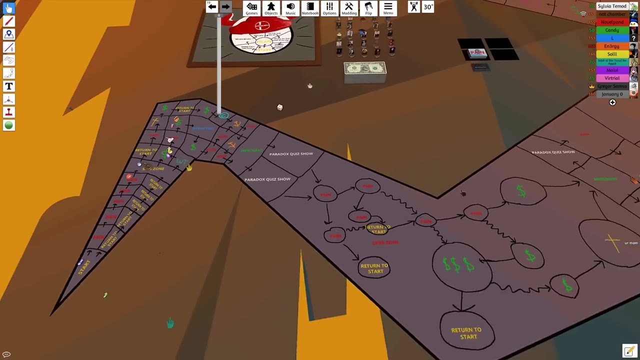 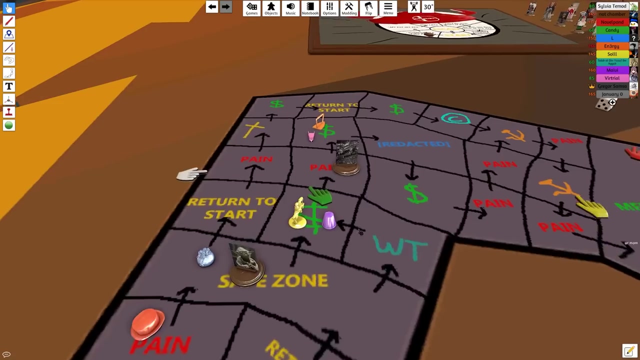 person rated 1800, rapid one against an anonymous player. so if you win, you move back a space unfortunate. uh, back to the game. you can spawn banana. i will shut up, yoda. go back to the swamp. you fucking swamped, gremlin. oh, you're on the clown board. i. 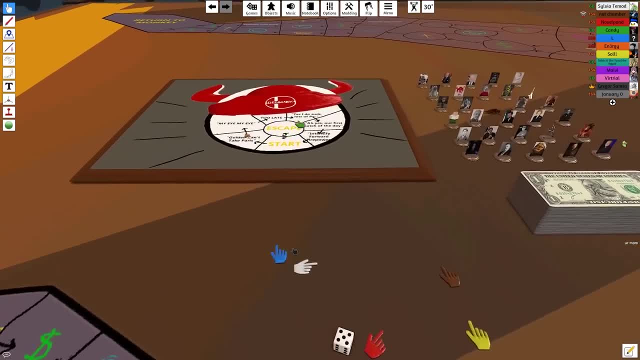 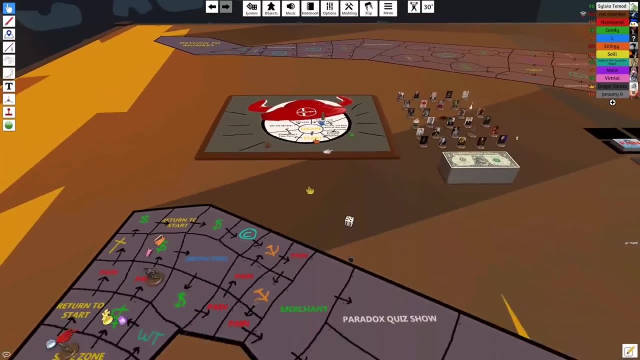 forgot. those are all direct quotes from the uh bocone one page on the aux cast wiki. uh, except that one. what does it do, though what? what does it mean, though? nothing. oh, you were simply going around in circles until you get to leave, actually. no, you just timed out 10 minutes because of the spam. 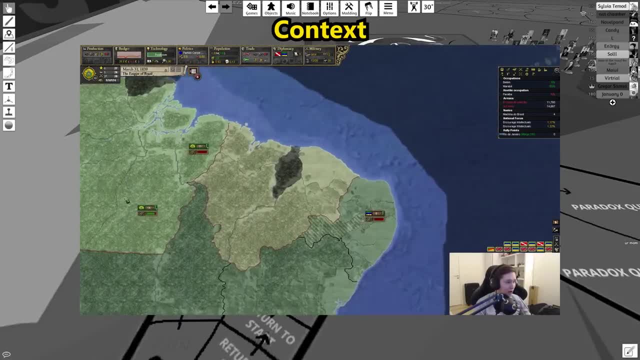 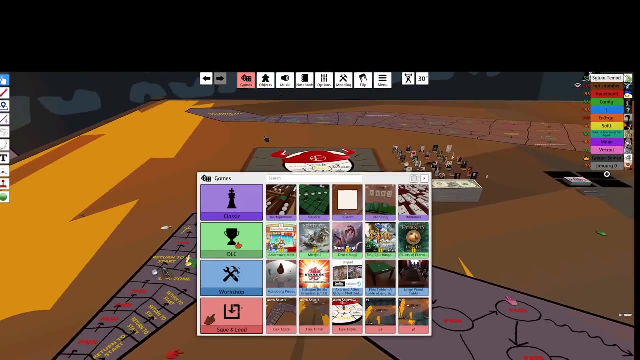 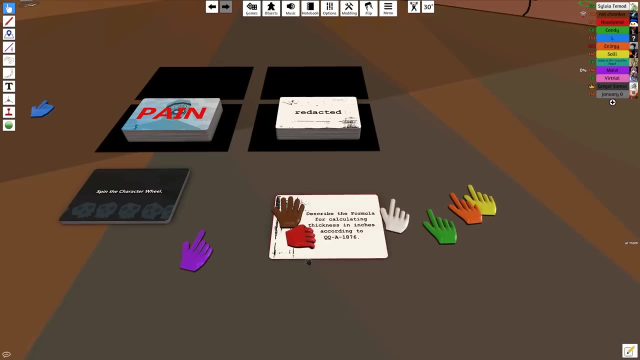 i'm reactionary. candy fang for the one. i do suck my policies. i can allow slavery. oh, you're unredacted. okay, now it's time to explain uh, one of my favorites uh types of cards here. do you draw a card novel and uh, flip it over for us? no, you're not gonna know what that means, right. 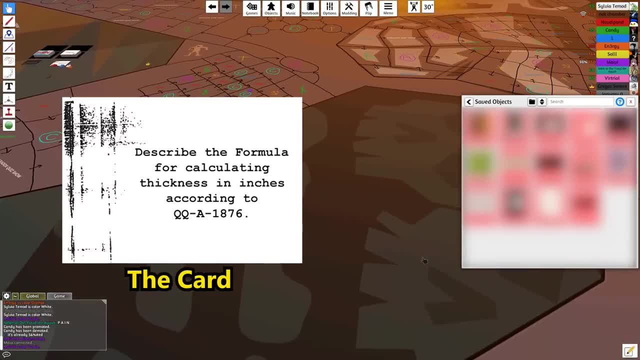 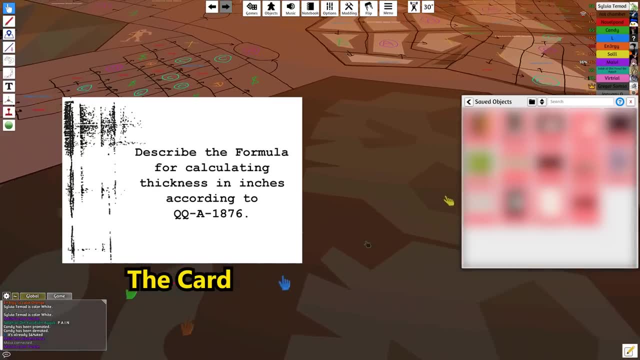 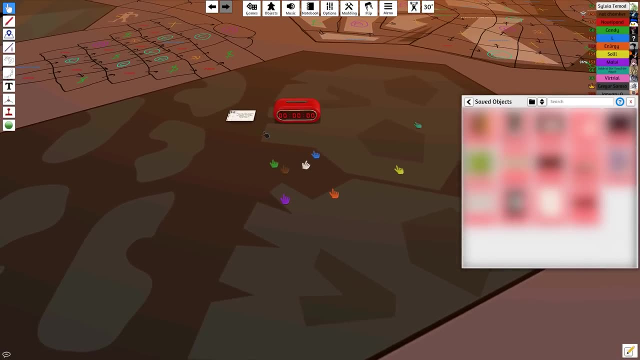 now, i'm not a cruel man and i'm going to actually give you the ability to find the answer for this. we're gonna drag this over here. this, this armpit. here is the redacted card play field. here. i'm not a cruel man. i'm going to give you, uh, 60 seconds on this timer here. uh, to find, 60 seconds to find. 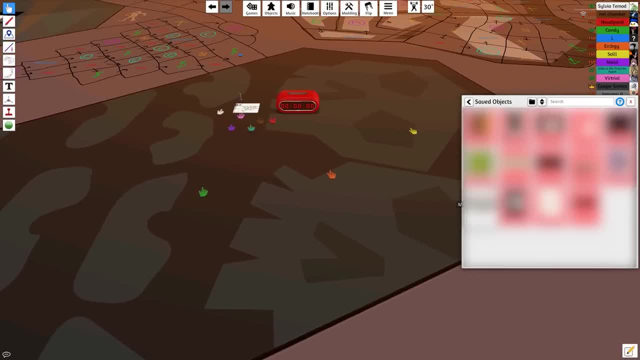 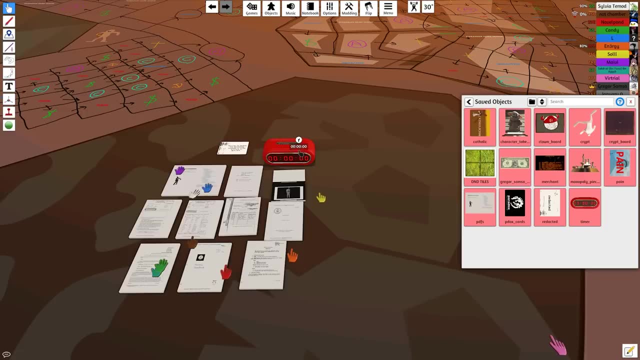 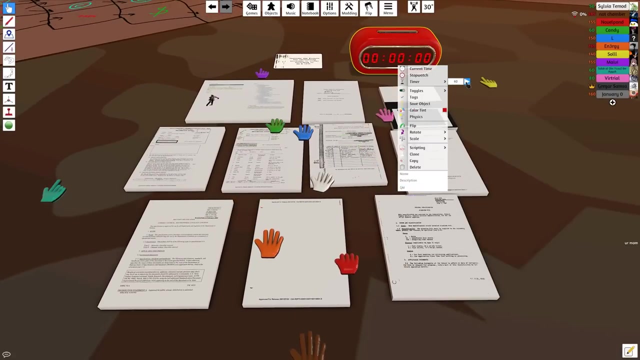 the answer to this question. now and again, i'm going to provide you with the ability to find the answer. the answer is in one of these. one of these redacted cia documents has the answer to your question and you have, uh, 60 seconds to find the answer to your question. go, you have 30 seconds. you have 30 seconds to find the answer. 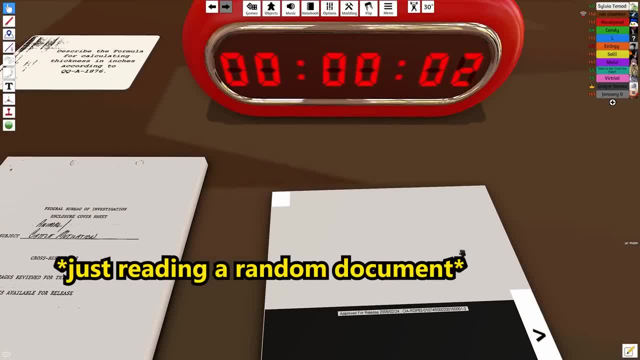 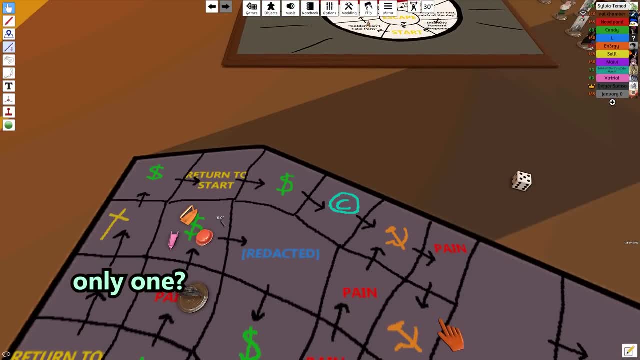 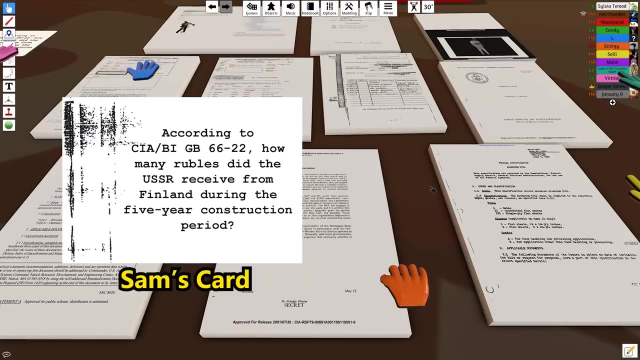 crumbling napoleonic uh, uh empires. oh, i'm so sorry you are out of time. i'm afraid you go back one, only one, pieces, only one. yeah, i know you don't get money. you don't get money. i should clarify. some of these pdfs are like 200 pages long. oh, my god, these are the. 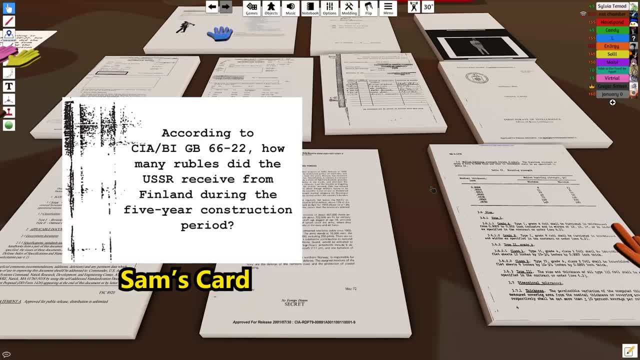 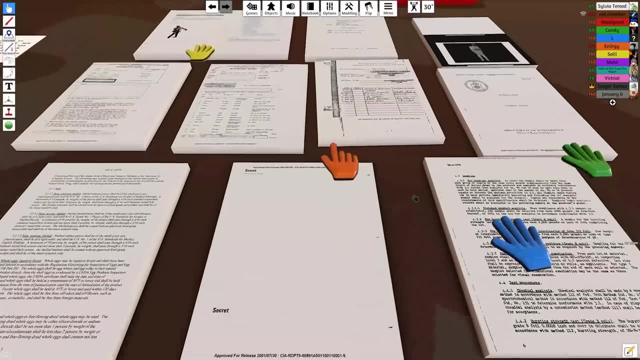 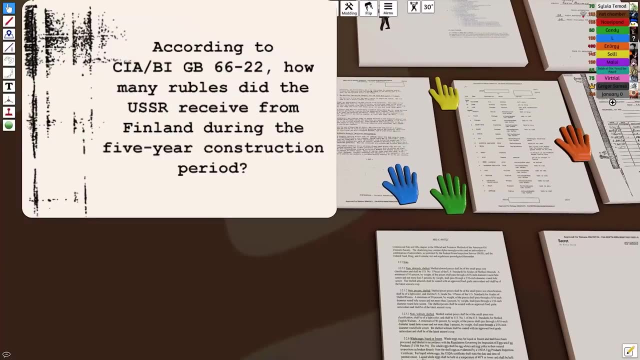 pdfs you guys were talking about the whole time. yeah, god, yeah, yeah, i'm a bit. personally, i'm a big plan, a fan of con plan 8888. yeah, complain, 808 is actually quite great. or the man, as it's known, the scp. i would say, sam, a good start would have been to look for the document titled cia-bigb6622. 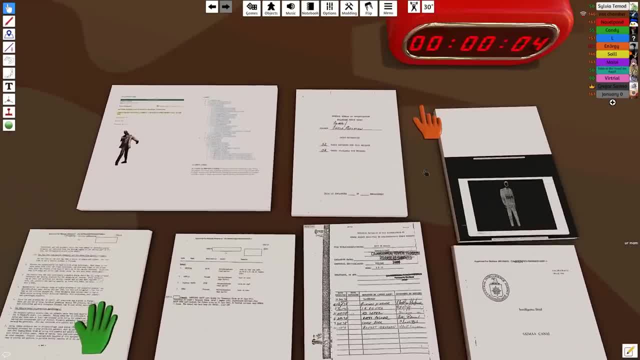 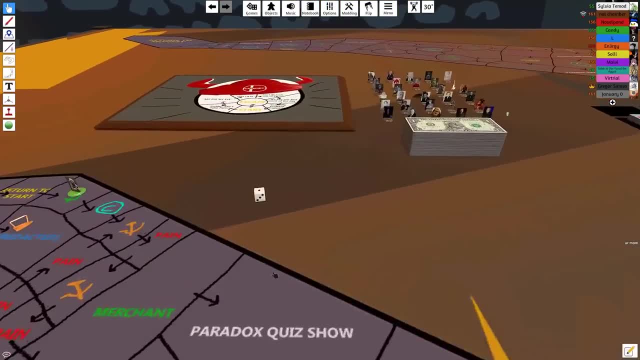 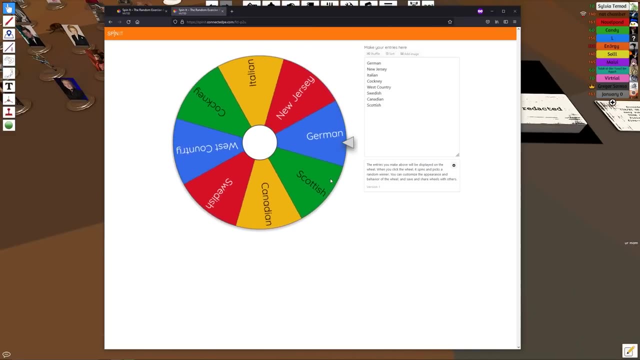 uh, no, no, he's playing on the hardcore difficulty. yeah, you're not allowed to even look at the nightmare. oh, out of time, i'm afraid you go back to space. oh, soul, time for an accent and i have to go back on space. what's saul's accent? oh, please don't land on. oh, it's german. 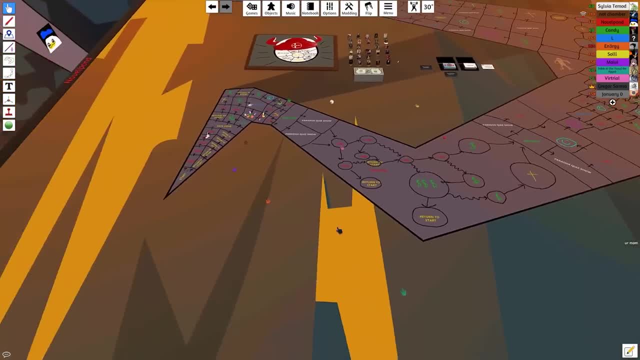 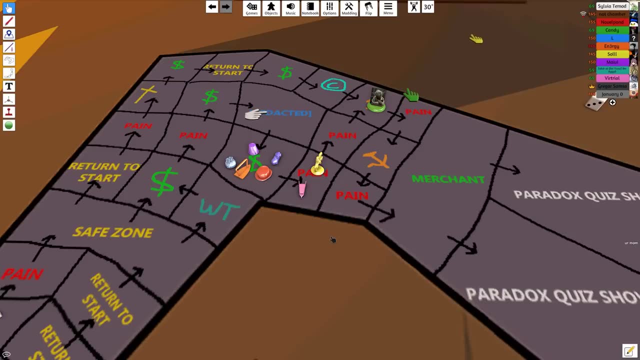 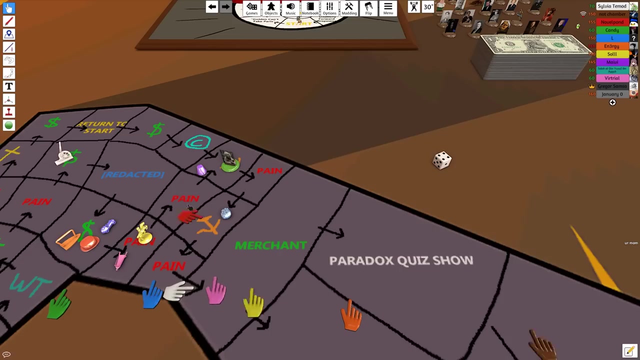 again. this is the worst, the worst. he's the worst. this is absolutely amazing. teddy has like a lab coat and an eye patch and he's making some death ray in a lab somewhere. one, two, three, four, pain, pain, oh god. roll a d20 and move back that many spaces, oh my god. 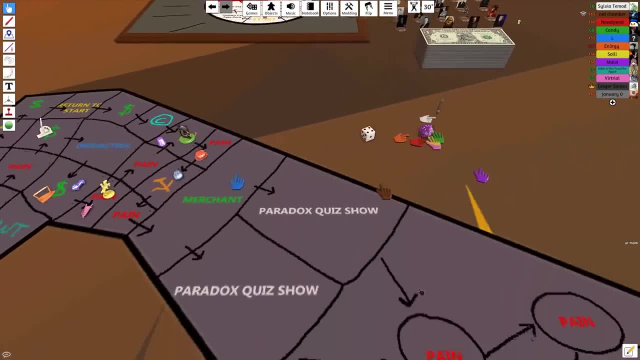 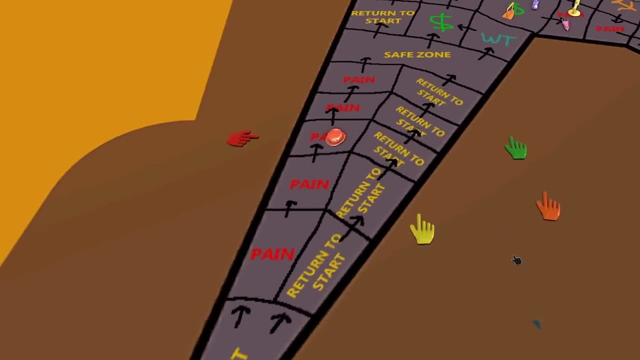 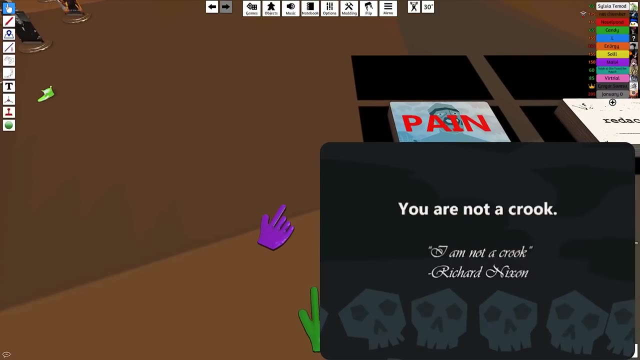 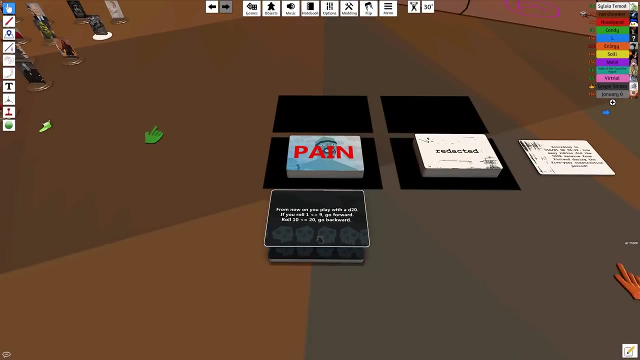 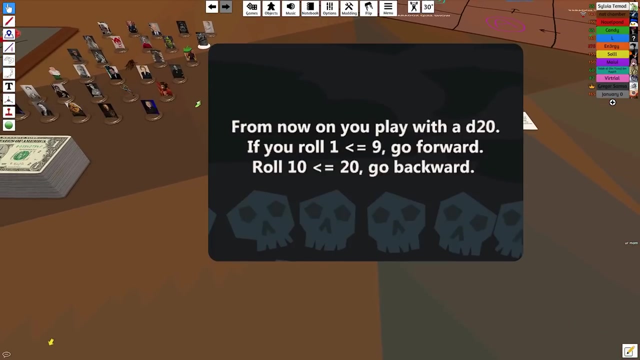 oh no, spain again. richard br走. oh, oh, sam, oh, poor sam. oh yeah, ninth, ninth, From now on, Sam, you roll with a d20, and if you roll a 1 through a 9, you get to go forward. 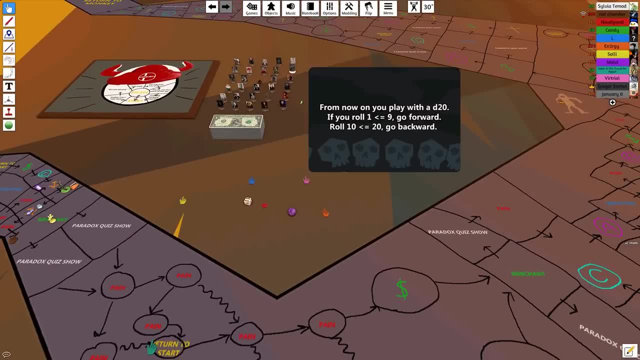 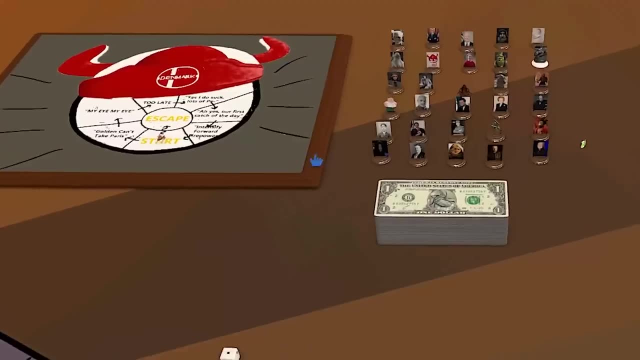 10 to 20,. you go backwards, Oh my god. and then what? And then afterwards you roll with a d6? No, this is permanent. Uh, then maybe go. Ja ein, The fucking German is spreading, I swear. 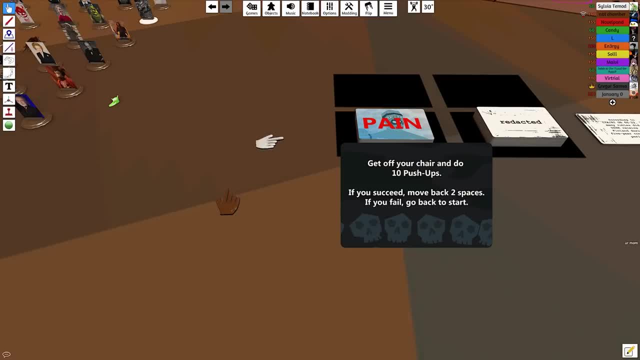 You're all over as well, I cannot even do one push-up. Well, if you fail, you go back to the start. Okay, but how do I prove it though? Uh, we need to hear a real physical effort over the microphone. 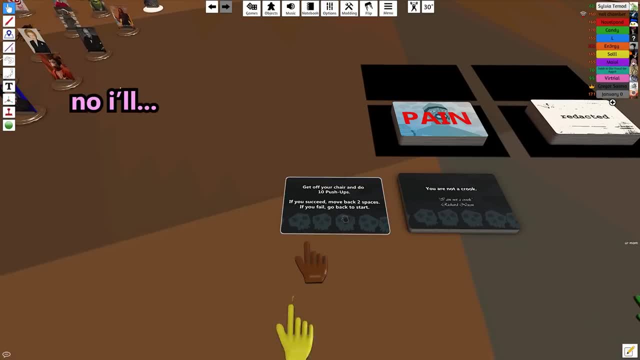 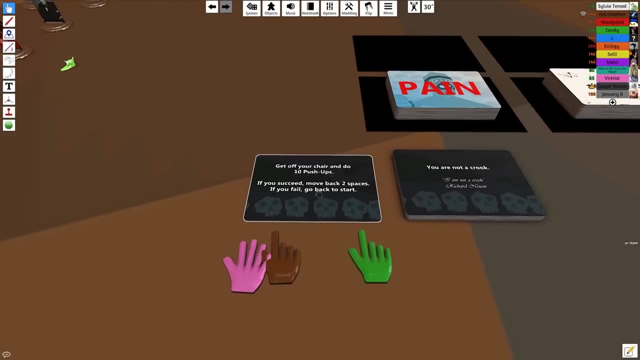 If you'd like, you can skip it. you can skip. you can simply, you can simply fail and go back to start. Do it needs to be continuous, because then I know I'll fail. Yes, I'll try, I guess. 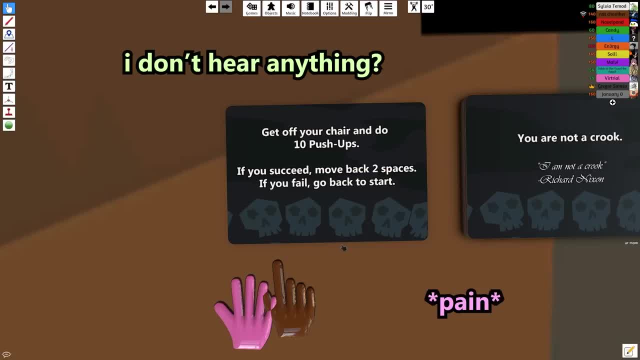 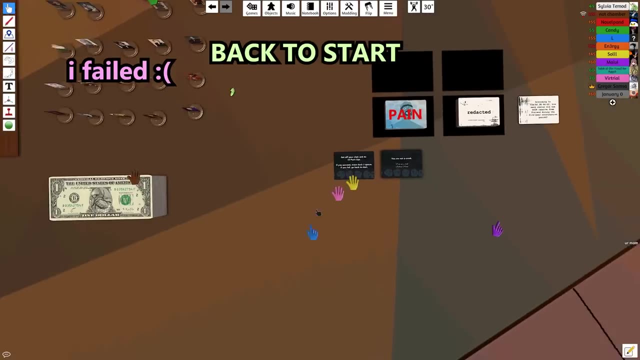 I don't hear anything. There's no. where's the F for it? Two Pitbull, Pitbull, Hi, I failed. Back to start. Back to start. I'm lucky. Good effort maybe, but I'm afraid you failed. 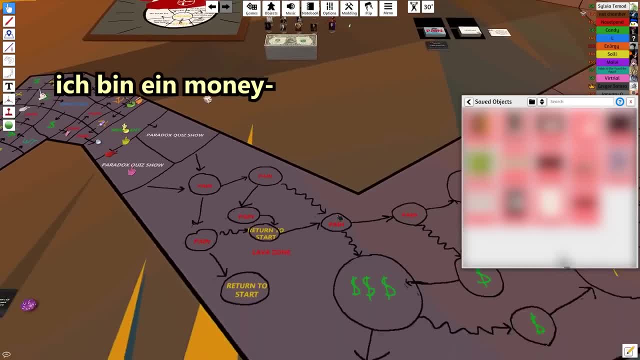 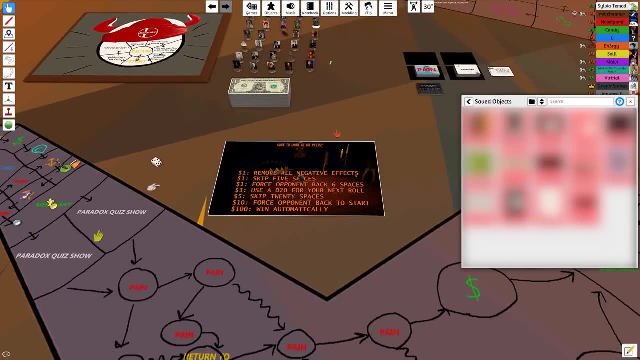 It's fine. It doesn't sound fine to me. I now no shh, shut up. I'm now going to explain how the merchant works. So with your money you can buy these things. Yeah, just press uh Q, press Q and E to see it. 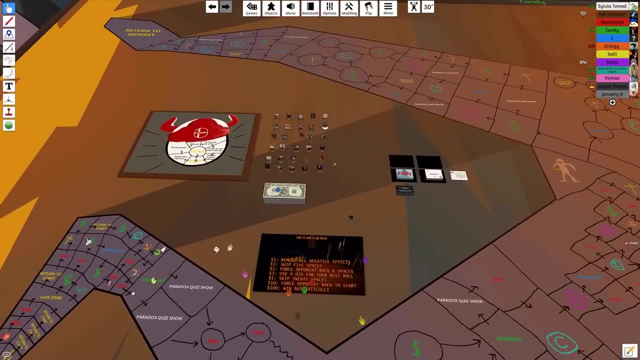 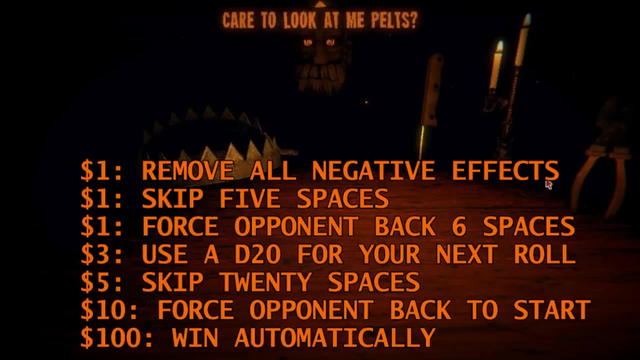 It's inscri- yeah, it's inscription. Yes, it is inscription. Oh my god, I feel pukey now. Oh, I swear, if my board game has actually made someone physically sick, I'll be so happy. Only ten dollars to force somebody to go back to start. 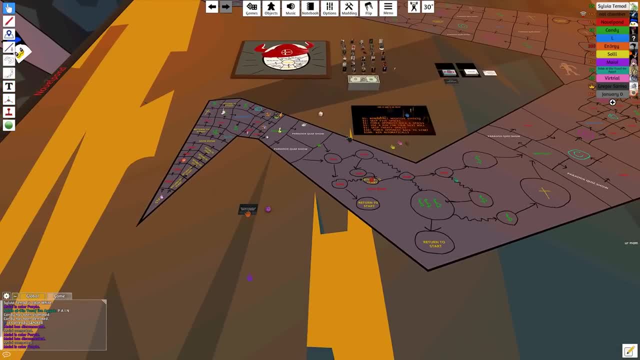 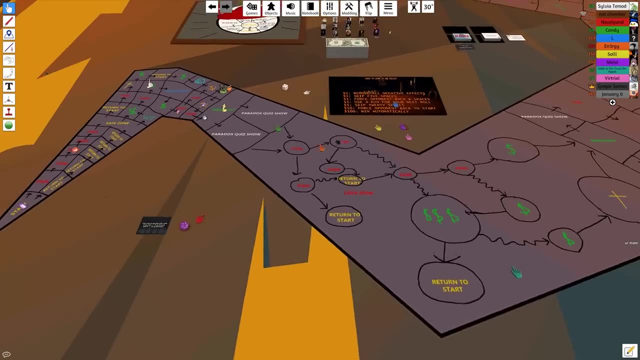 Now, the only other thing I need to make note of is the start actually is also a merchant as well. If you get sent back to start and you have money, you can buy something from the merchant. This could be very useful for someone who say: who say has been doing an accent or character. 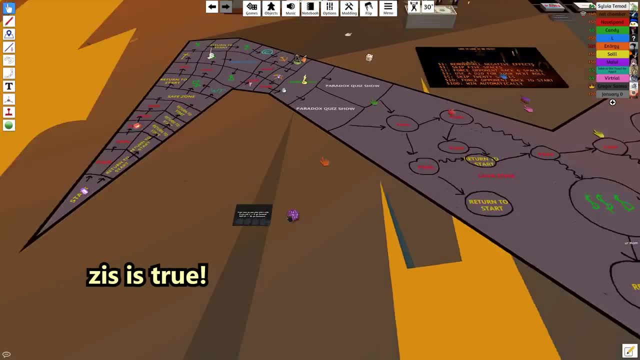 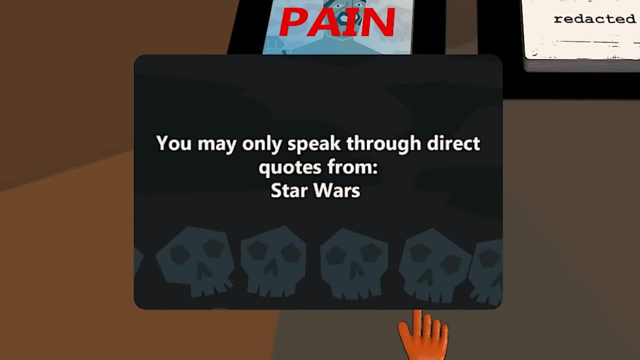 for like an hour and a half and really want to get rid of it. or like Sam, who currently is stuck rolling with a D20.. All right, virtual, now you can roll. Unlucky man, Are you pulling out a fucking like sheet for him to use? 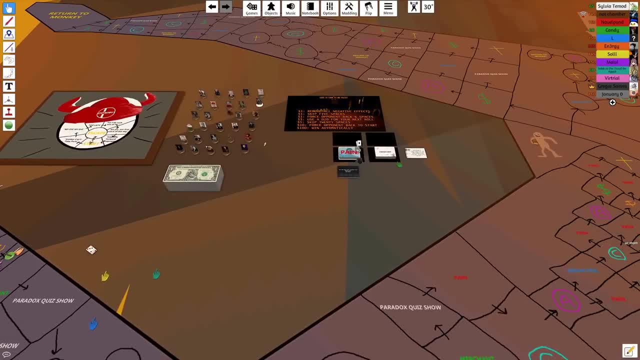 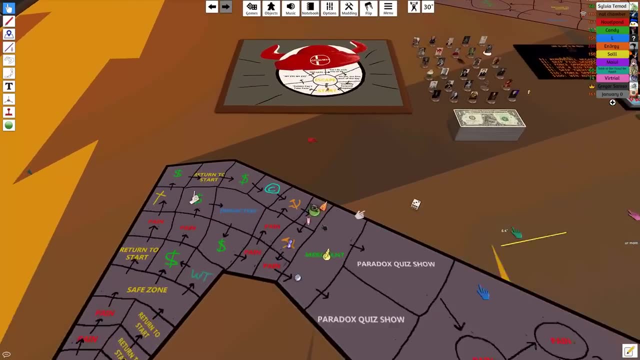 No, no, he needs. he can go to the IMDB page himself and find the course list. I mean he could just say: I have a bad feeling about like throughout the whole game. I have a bad feeling about this. Don't get cocky, kid. 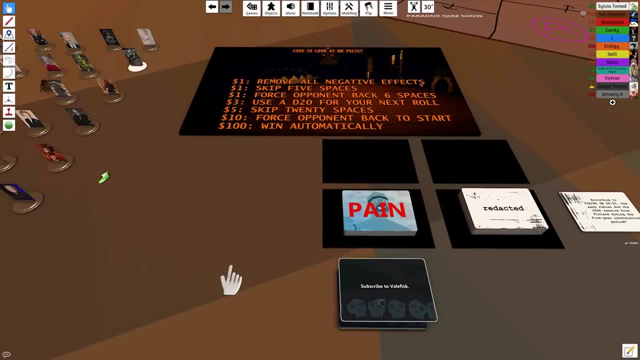 Nice shot, kid One in a million Pain. Oh no, the worst. Oh no. Wait, Vail, if you're already subscribed, do you have to unsubscribe? No, you have to PayPal me $10 directly into my bank account. 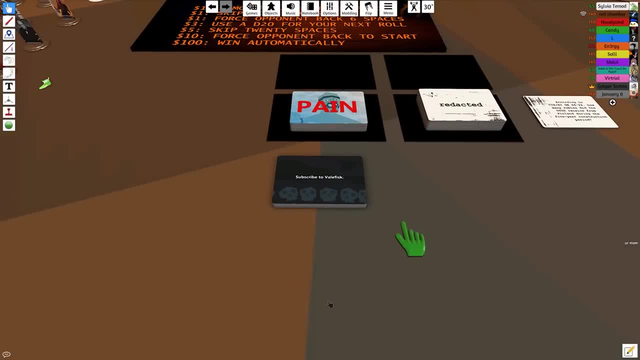 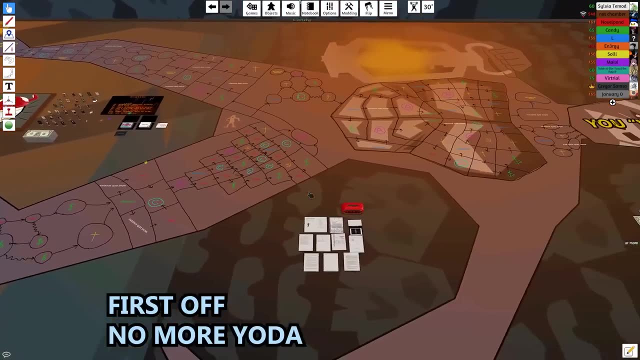 Yoda, Yoda. Is that the merchant? Wait, isn't Candy the one with a shit ton of money. He's $6.. First, stop, No more Yoda. Theoretically All right If I were to, if I were to send Chamber back for six paces. 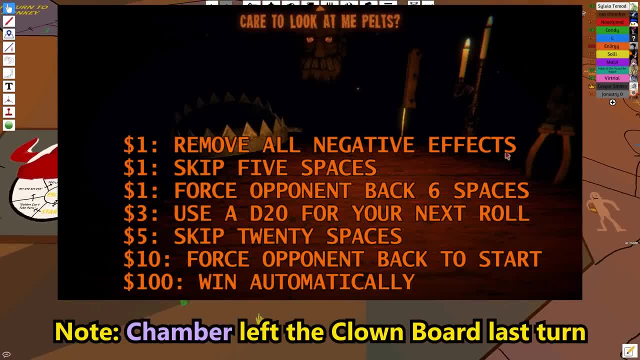 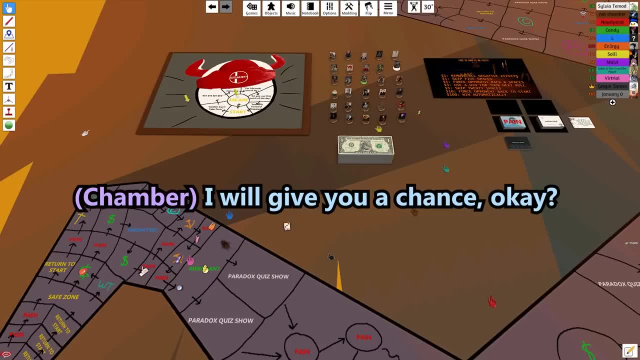 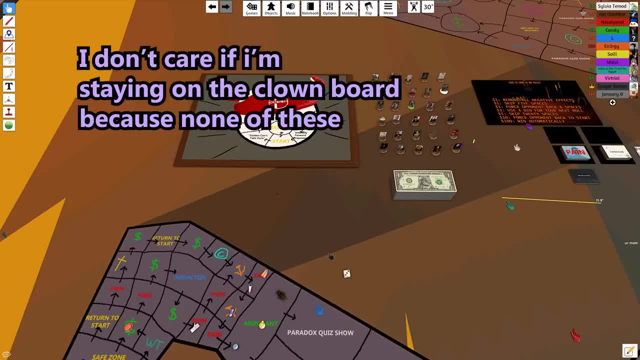 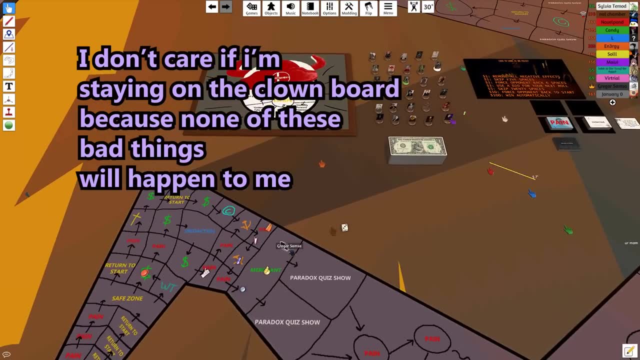 I don't care if I'm staying on the clown board, because nothing, none of these bad things will happen to me. I'll just go, keep going round and round and we'll go in Waste, waste your entire afternoon. Oh, are you going to spend your five Candy? 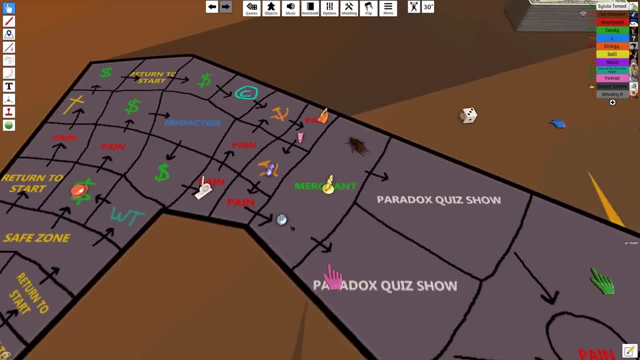 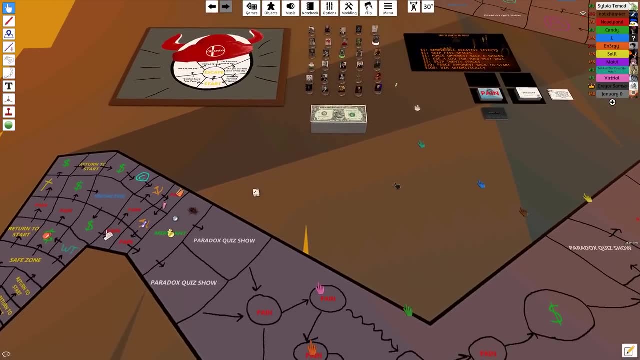 I'm thinking: Think faster Shit. It's a bit difficult for me. I just like to say it's been an hour and no one has actually exited the start yet. You know what? I'll keep my money, All right. 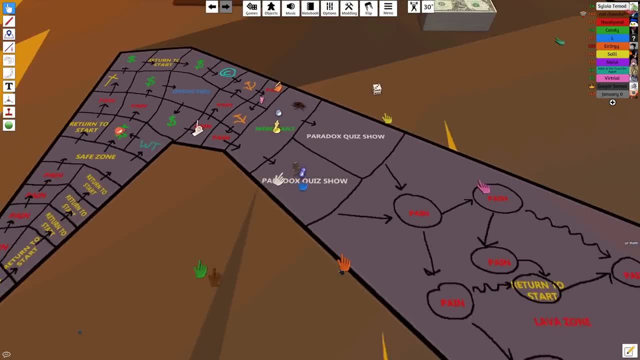 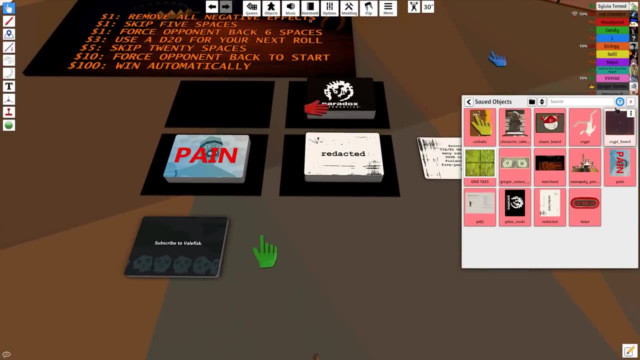 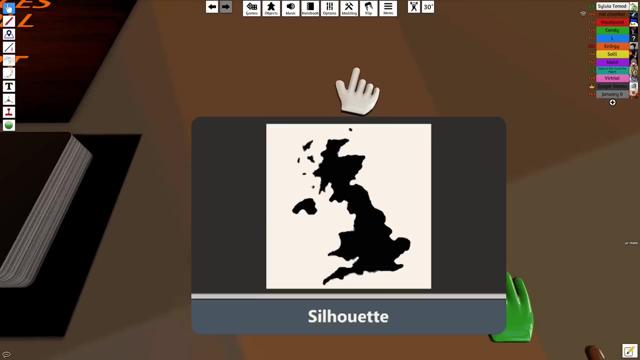 Uh, Patajo. Oh, it's time for the Paradox Quiz Show. oh, it's time for the return of the paradox quiz show. god, it feels so wrong to not be speaking like yoda now. now you have to tell me what silhouette, uh, that is of, and then what game. 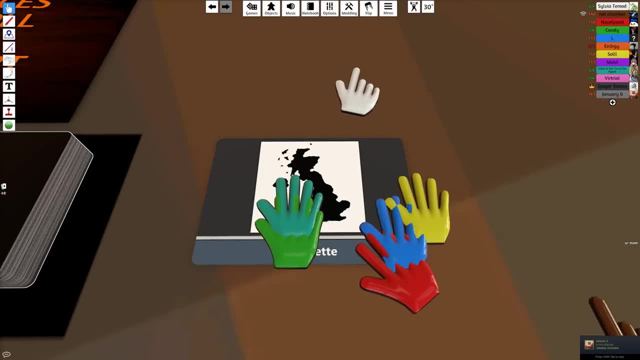 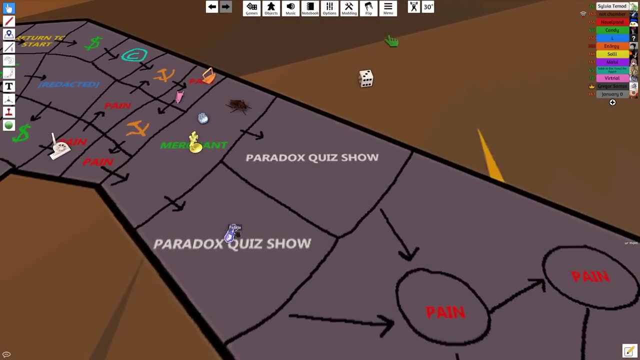 it's from: um, that's the united kingdom from, uh, hearts of iron four. no, i'm sorry, that is the united kingdom from hearts of iron one. i'm afraid you'll go back a space unfortunate, and you don't get to use the merchant either. it's just like old times. it's just like old times, it really is just. 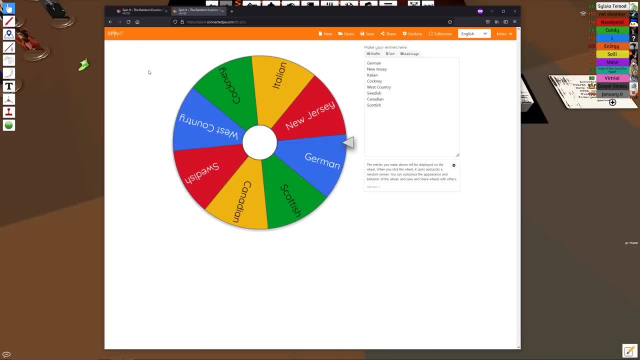 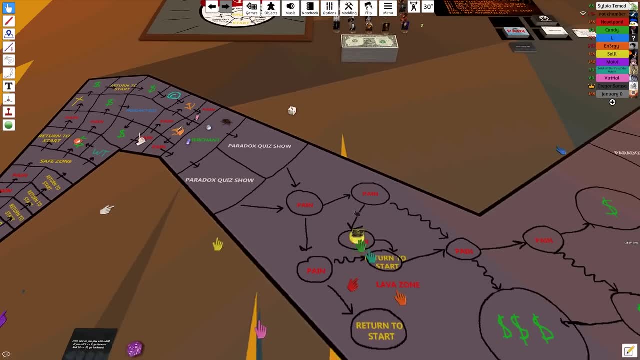 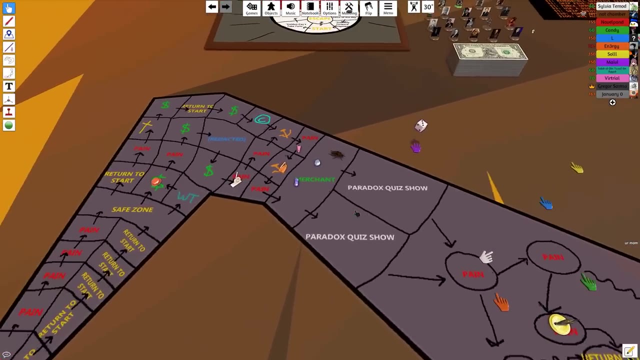 like it's beautiful. oh, you're no longer german soul, you are something worse. oh no, all right. it landed on shrek. it landed on um. all right, all right, what are you doing, amy swamp? oh my god, uh, baby, it's baby's turn. are you alive still, or you did you, did you die? 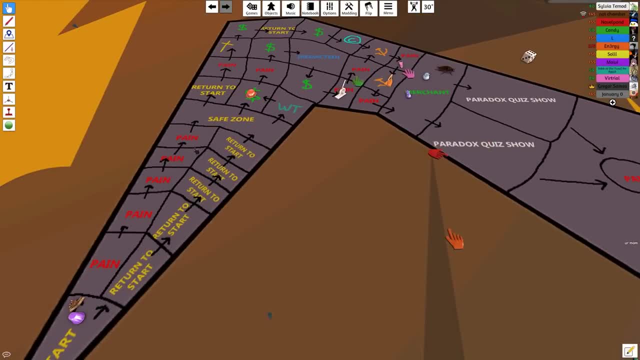 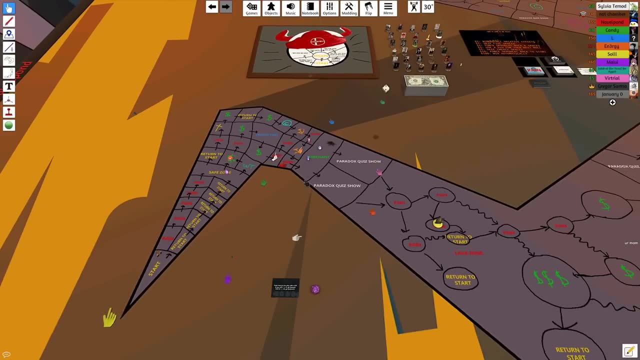 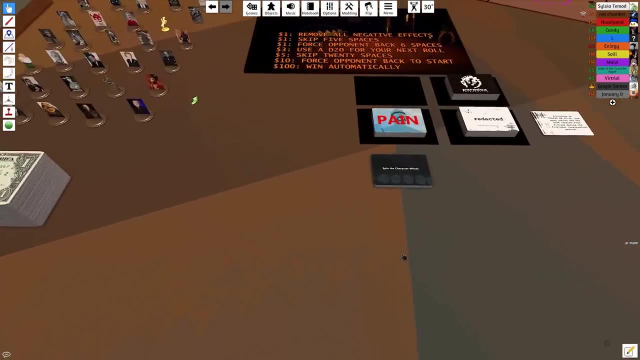 now you're alive. i took a painkiller. okay, don't worry, you get to go to the safe zone now. yes, oh my god, you're the. you're the. wait a second. you're taking a painkiller, but hold on. is that a performing enhancing drug? oh, those aren't. those aren't banned, those aren't banned. oh, teddy, you were a loved one. 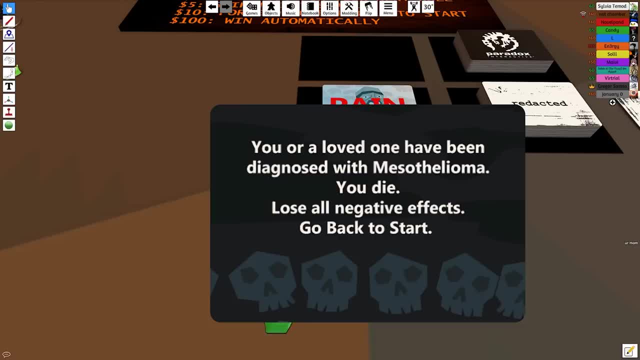 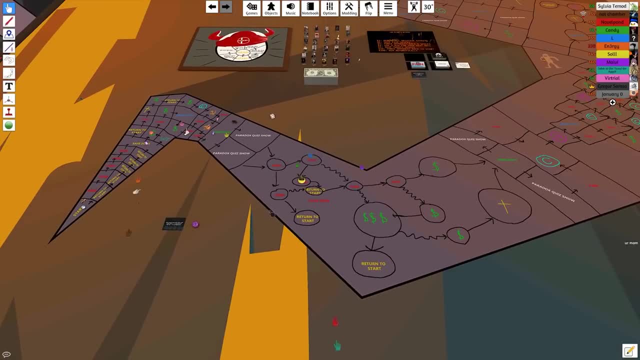 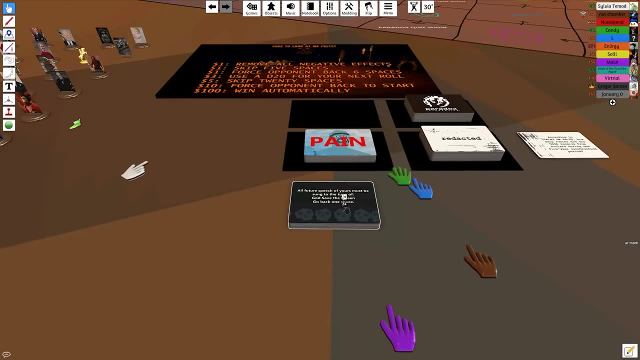 have been diagnosed with mesothelioma. you die, lose all negative effects and go back to start. no, i don't get it anymore. you may not. you were literally in first place as well. all future speech of yours must be sung to the tune of god: save the queen, go back one space. 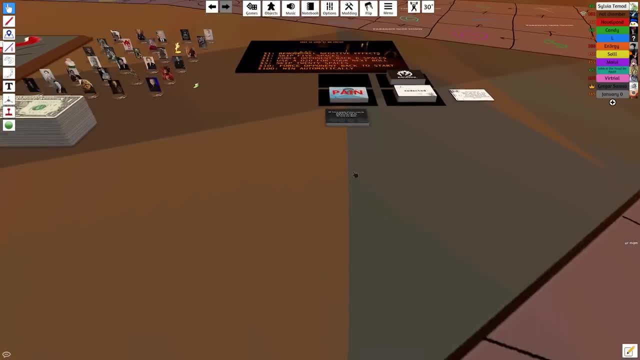 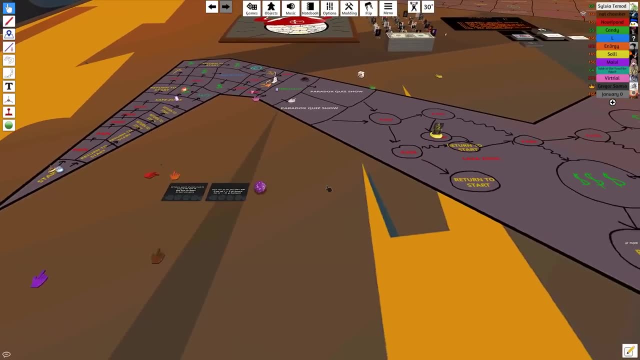 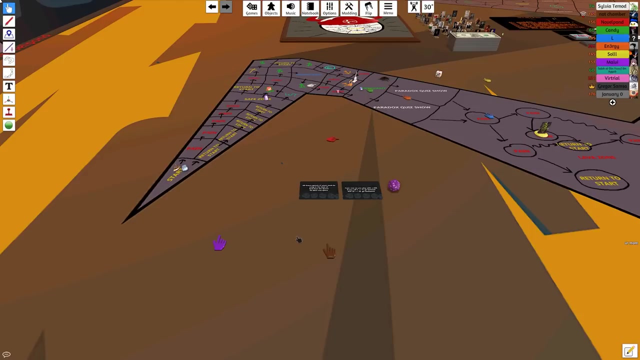 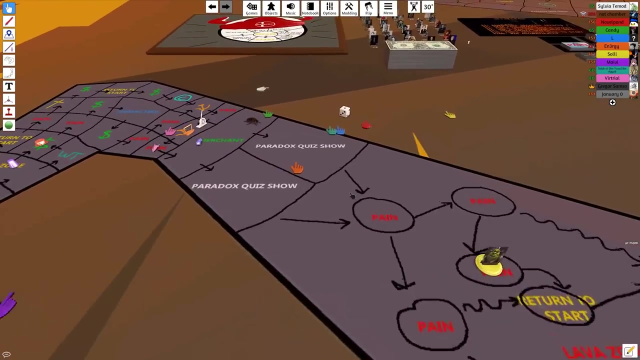 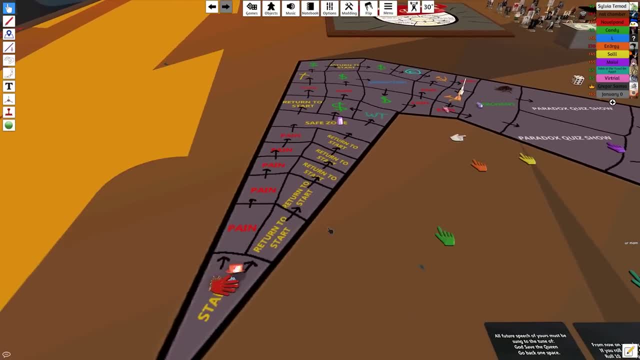 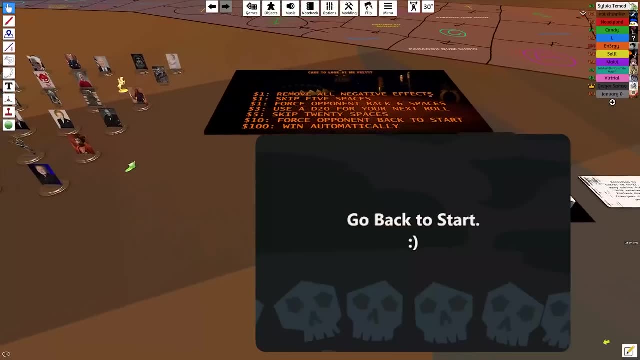 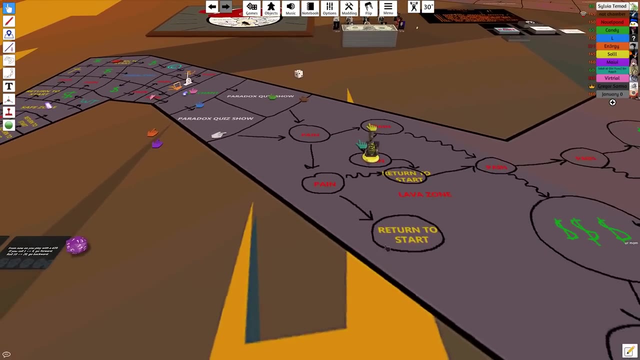 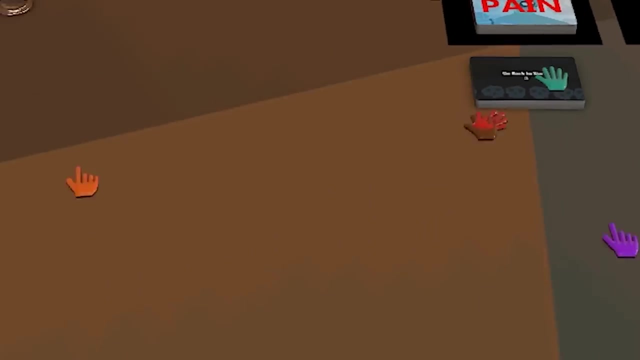 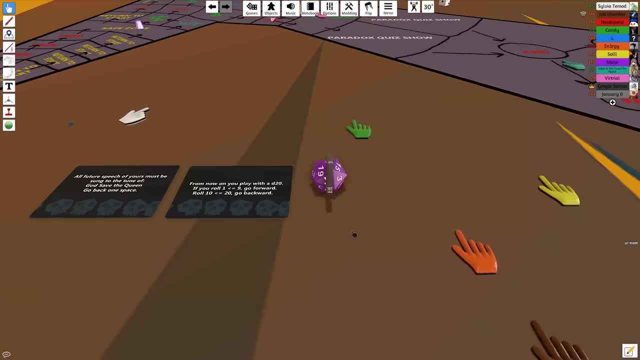 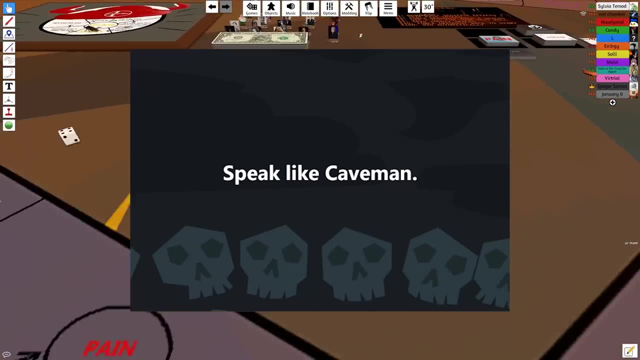 all right, let's go with the pain. another one doesn't matter. back we go, it's rigged, back we go. a blessing and a curse. a curse, what was that? four, four, four, good job. one, two, three, four. you're on this pain. you now have to speak like a caveman. um, yeah, like that, that's perfect. yeah, we haven't even landed on the other. 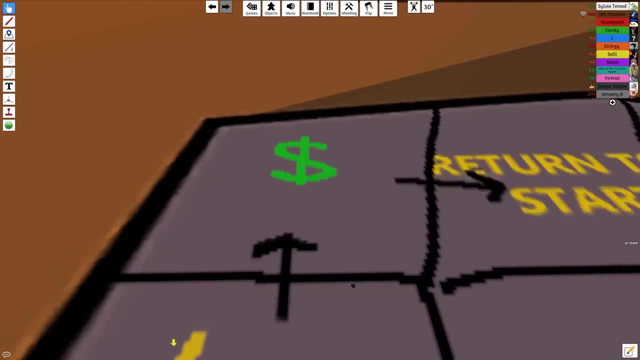 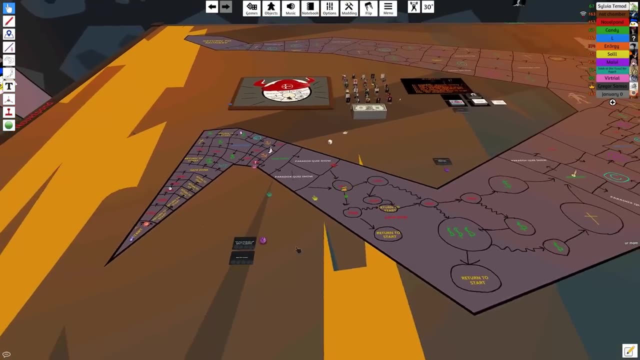 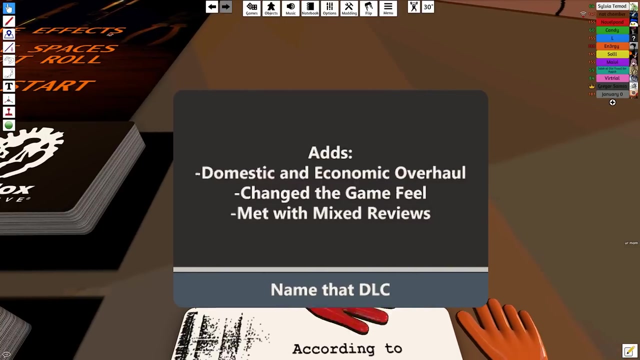 there's still a full card deck missing. why is it the christian one? i'm not sure. yeah, no one's landed on christ. actually, i think he went no, no, never mind. oh, paradox quiz show. you get to do the paradox. oh, name that. dlc. a classic category, this one adds a domestic and economic overhaul. it. changed the game's feel and it was met with mixed reviews: wealth of nations, wealth of nations. so he has answered: wealth of nations for eu4. let me just uh quickly check here now. i'm afraid. uh, this was actually the new deal brought in by fdr to the united states. excuse me wrong dlc, sorry how much. 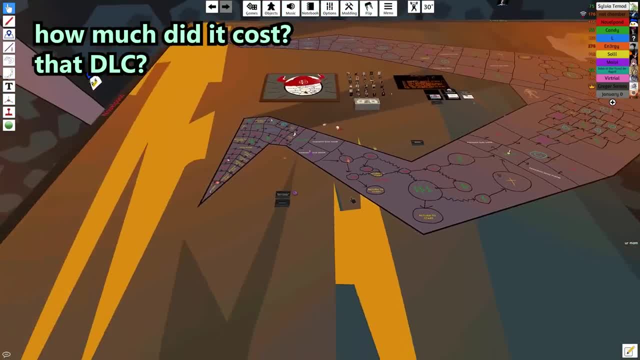 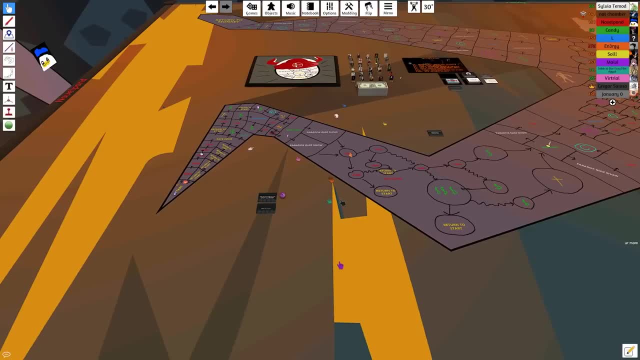 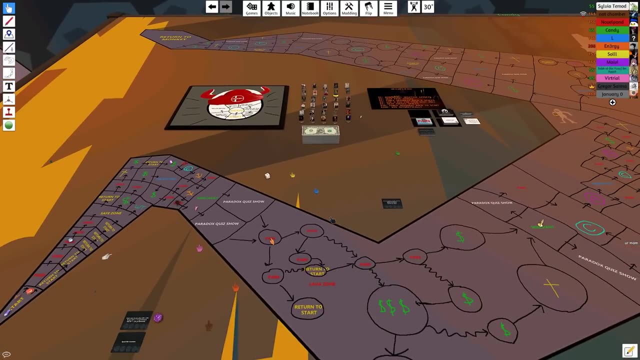 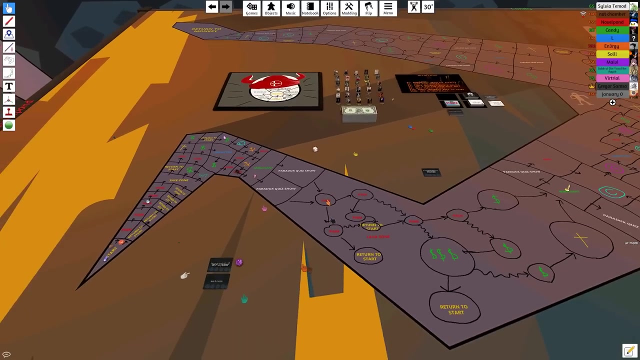 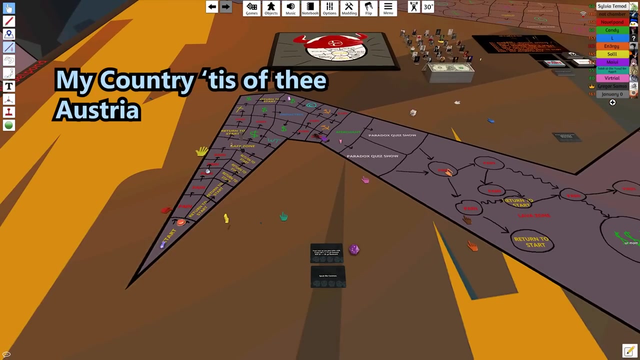 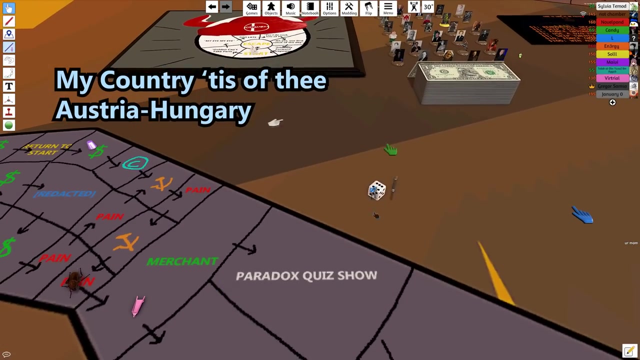 did it cost that dlc? uh, some billions. just a quick question from me: what if i only say one word, to say it starts to be the two to the tune has to be like one of the notes, i guess. okay, my country, and then we don't have the rest. nobody did the rest of it. i forgot he's using the 20. that only. 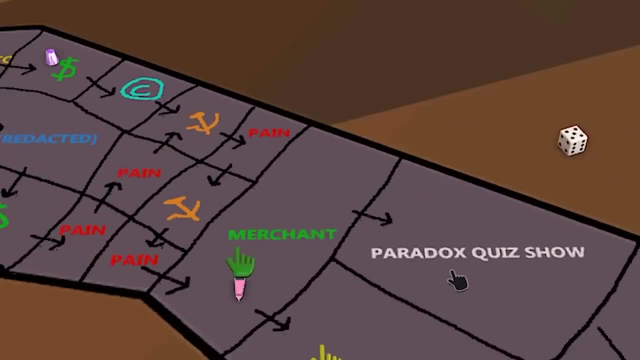 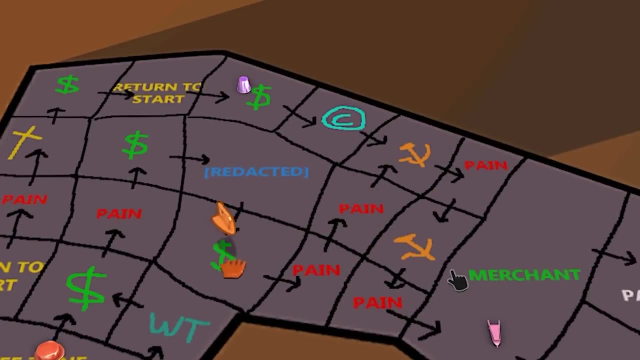 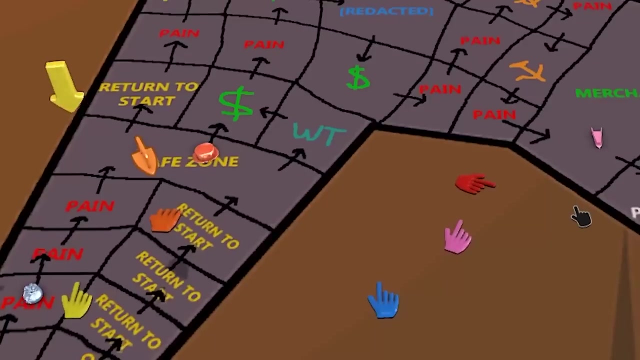 is the caveman. oh, you have to move back 17 squares. start moving, then 17.. i want to watch all of it. one, two, three, four, five, six, seven, eight, nine. i think that would straight up put him back at this. no, no, you're gonna go that way. eleven, twelve, thirteen, fourteen, yeah, fifteen, sixteen, seventeen. 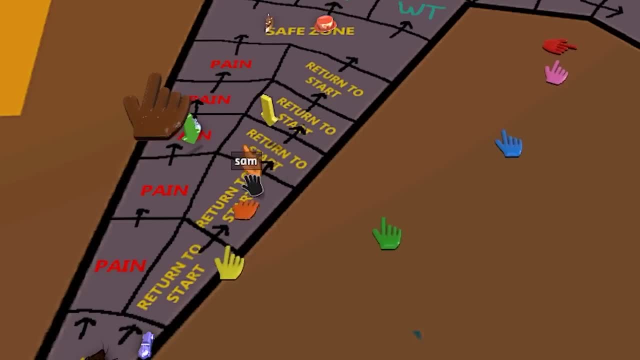 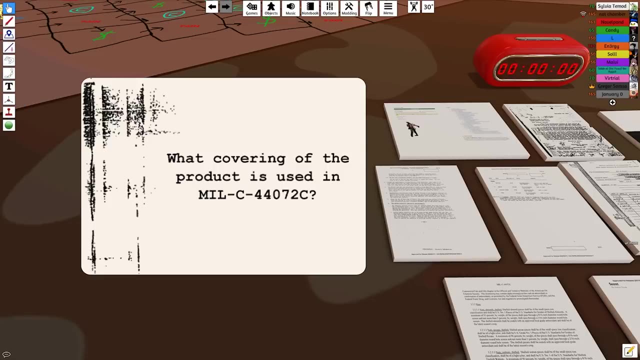 there- i think it's one of them- and then return to start or be on the pain, it's your choice. there you go. uh, you're gonna have 60 seconds to find the answer to what covering of the product is used in mill dash c, dash seven four four oh. seven two c. and to clarify mill dash seven, dash four four oh. 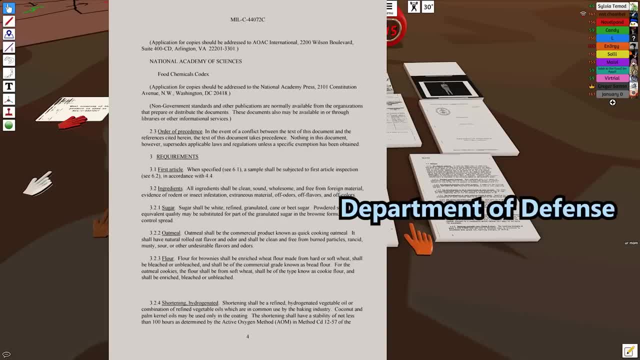 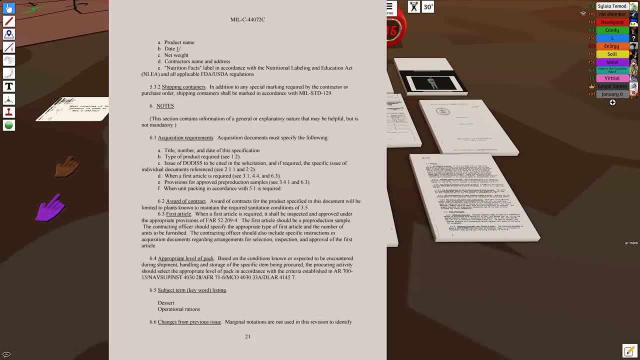 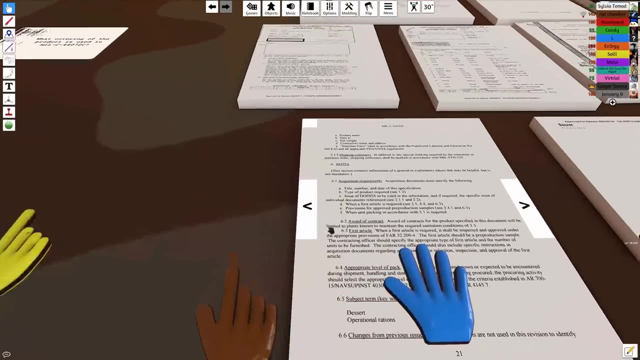 seven two c is the military manual for the cooking of brownies, defense, department of defense. sorry, the department of defense. manual for cooking brownies. has anyone actually that itch to do this in the test game? yes, yeah, i'm so sorry, phil. if you go back to the, if you go back to the first. 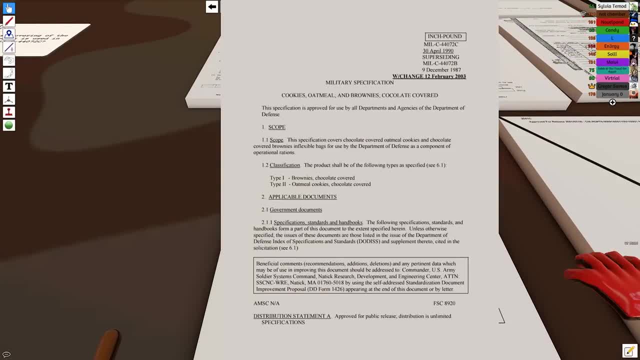 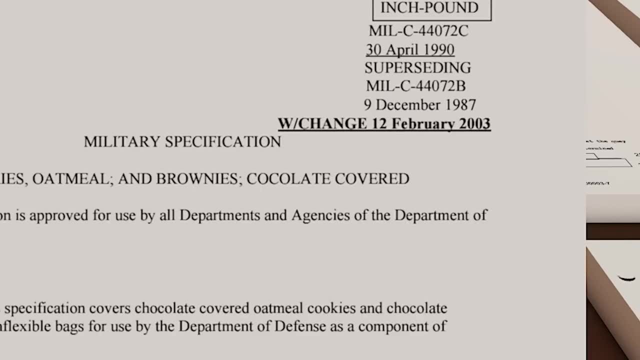 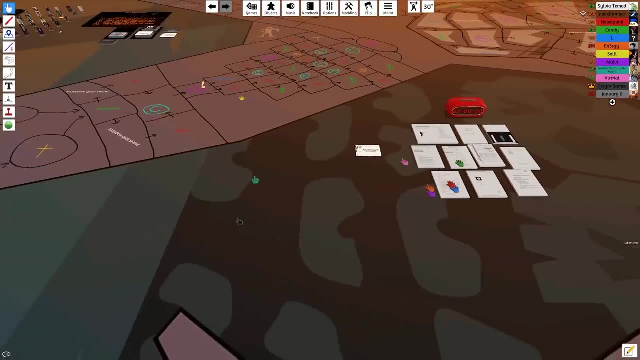 page of this article, you will see uh. it says at the top there: this is a coccolate covered brownie. oh yes, so it's uh. the answer would be: i don't know, the department of defense doesn't hire people who can spell, i guess. oh well, i guess i go back once, that's you know, it's legitimate. 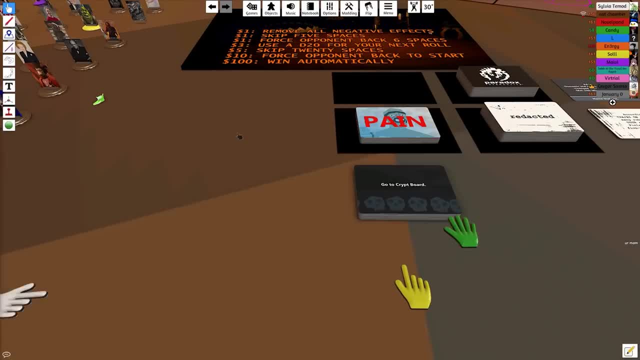 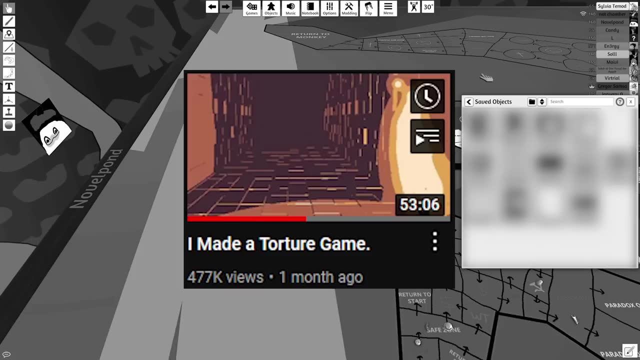 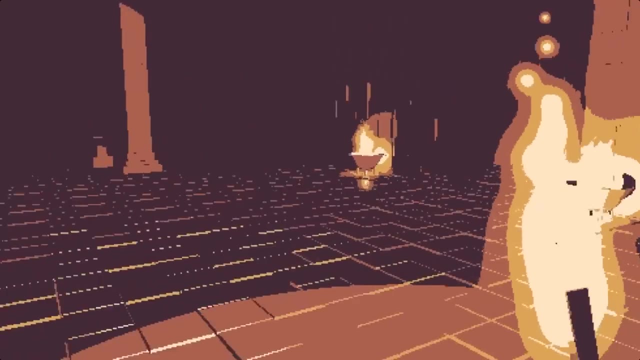 oh, it's time. it's time to run. bring in clown board number two. i should clarify, for anyone who hasn't seen the crypt video, that the last torture video i made was a lot like this one, except instead of a board game i made a full video game. it was a horror game entirely designed just to gaslight and annoy the player, as you can. 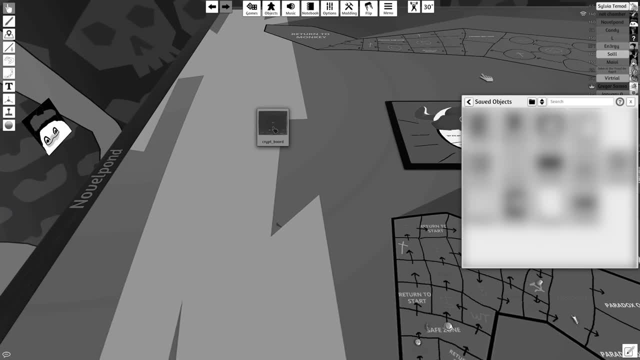 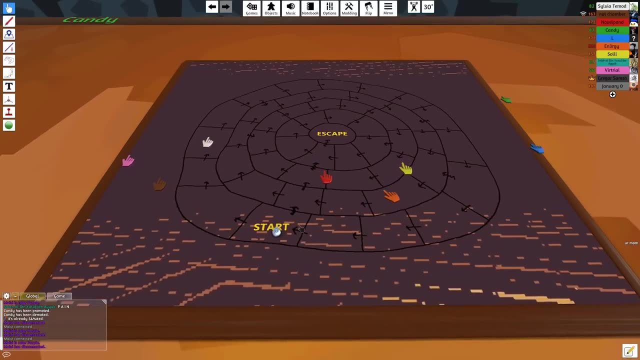 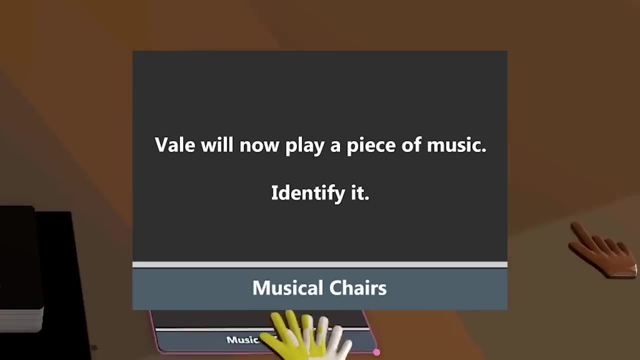 guess it was called crypt and this extra board is based on that. the crypt board has some, uh, interesting rules that will only be revealed. teddy knows what they are because he has spent. he has suffered in the past. but, uh, for, everyone else will find out what the crypt board does once teddy gets to the inner ring. oh, it's time to play. 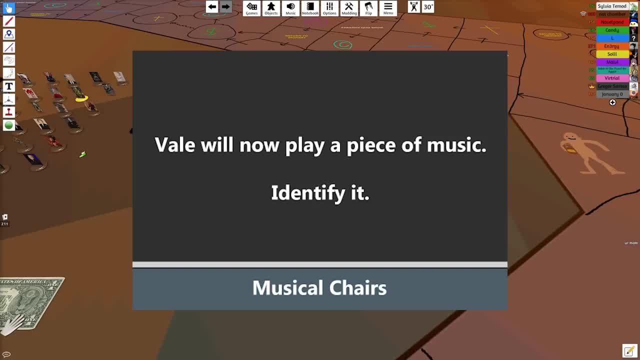 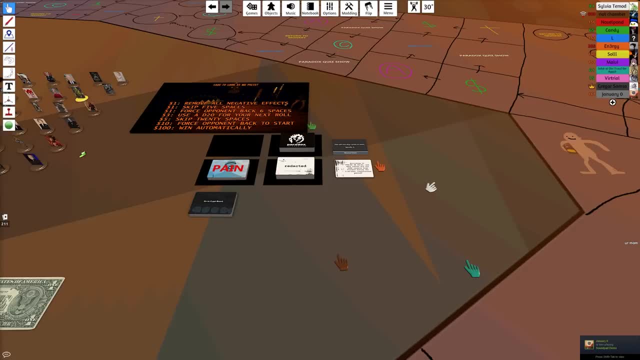 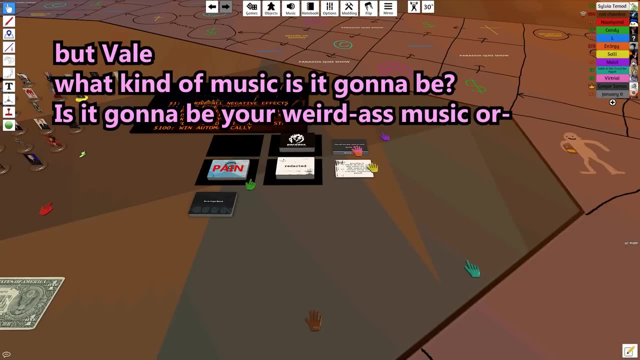 musical chairs. now, i could do this correctly, uh, but instead i'm going to play it through my phone, through my microphone, because i think it's funny, it is humorous. stop, no, mute them right now. mute them right now. what kind of music is it gonna be? is it you're weird as music or it's the paradox? 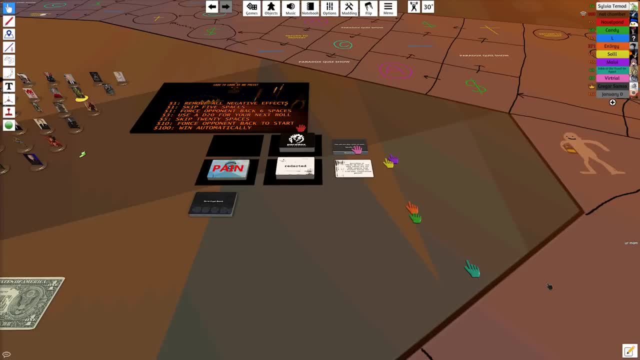 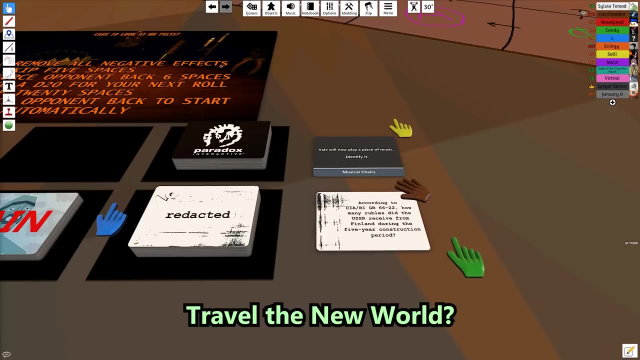 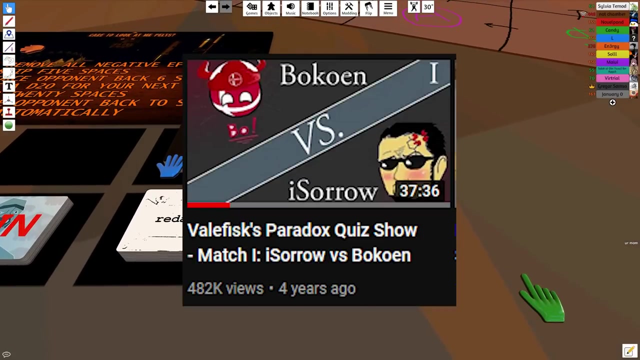 quiz show. so it'll be from a paradox game. oh, i see, i don't. i know this one. oh, i know this one very well: travel the new world. okay, you are just making the. i'm afraid not. that was, uh, the song kings in the north, which is from veilfisk's paradox quiz show, episode one. oh yeah. 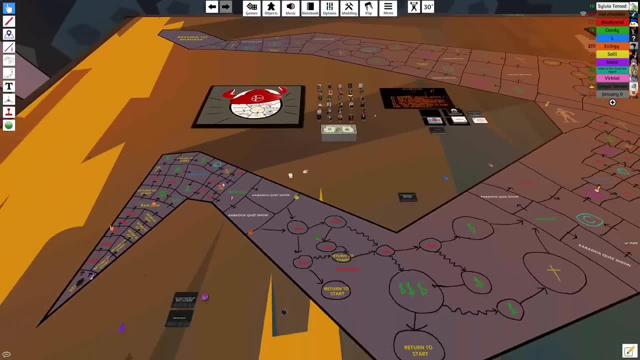 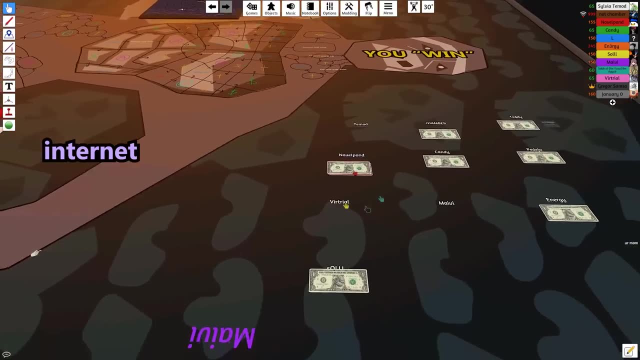 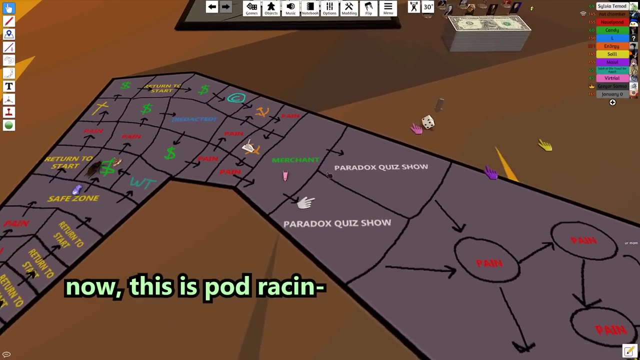 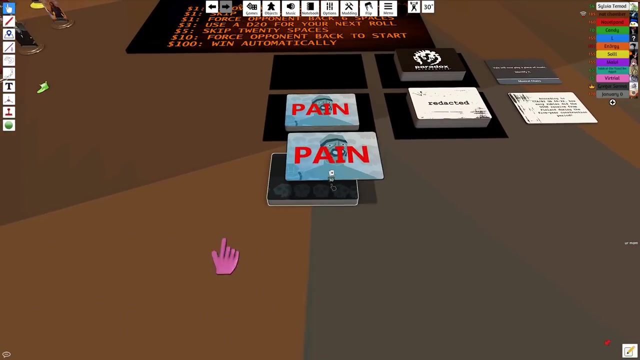 who were the contestants? uh, bo cohen and isp. i was there. oh, that was a great episode. i was there. a turn that trouble. hold on, hold. on. now this is pottery. oh, i forgot. he's been talking in star wars quotes the entire game pain. oh yeah, i'd completely forgotten about that, unfortunate. uh, worst thing is to get an accent. 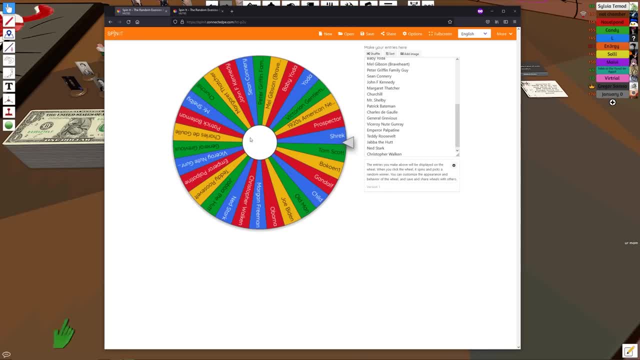 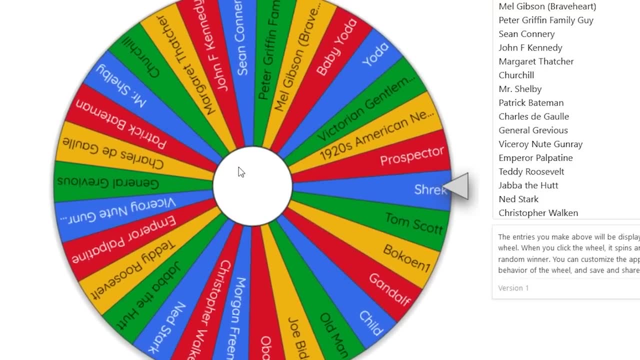 and then get even worse. now you have to do star wars quotes while in character. oh god, i hope you get yoda. yoda, it's gonna. later it landed on shrek again. you have to do star wars quotes in shrek. there's a quite a few star wars quotes in shrek. there's a quite a few star wars quotes in shrek. 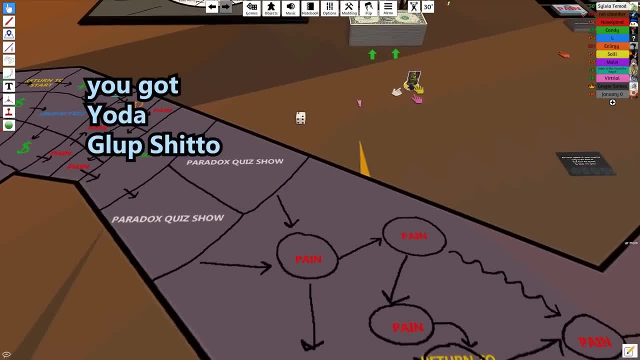 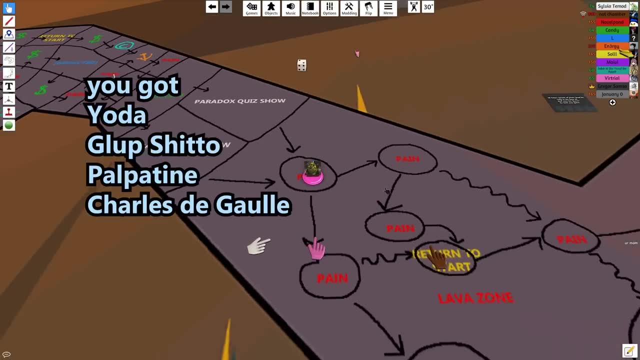 characters. yeah, like shrek, he's from star wars. you got yoda glop, shadow palpatine. charles de gaulle, famous. uh, yeah, he was in the rebels. yeah, he was in the resistance with general solo. who's this? that's christopher walken. oh, christopher walken. 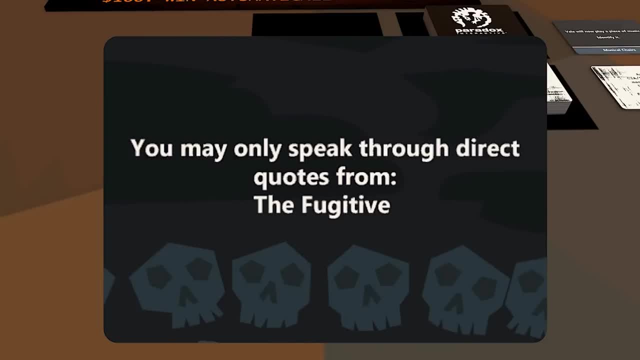 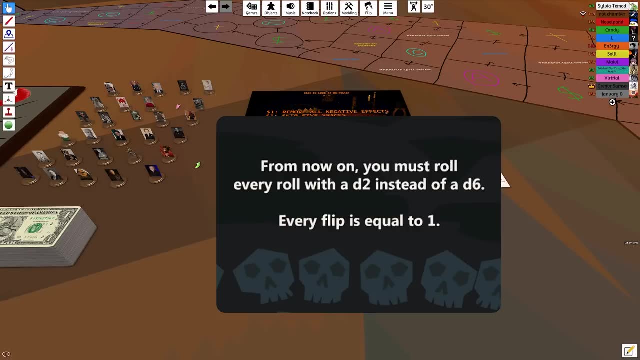 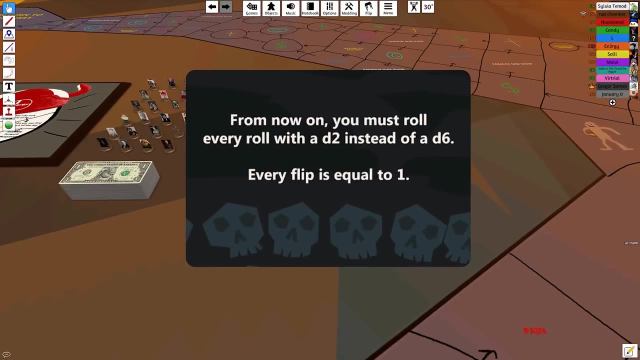 oh, very unfortunate team want to get such an obscure little movie. is the fugitive? i'm loosely. it's my favorite harrison ford film. what do you mean? i'm so sorry, candy, you will now be rolling with a coin from this moment forward. what if it lands on? 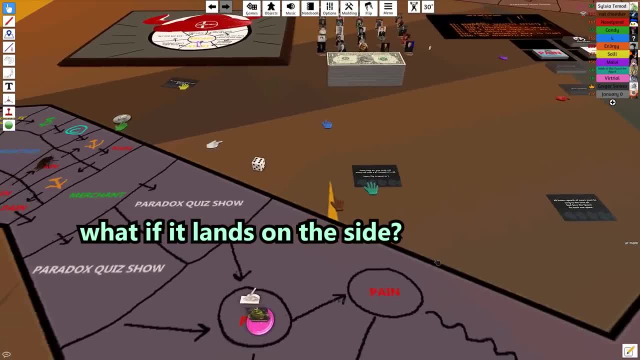 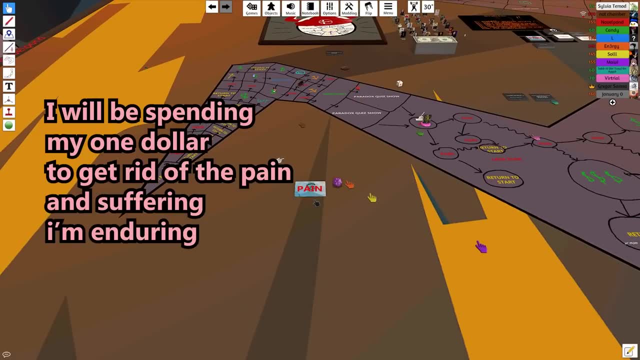 the side, also one it says every flip is equal to one. so no matter what he does, he only moves one- my one dollar. to get rid of the pain and suffering you know you no longer have to use uh the d20 either. good for you. i can't wait for the uh. 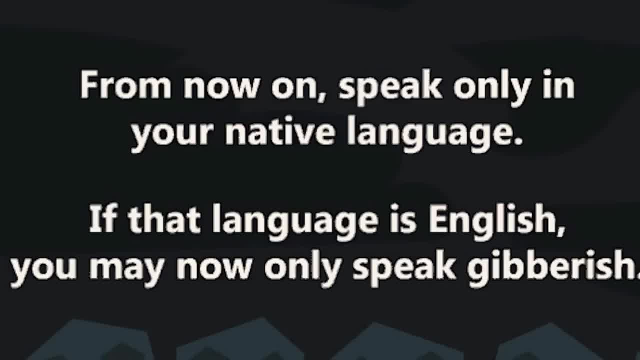 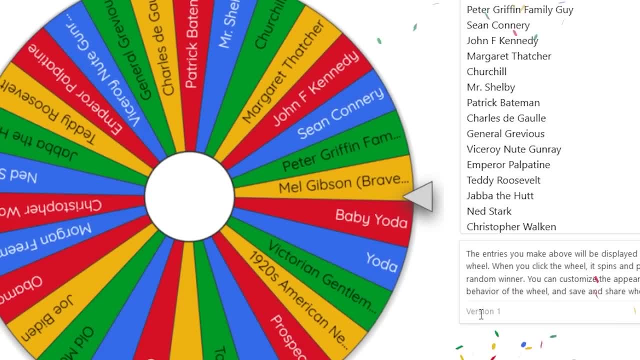 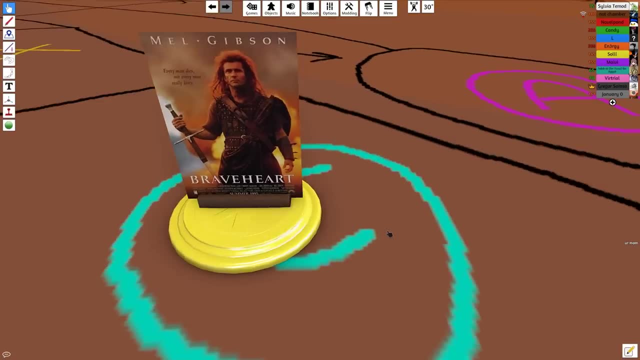 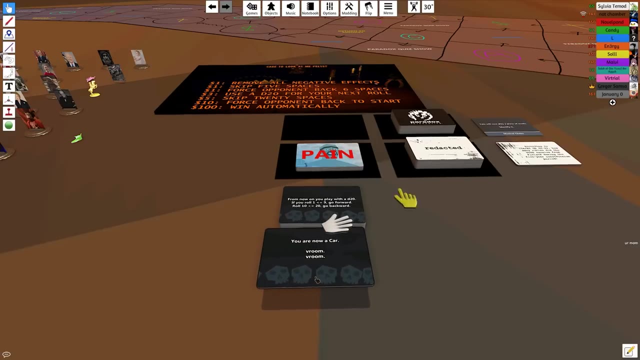 but now back back to uh cave and speak you go. i guess solos just rolled. uh, mel gibson from braveheart, you just have to do a bad scottish accent. just a wee bit of scotch, i know. yeah, oh, unfortunate. so now, in addition to only speaking in star wars quotes while shrek, you need to end every sentence. 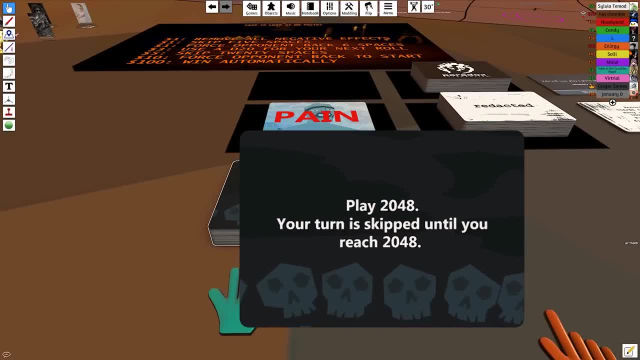 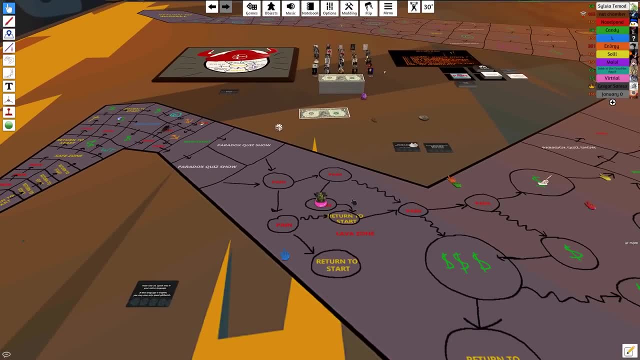 with a car noise. play 24- 8. your turn is skipped until you reach 20- 48.. yeah, that's right, richard, i don't care. oh yeah, playing this in the steam web app thing, it's uh, boosters, it's novel's turn. 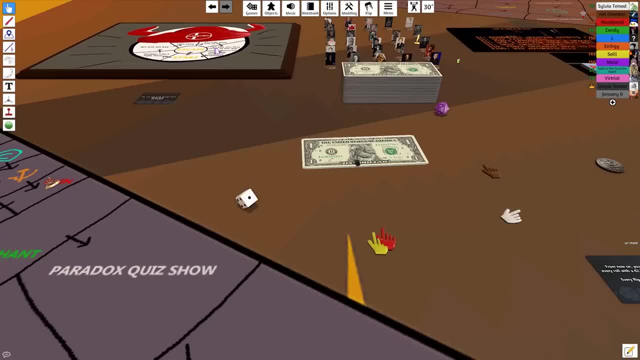 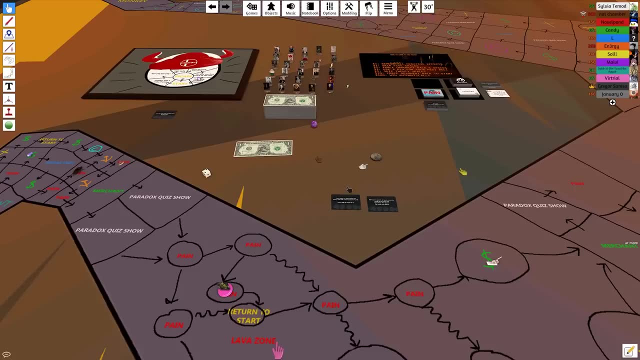 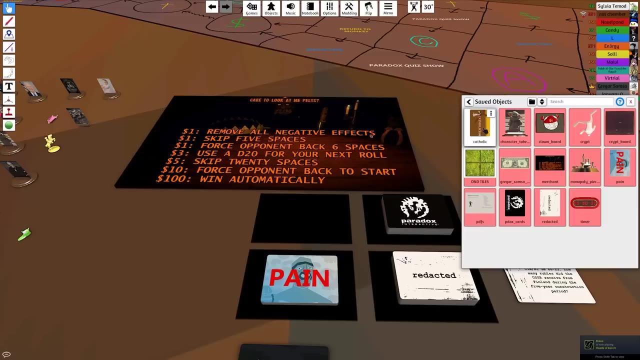 novel. roll the dice. no, we've got him rolling. we have one guy speaking in the fugitive, we have another guy singing god save the queen, we have somebody else- our skins, and then that thing- whatever that is soul- has landed on the last cards, because, of course, this is a christian board game. um, so it's time to introduce the last. 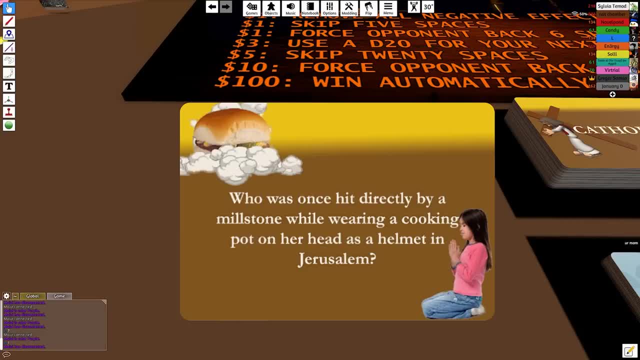 set of cards, uh, the catholicism cards. now i have to say, this is all. this is easily the most obscure question on the whole thing, but we did do this yesterday and i don't think i told you the answer. yes, we did yesterday, did not? you did not tell me the rest. i think i did this yesterday and he did. 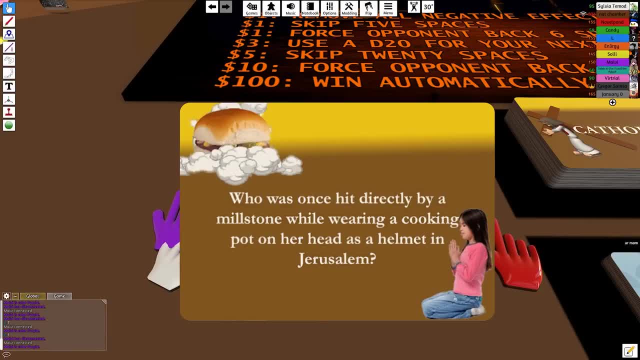 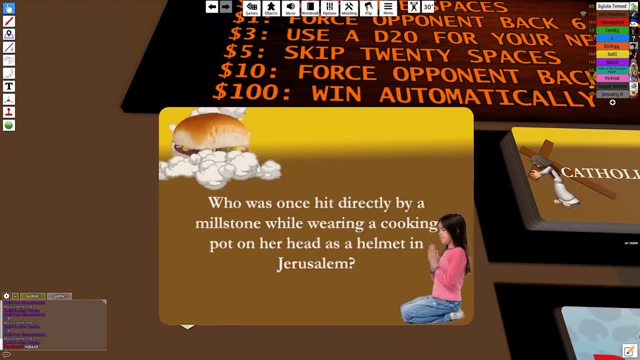 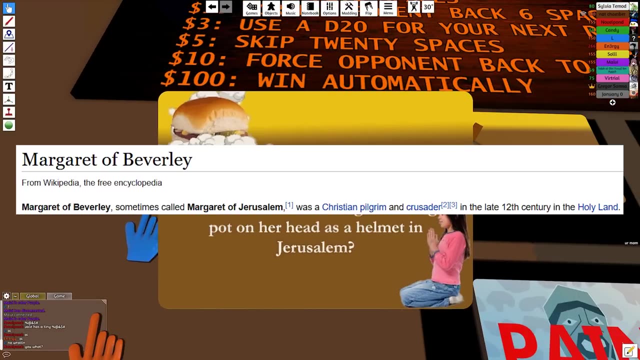 not tell me the answer. it's true, it's real. then, yeah, i remember this, we had this exact conversation. she. so she was: um, oh, it's churchill, right? churchill mary, queen of scots, that's what you're saying? no, i'm afraid this is margaret of beverly. uh, we only know. we only know about her because 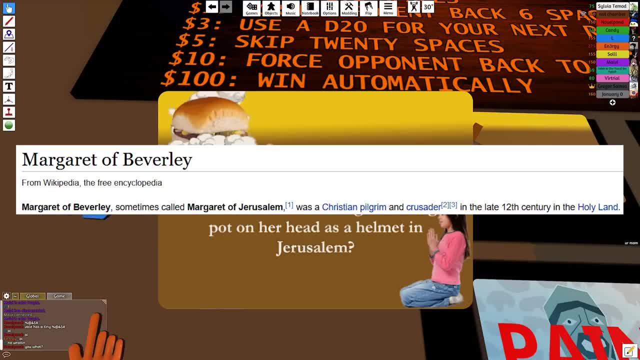 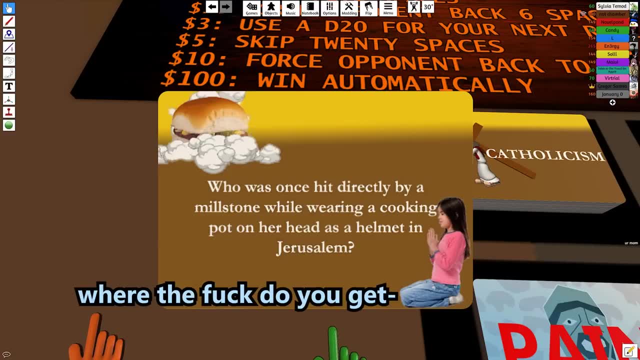 her brother, uh thomas, was a monk in england and he wrote a first person poem describing her time and her journey as a pilgrim to uh jerusalem. you would- literally you would not know this unless you had read the account yourself. how the fuck do you get hit by a millstone, though? i don't know. 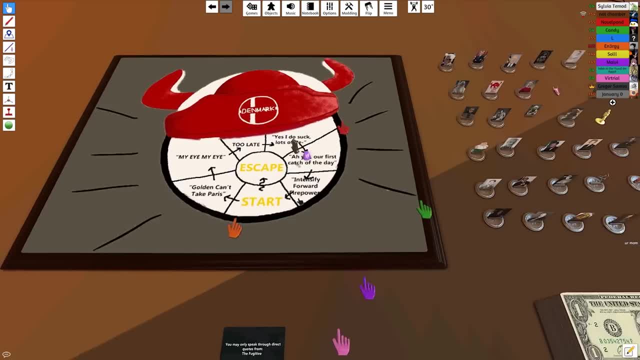 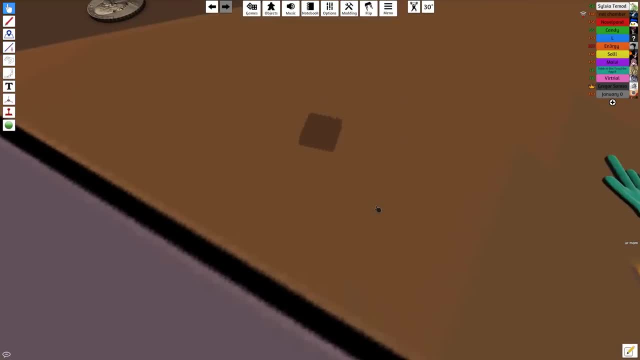 catapult like that's just what happens in the poem. i don't know what to tell you. it's teddy's turn. oh, here we go. now we get to talk about the crypt board again. about time, what do we got six. oh, very good roll, very good roll, teddy. one, two, three, four, five, six. 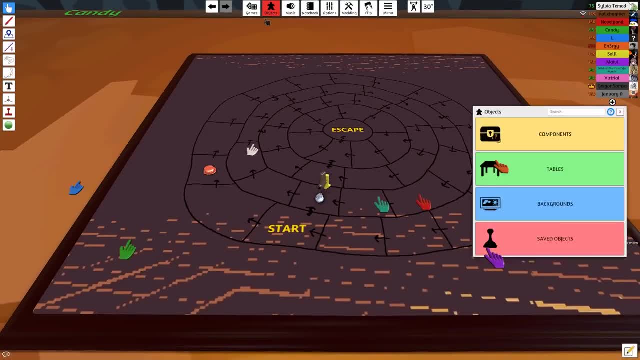 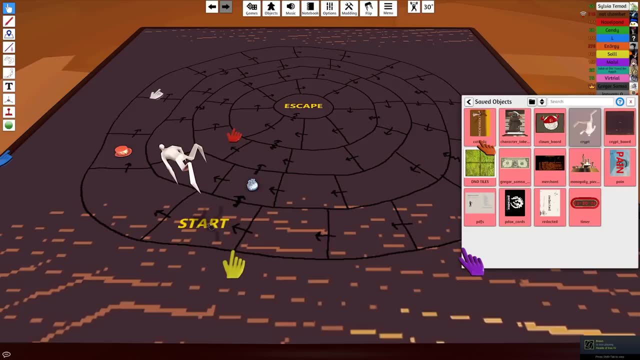 teddy actually could get out of this. now here's how the cardboard works, teddy teddy has. by getting to this ring, he has obtained the first key in the game of crypt. this means that the crypt monster has spawned one, and it's now going to also join you, by the way. 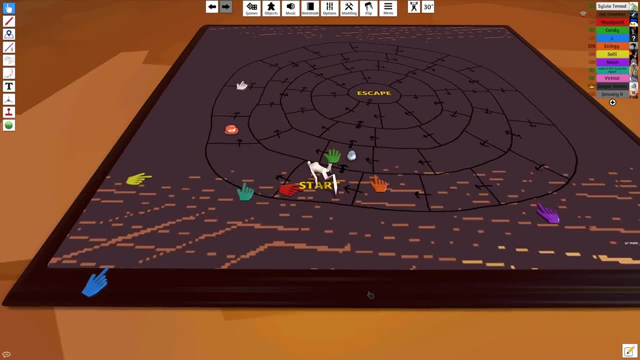 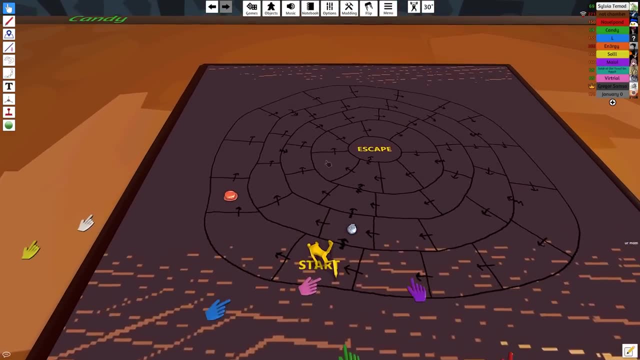 chasing you around the board. now, novel, you have. oh my god. uh, it is using a d6 right now as well. um, so as long as it rolls a one, you don't die. what happens if i die? you go back to start. if you get to escape, you go back to where you were when you got sent to the crypt board. uh, whose? 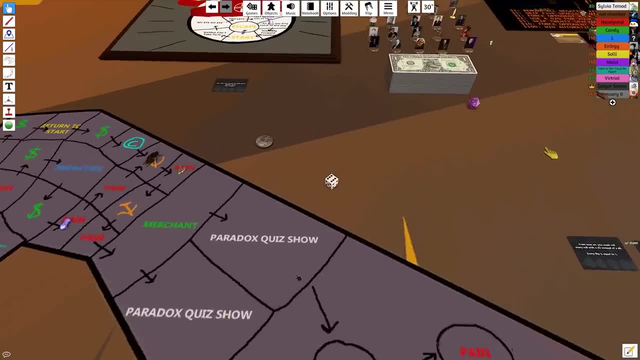 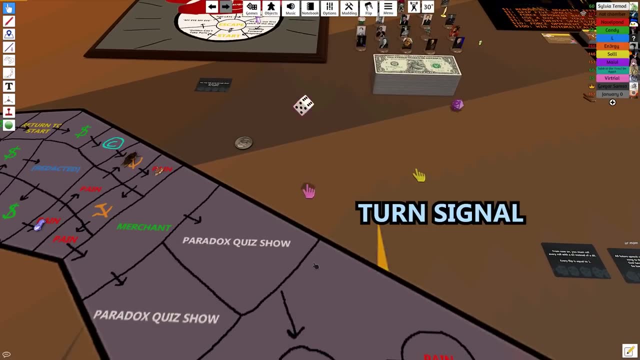 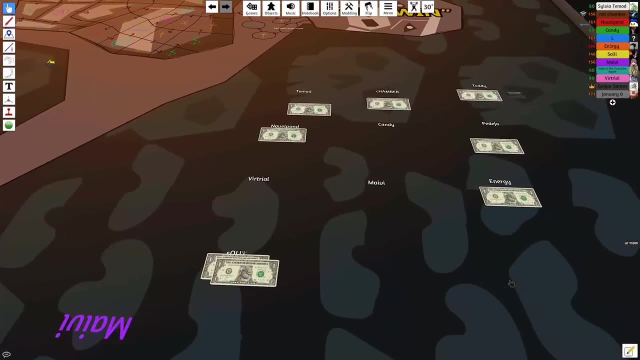 turn is that? right now it is virtual's turn. sorry, it's uh shrek. it's star wars, shrek's turn. speaking uh french signal. oh yeah, you make a car noise. i forgot. i was like: what the? do you have money? you can get rid of everything? oh, you don't. 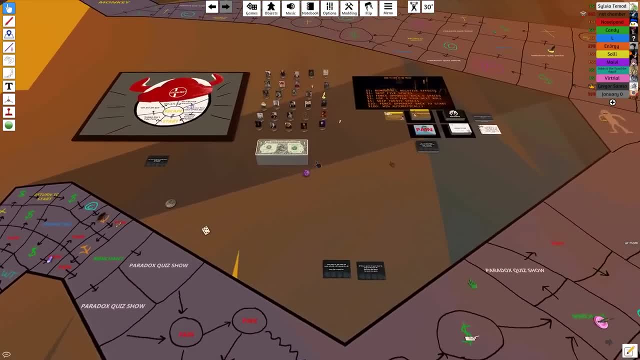 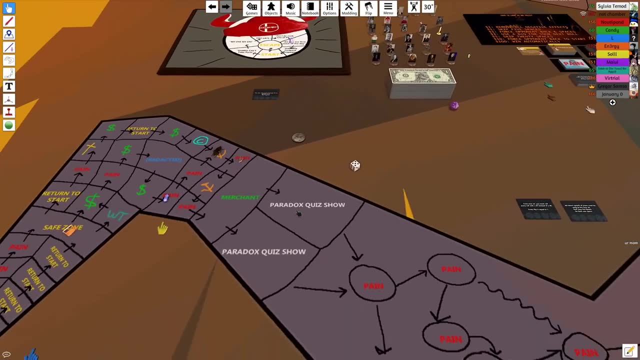 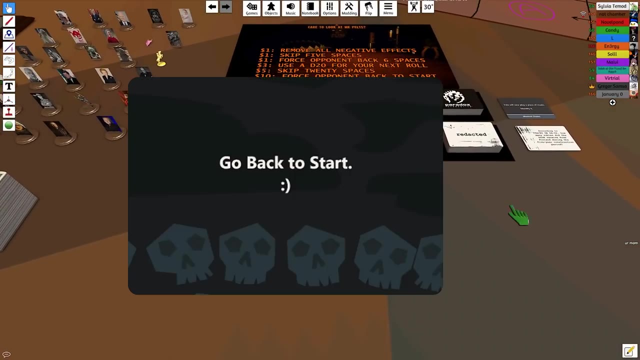 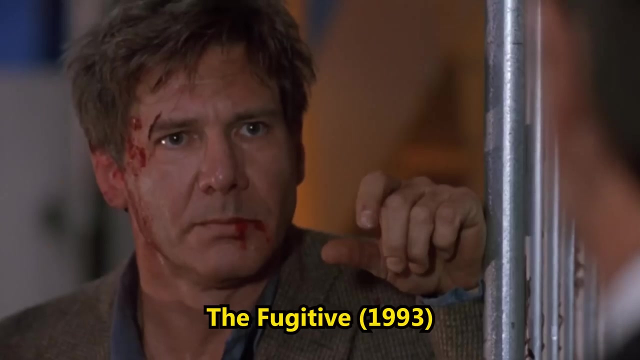 i'm lucky. no money can't spend. you remain a star wars shrek making car noises. i have a bad feeling about it. no, no, no, no, no, no straw, go back to start. well, you were in seconds, not anymore. they killed my wife. they killed my wife. 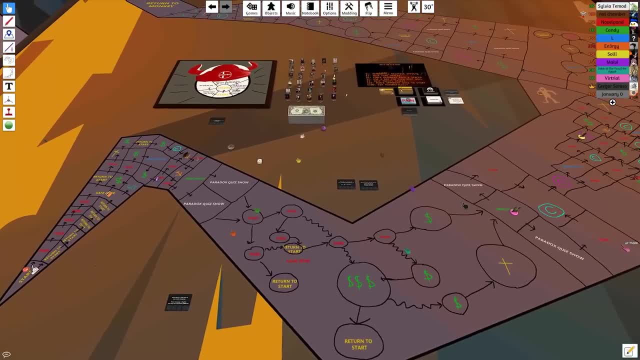 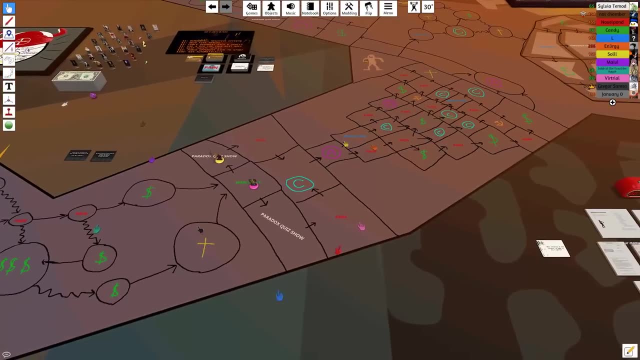 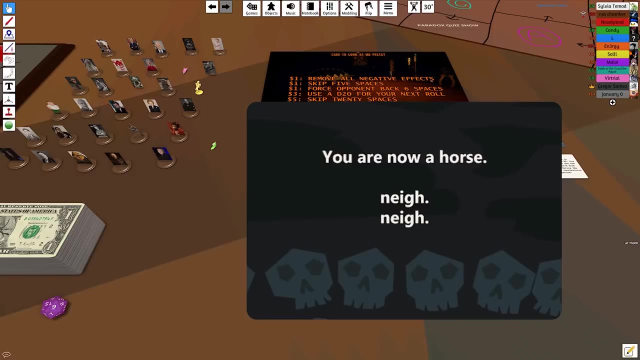 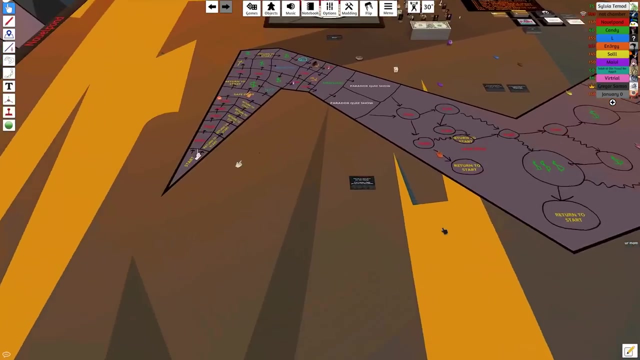 how long the clock been in one hundred percent. how to still get now. i am the migrant. you're a urbex. Praise God, freeze. delete quote on half 00. what time is it? two, three, three, four, five, six, six. you're on paradox, two writings, brother. 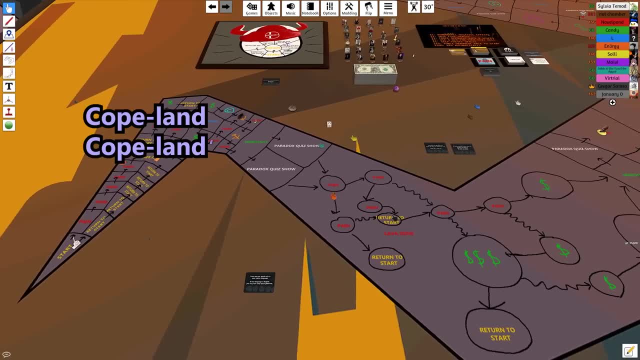 one, two, it's a one. if you wanted to get partake for the life of uihite, your whole life. members, your whole life, the rest of your life, your entire life. Copeland- that's a quote from the movie, because that's someone's last name. 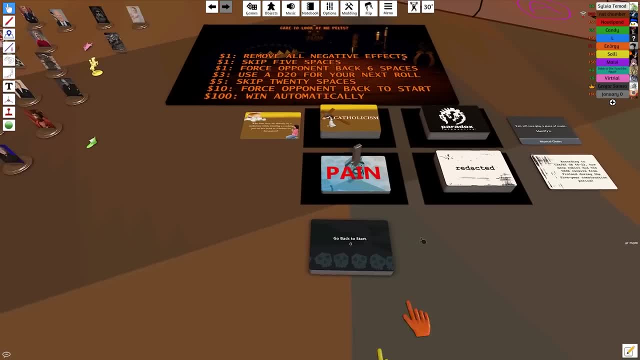 No, Someone just says: Copeland, It is All right, Candy gets to draw a paint card. I'm going to say there are only 16 left before we reshuffle these, and I know one of them says: send all back to start. 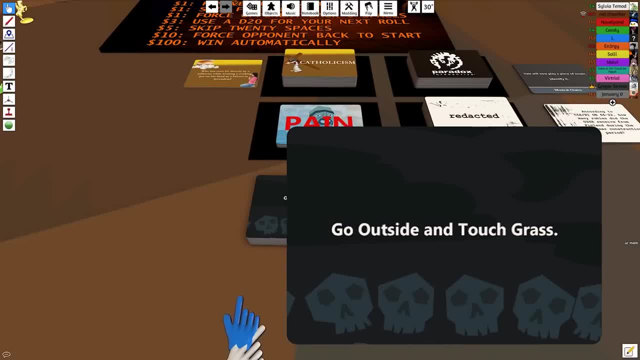 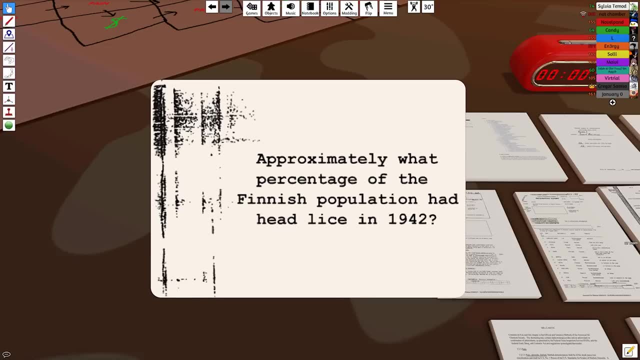 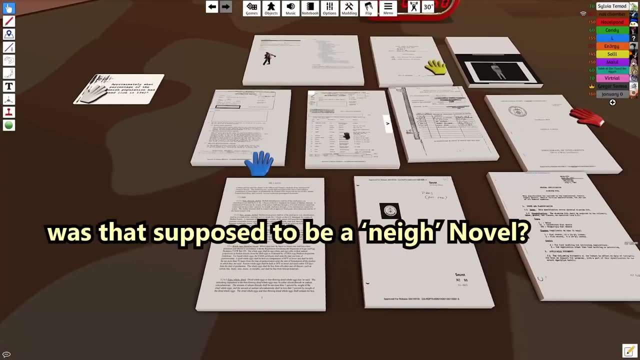 Oh God. So go ahead, draw one Candy. Do I have to? Yeah, yes, I mean, if it was today's population, it would be all of them Touched grass. Is that supposed to be a name now? 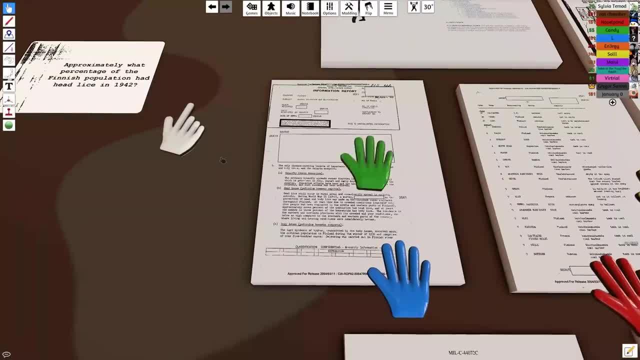 Sorry, were you making a siren noise when the cops are chasing him in The Fugitive? Was that what that was? T-Bone? No, That's a way of going. That's true. Someone does say no in that movie. 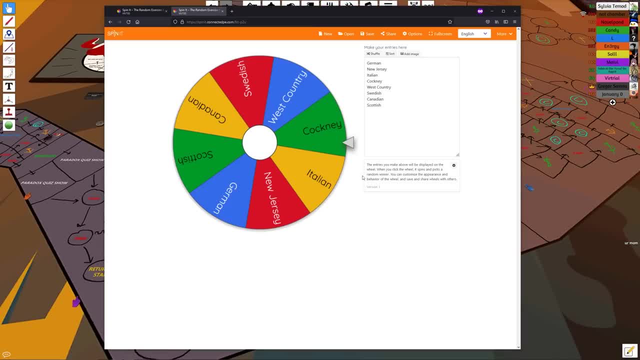 Yeah, so Virtro gone. You have Oh accent wheel. Okay, so you're no longer Shrek, Instead you are Koknai. No, that's a character. Oh no, West Country. You had to do a West Country accent. 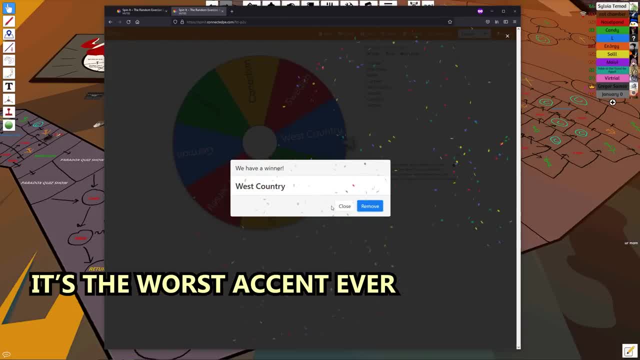 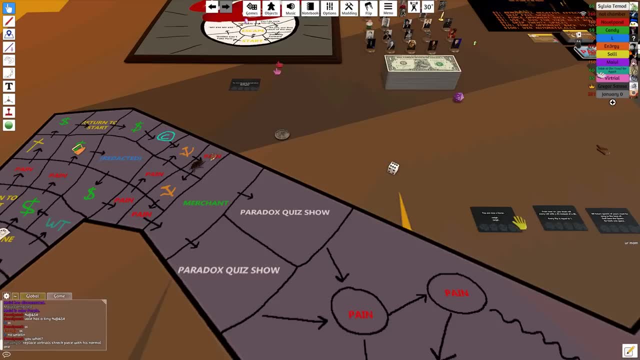 It's the worst accent ever, The actual. I don't understand how you do it. Yeah, so now you're no longer. Now you are a West Country Star Wars quoting car. Can you roll Chamber or are you dead? It's going back to the right. 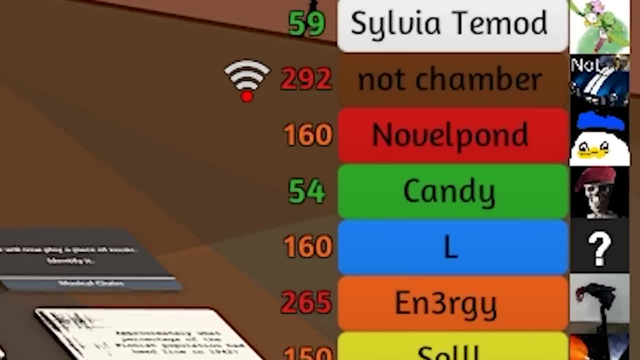 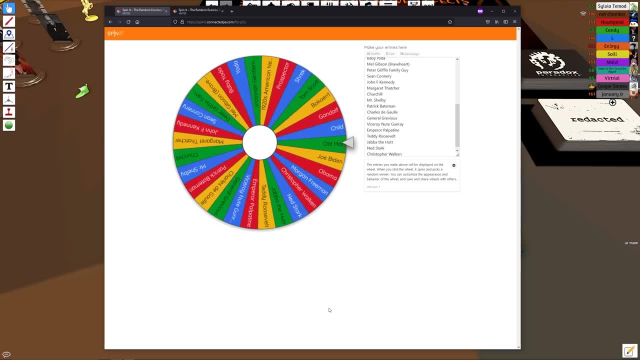 I'm still playing. Every time he speaks the ping goes up Four eight. There you go. Okay, You're an old man now. Novel Jesus Christ. Oh God, There he is. Is that the old man? 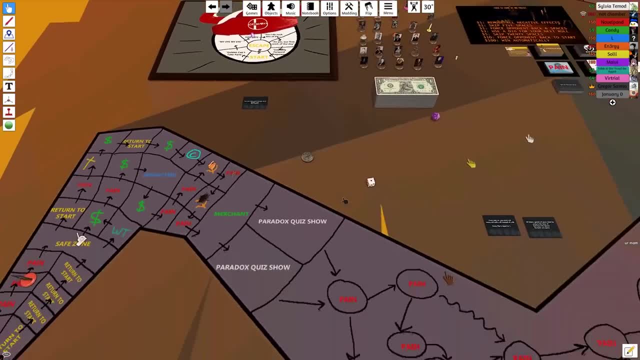 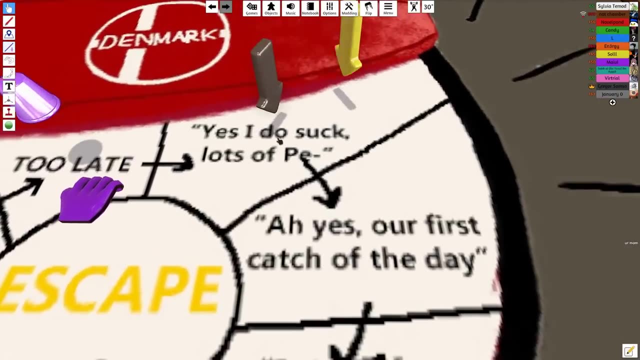 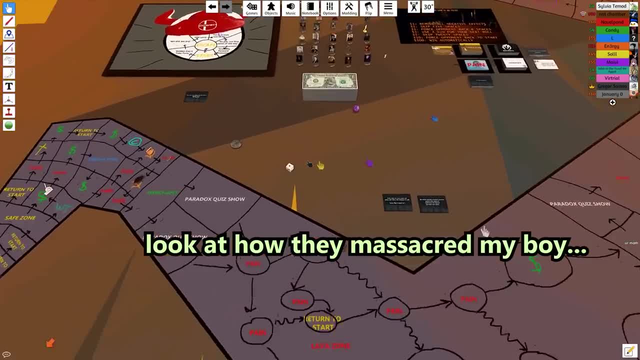 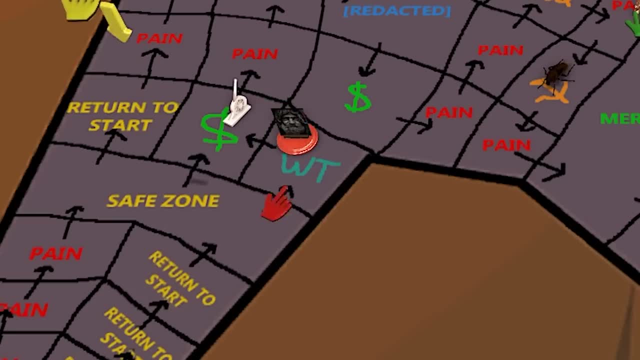 No, I'm so sorry. No, Okay, let me ask you my question. Chamber, don't forget to say nay, Novel, Nay, War Thunder, War Thunder. Do you have War Thunder installed right now? No, Prove it. 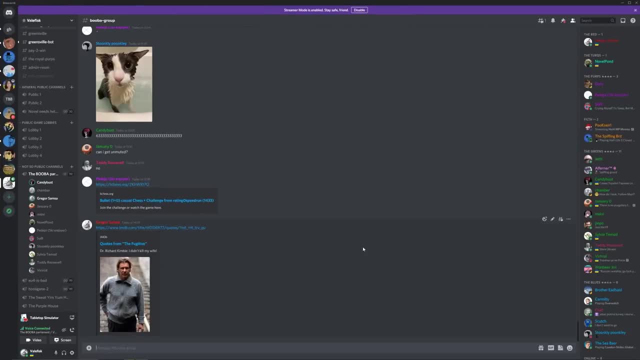 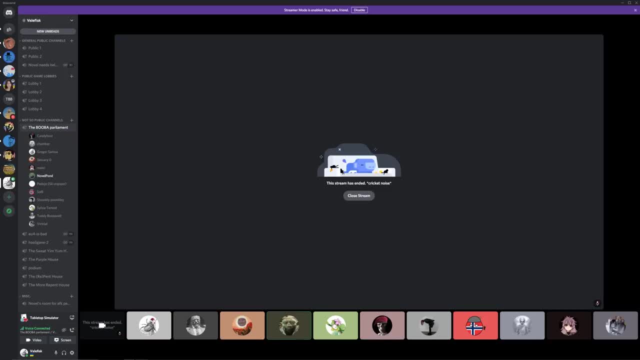 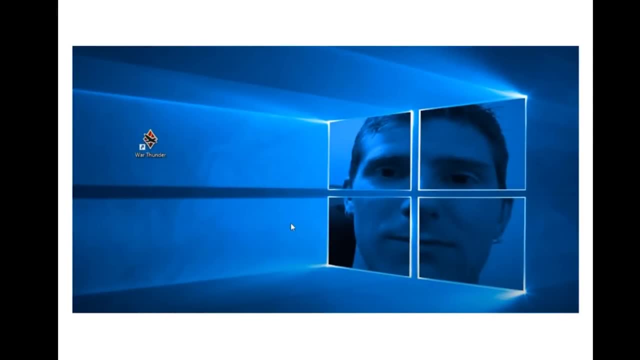 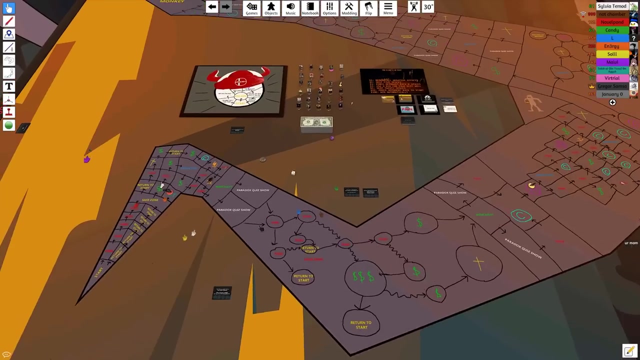 I see something opening. We can't see what it is, but I know you just opened it. Let me show you. Fuck off, Alright, I don't think he does. I don't think he does, He's fine, We'll let you through on this occasion. 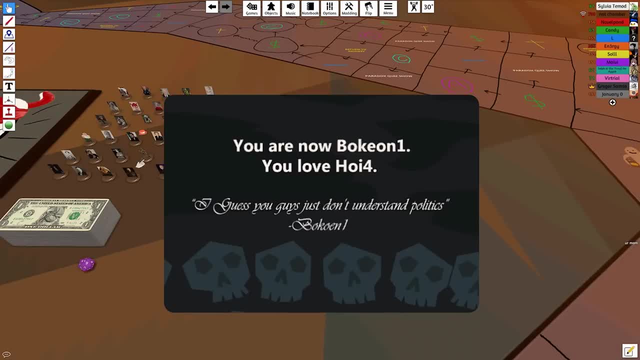 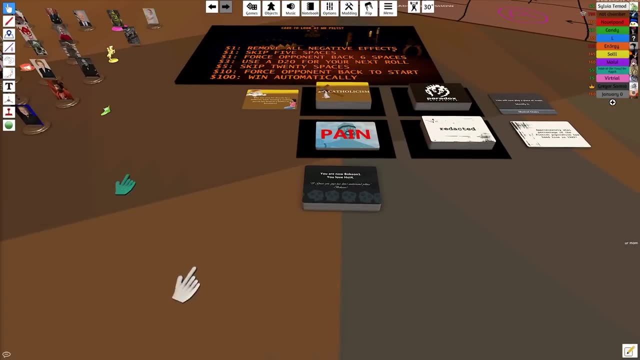 Candy's turn. Oh, I love you. You are now book code one. You love Hoi4!. Anyone see the most recent post on r slash Hoi4 encirclements. Holy shit, It was fucking amazing. Shut up. It's Pettishow's turn. 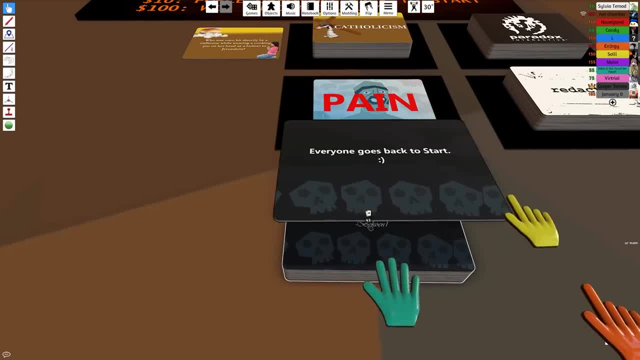 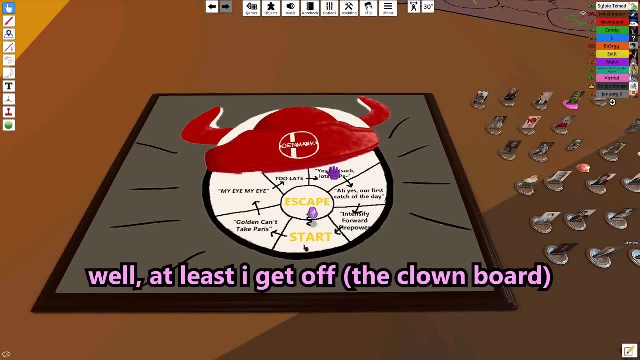 There are 11 cards left. There are only 11 cards left before we reshuffle. Fuck's sake, Pogos. At least I get off. No, no, no, You go back to the start of the clown board, so you get next turn to escape. 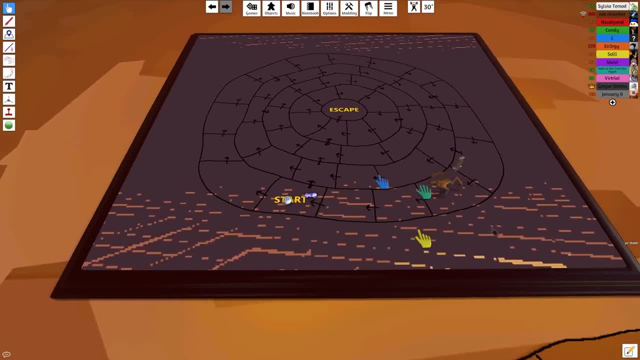 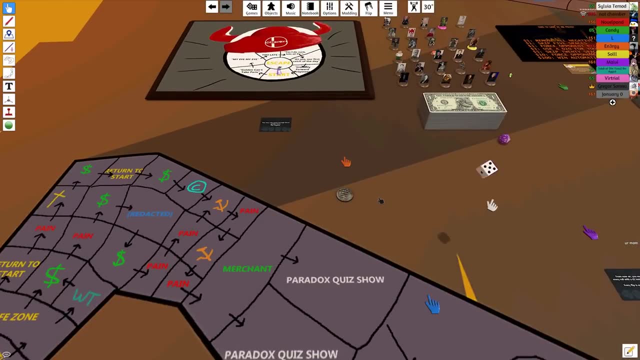 These two guys go back to the start of the crypt board with the monster right behind them. No, Maeve's turn. Maeve actually gets out of the clown board. now She gets to play the game. Hell yeah, I'm scared actually. 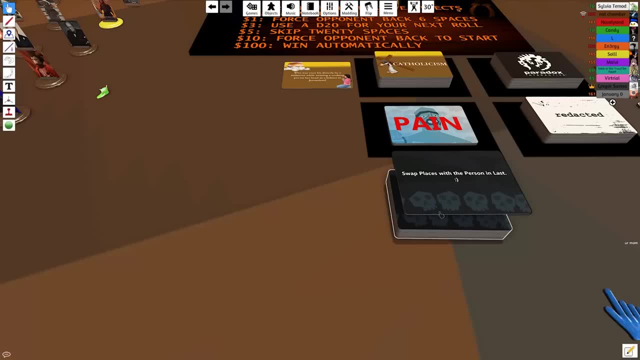 Until you land on the clown board. So one. and then you get to move four on the actual board, Swap places with the person in last, Wait me- and Pettishow- Yeah, one of the crypt board people. You go to the crypt board. 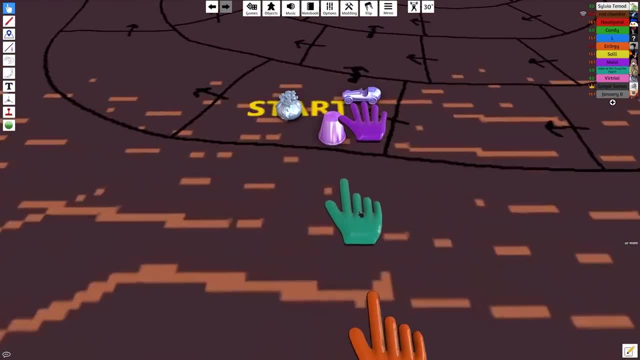 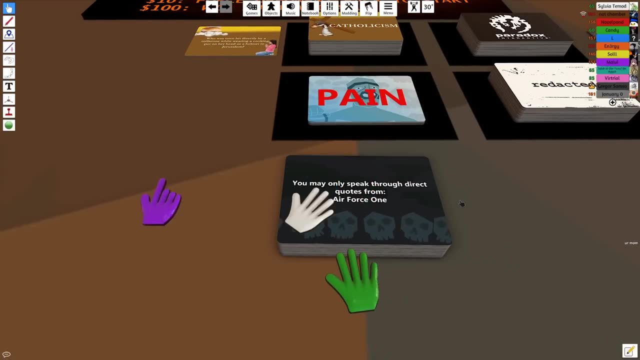 Take me Straight off the clown board. Virtual's turn. Oh, good news. You're no longer doing Star Wars quotes. You can only do quotes from the famed Harrison Ford film Air Force One. Remember what you told me? Yeah, that's right, Richard, I don't care. 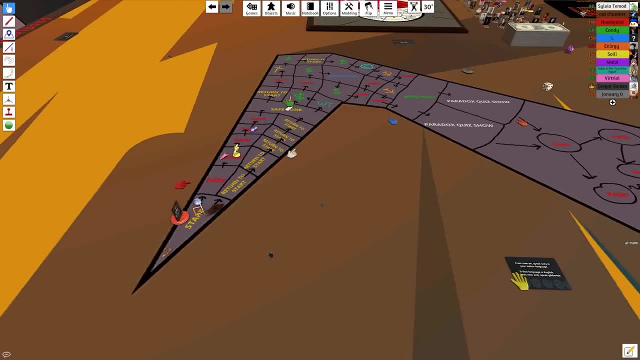 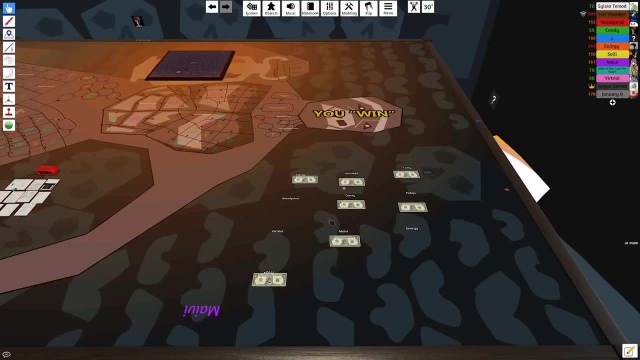 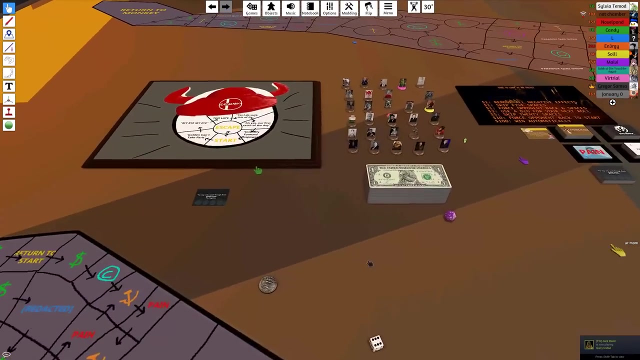 Uh, Chamber, have you finished 2048?? I have not. Would you like to spend a dollar? I have one dollar to spend. Stop singing. It's Toon Now. I gotta say the queen really needs to upgrade her broadband from BT. 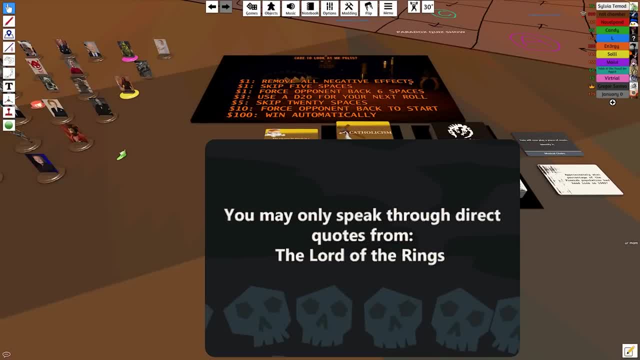 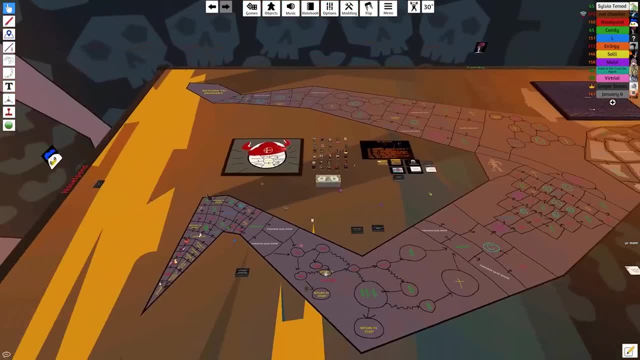 and then novel can go. So now novel is an old man, a horse and also speaking in Lord of the Rings quotes. You'll love to see it At this point. can I just be fucking Gandalf now? You basically like to say we are. 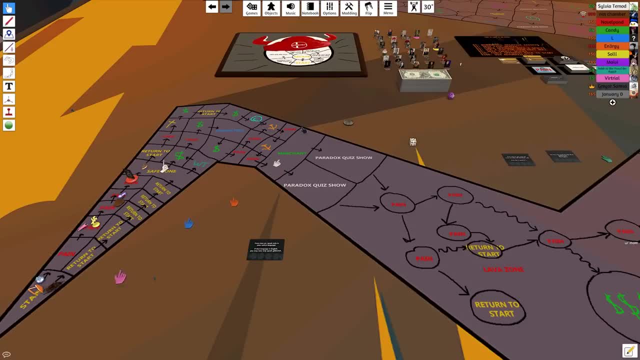 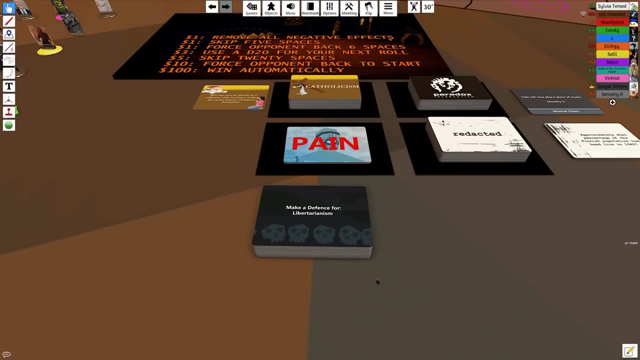 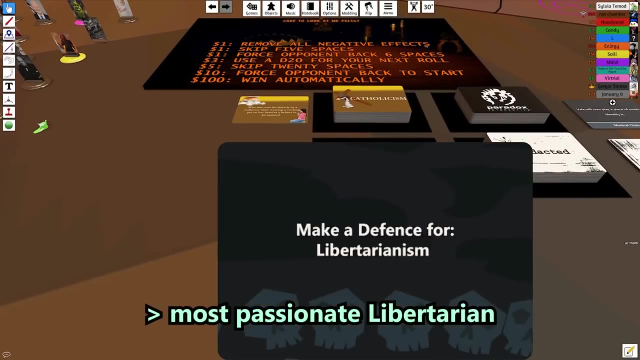 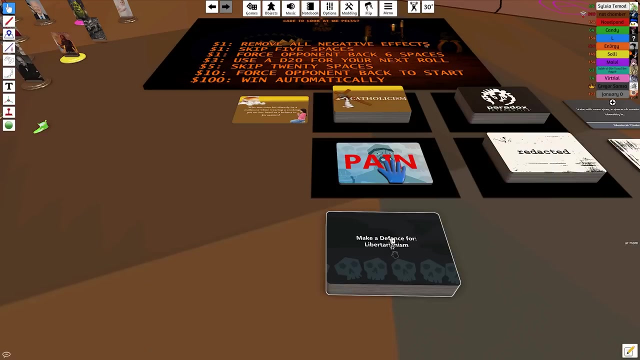 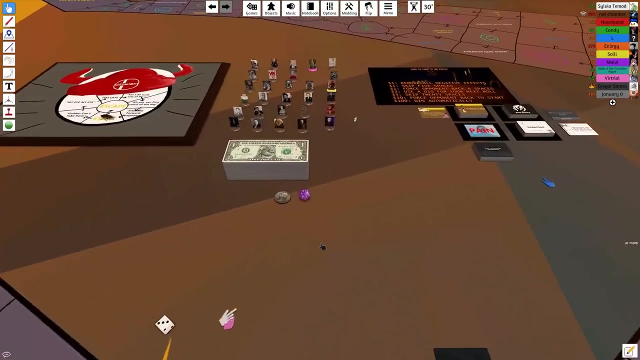 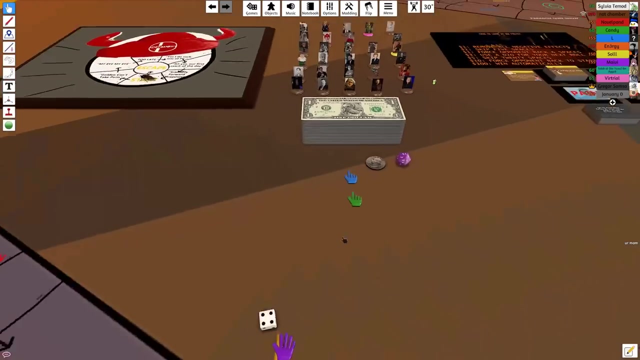 two hours in and everyone is at the start again. Yeah, Sam or caveman, make a defense for libertarianism in gibberish Cockney again. everyone's just caught. everyone is This eight, this eight On here and everyone gets cockney, except for virtual. who's what? I'm looking Germans to the Germans. 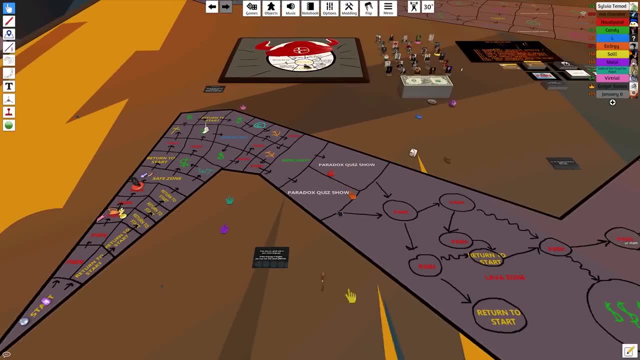 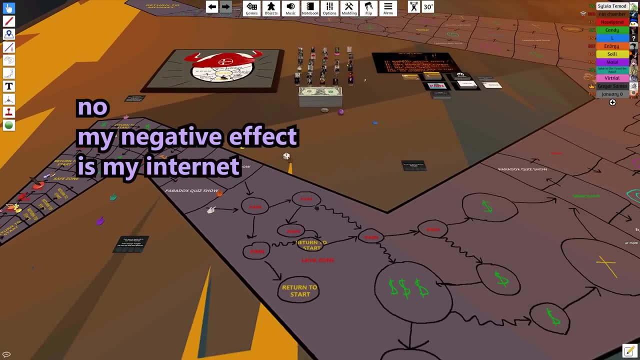 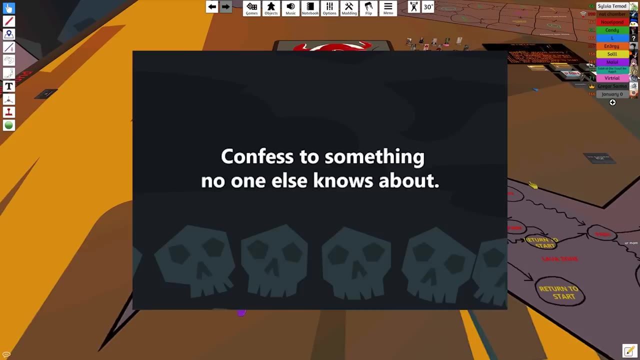 Yeah, chamber, who currently has no negative effects for the first time in at least an hour. No, my negative effect is my internet. That's not a negative effect, it's a permanent debuff. Wait, that's Gilda Sam. Sam confess, just tell. why don't you just tell the people how you use your keyboard? 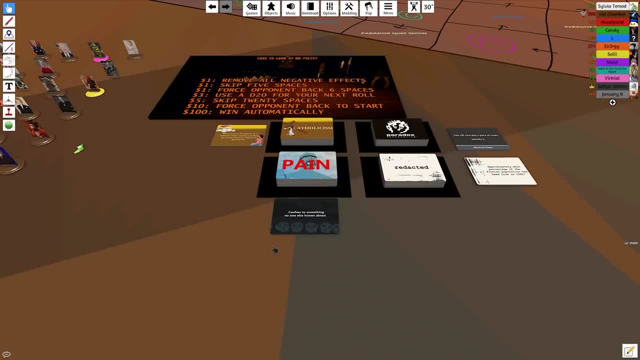 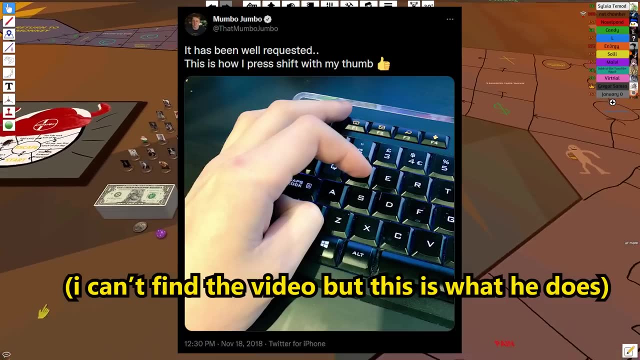 No, no, you can speak. I want you to Speak in English for this, because it's the most humiliating thing I could think of for my, for my shift. I've clicked, I use my thumb. Yeah, play the video. play the video- me in the edit of him using his thumb to use shift. and also, I have yet to. 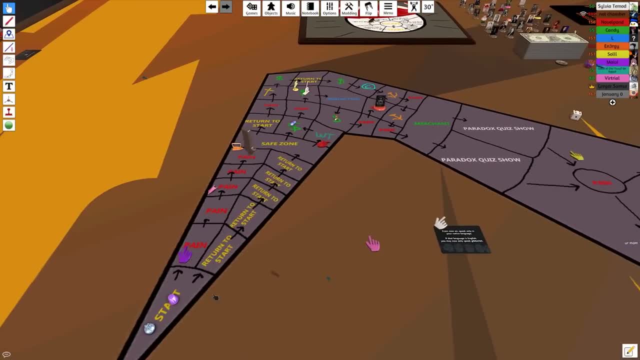 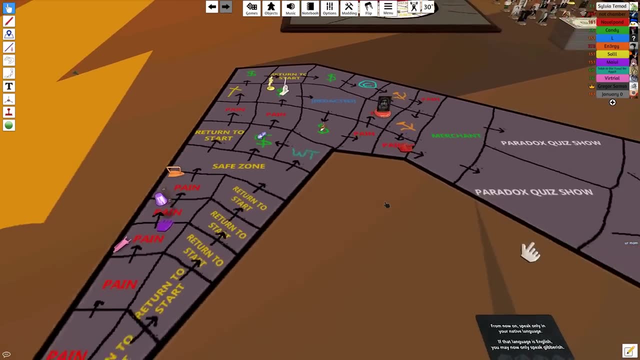 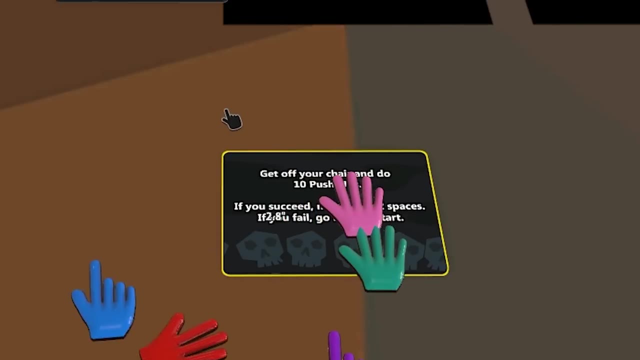 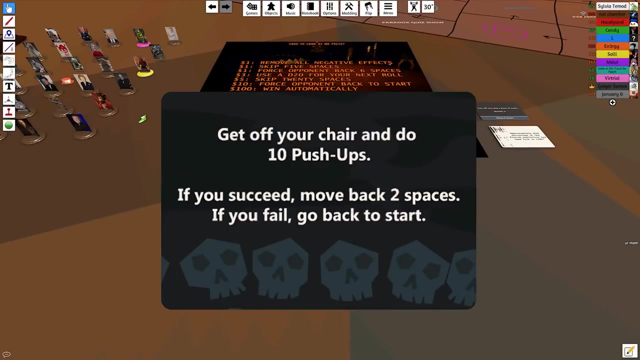 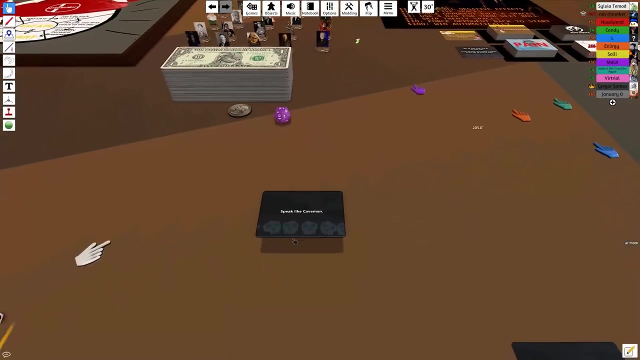 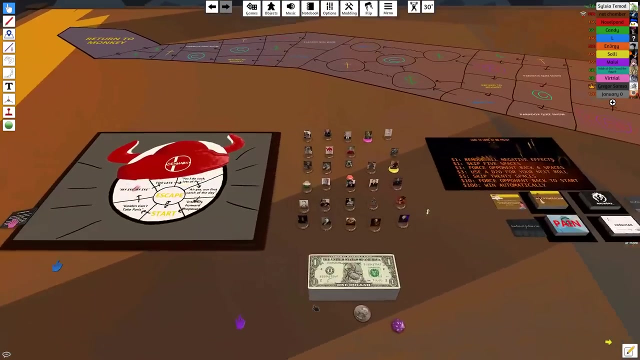 Make an accent or anything. Yeah, you've had. you've had to do absolutely nothing other than do, For it'd be very funny if you land on this and it get makes you do push-ups again. I Speak like caveman Teddy Novel, or so Gandalf, courage is found in unlikely places. 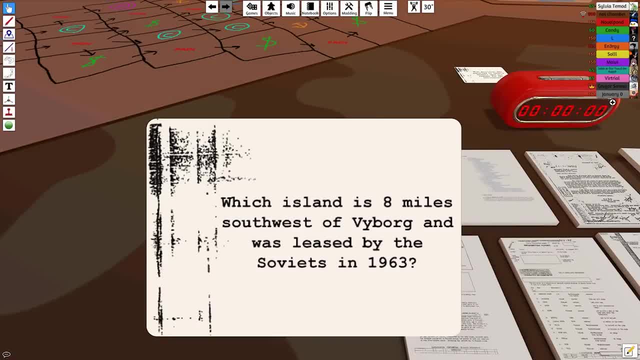 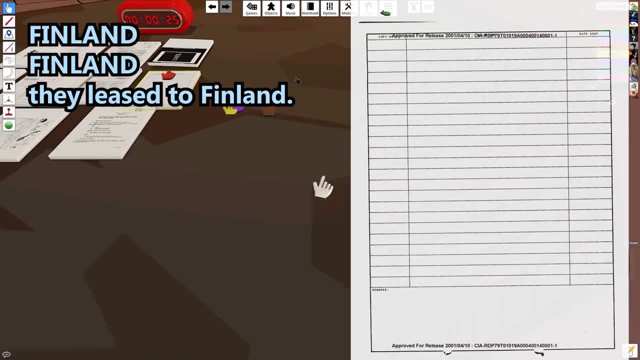 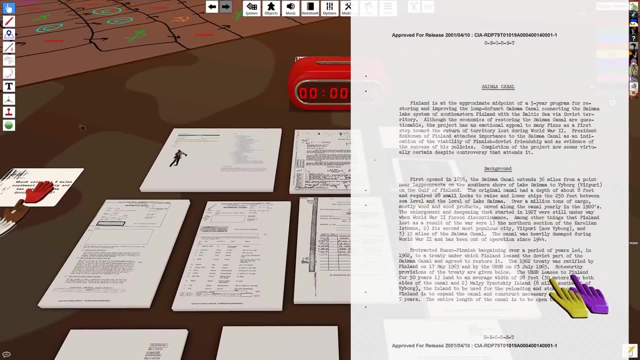 It just keeps going: which island is eight months? Let's to be Birkin- was leased by the Soviets in 1963. So it would be That's your answer. is Finland? Now I'm not very confident in that answer. I'm gonna ask if you read the question I. 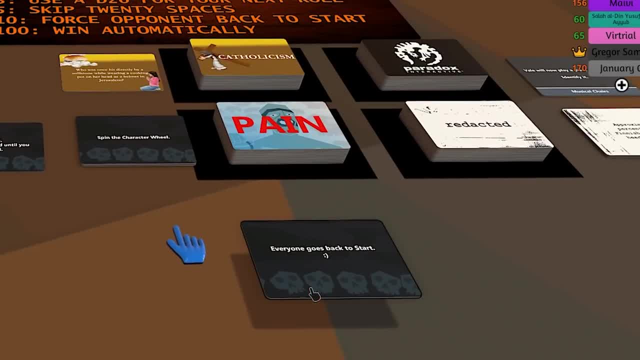 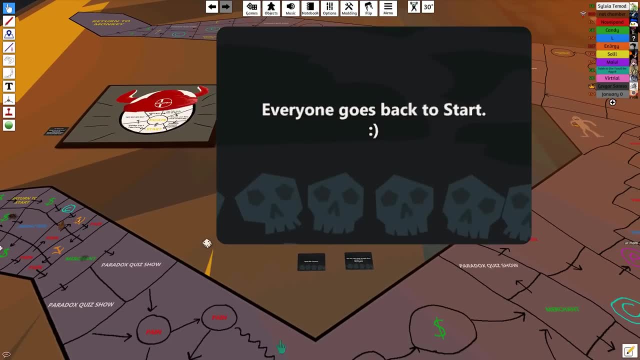 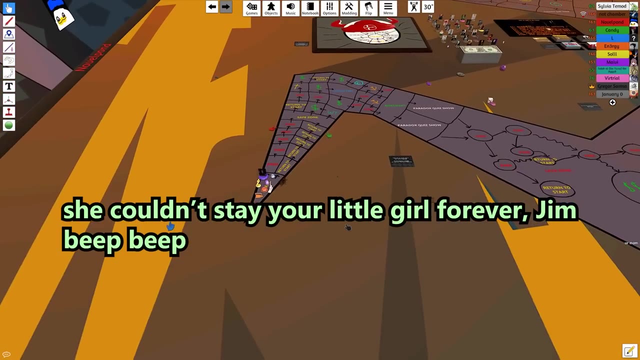 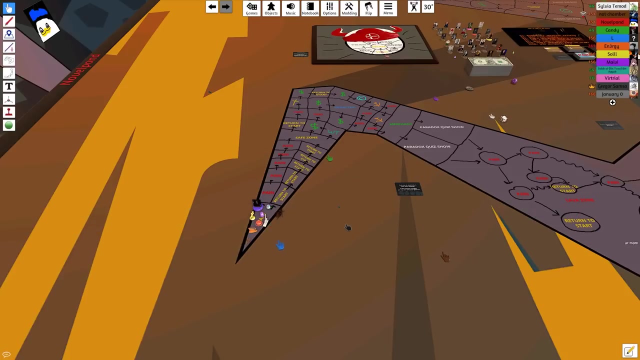 Don't think: Well, you are now, everyone goes back to start you. I couldn't stay your little girl forever, Jim, Beep, beep, Beep, beep, Beep, beep. I completely forgot. West Country Car sang. Air Force One quotes. 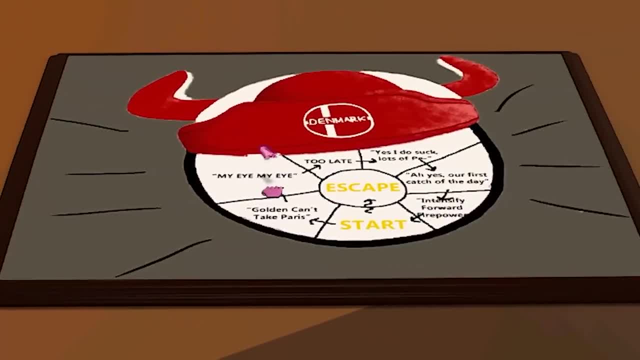 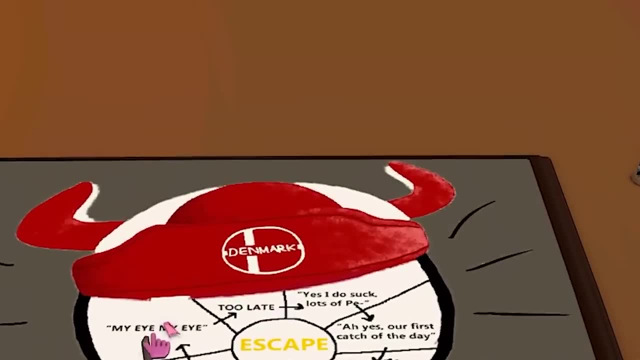 That's what a combo, Unfortunate. Oh, did you just roll two? Why did you go round and not escape? It's too late, Too late, Too late. You've committed to the climb board. You've committed. It's T-Mod's turn. 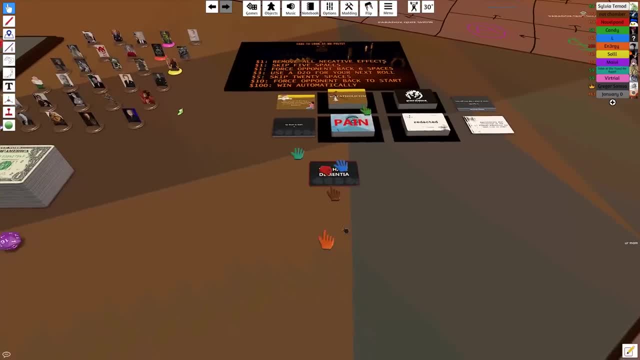 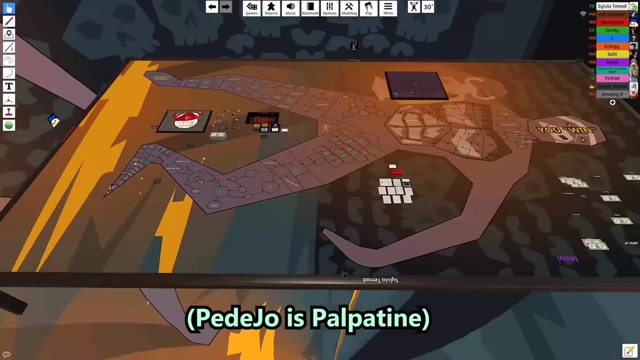 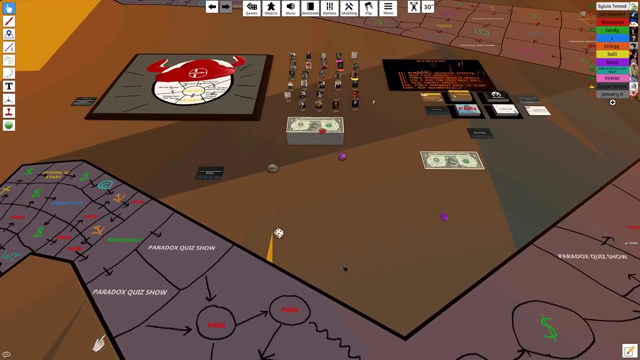 You've committed As in pain. Yes, I love you all. I will be paying to remove all negative effects from my sin. For you see, young Skywalker, I have won Gregor Sam's buck in my position. No, you guys don't know. 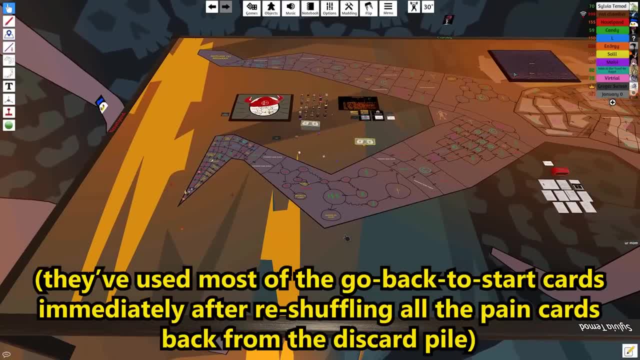 This is really good. You've used up most of the go back to start cards in pain, which means someone might be able to eke through. Yeah, we need to make it concerted. We need to make an effort to avoid the pain cards. 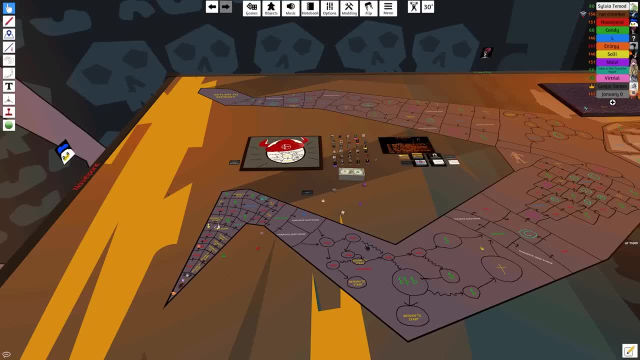 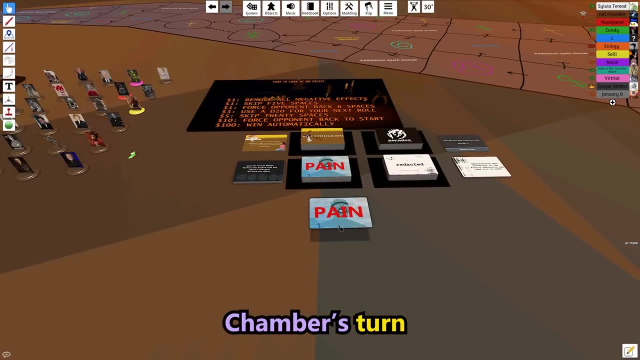 Otherwise we're never hoping. In order to beat the game, you have to conspire against me, the game master Two. Okay, That's a pain card. I like how anyone who rolls a low number is rather is wasting precious pain cards. 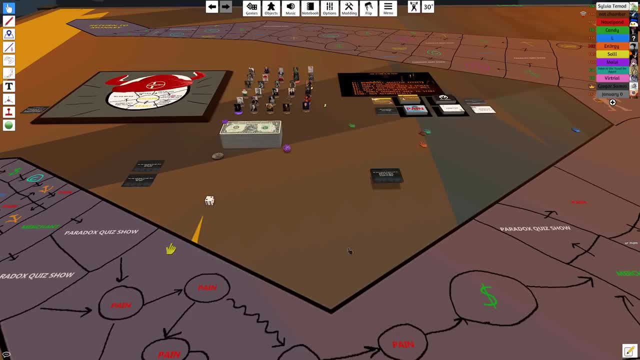 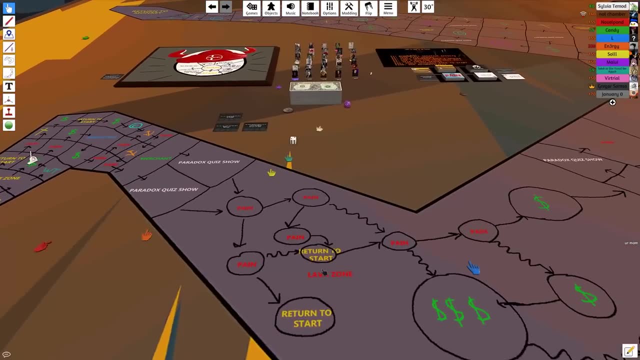 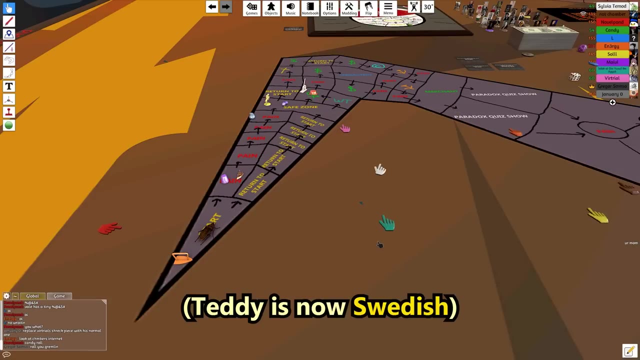 Unfortunate Chamber, Very unfortunate. Go back one space and you will be singing to the tune of God Save the Queen for the next hour. You have to roll, You have to roll. Unless you kinda mess up here Voice, They sound closer to tears than anything else there. 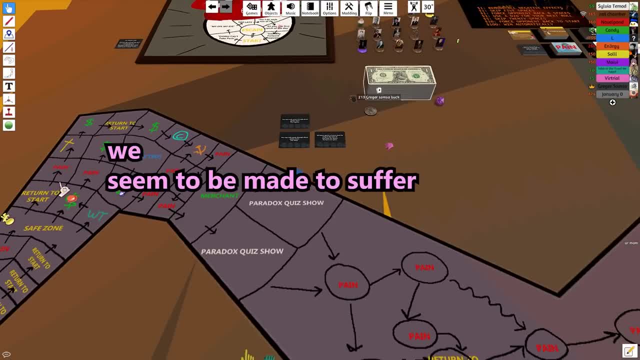 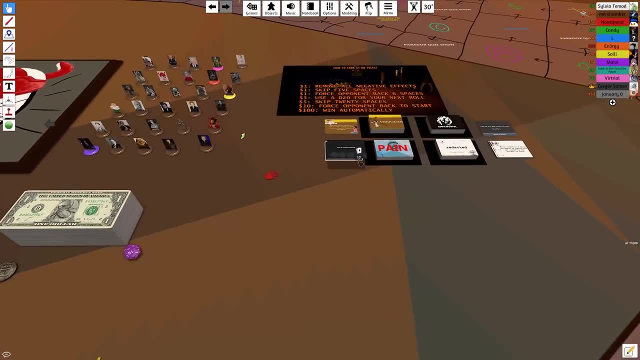 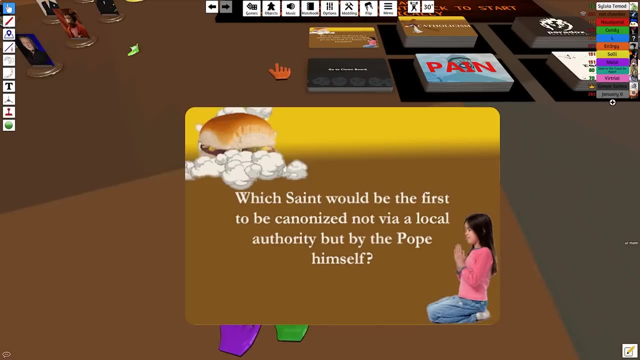 We seem to be made to suffer. True, That's impossible. Two clowns on the board now. Two clowns on the board right now, just like uh wish Saint would be the first to be canonized, not via local authority. 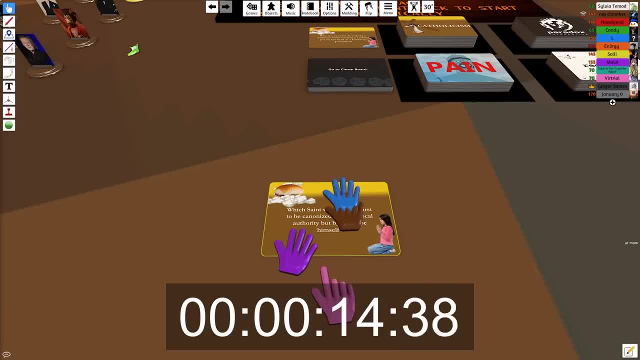 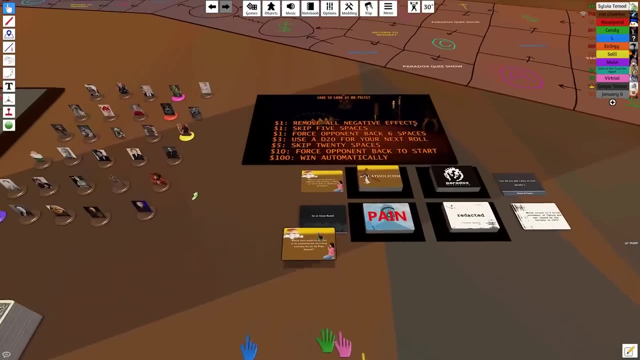 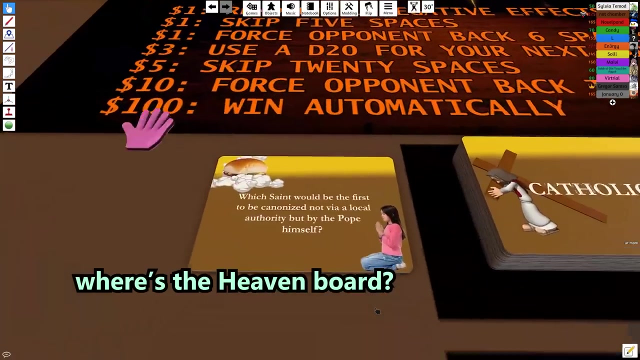 authority, but by the pope himself, richard. richard kimball was not scanning, i forgot that. i don't know these kind of stuff. if you get this question right, you go to heaven. if you get it wrong, you die. where's the heaven board? yeah, where is the heaven? and maybe the game is stuck until you answer the question whether. 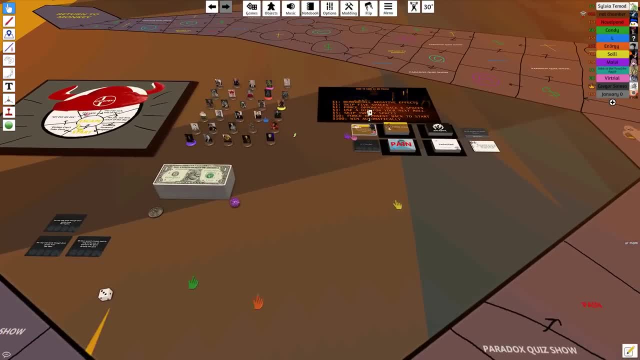 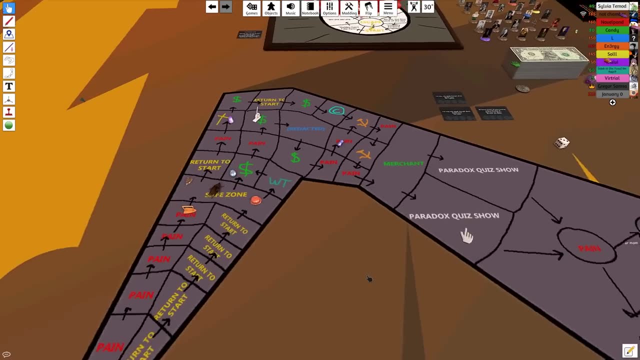 you know it or not? i know you don't. i know that no one in their right mind would know the answer to this question. that's the whole point. yeah, name even steven. no, uh, ulrich of augsburg. okay, that's close, very close. yeah, oh, play bullet chess again. petrillo's gotten this twice. 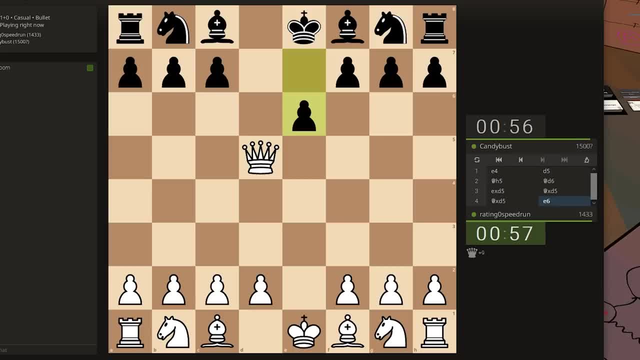 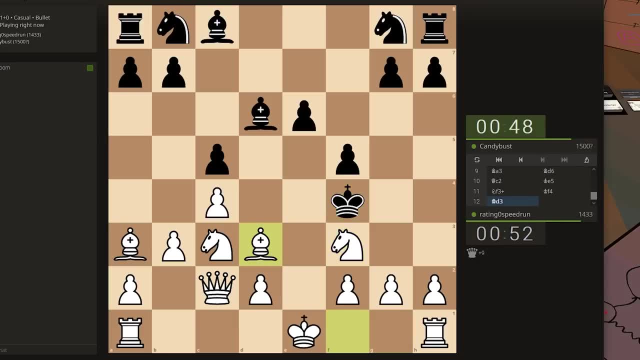 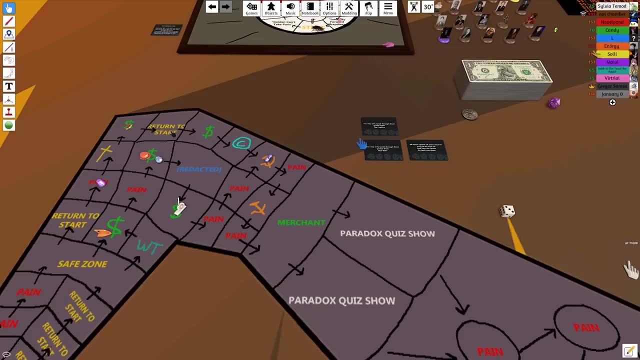 scandinavian defense declined. hangs this queen immediately, wait, wait. i only just realized what the is happening. you troll, he might get up. he might end up getting checkmated himself. here. oh, he did. maybe you just landed on return to start star wars quotes, you have to speak, maybe. 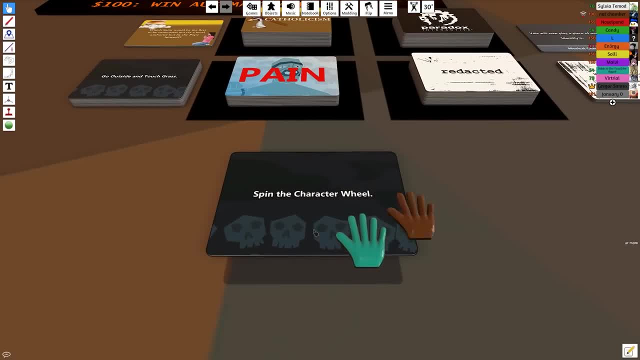 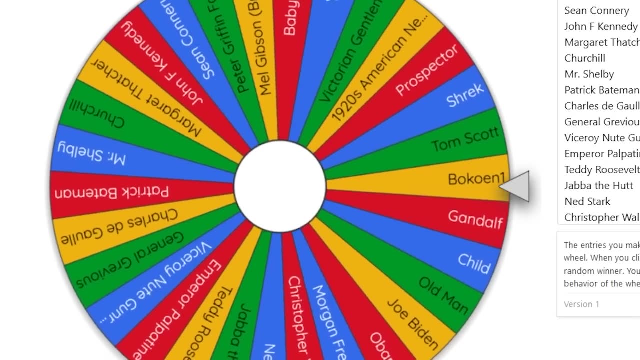 all right, i hope this just says: go back to start. no, you're a character. now, for the first time of the entire game, you get to do a voice. it's gonna be. it's gonna be someone you haven't heard of. it just landed on poco and won. 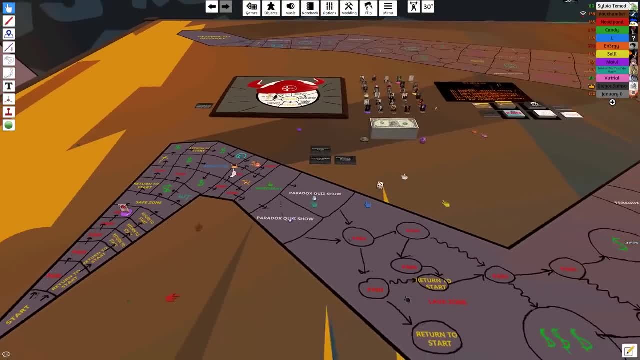 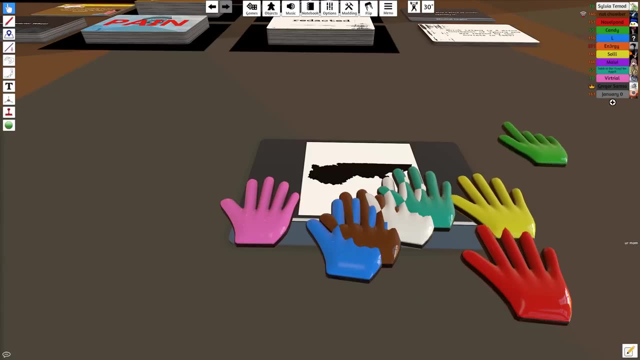 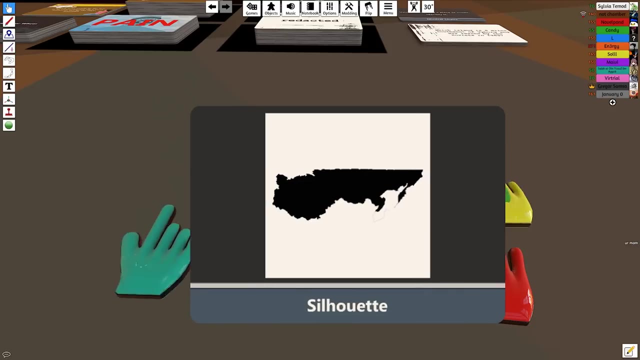 but you have to do it. oh, paradox quiz show. teddy's doing the paradox quiz show. what is that silhouette? what is that? that is uh the uh. that would be uh the uh. the russian empire from a victorian. no, very sorry, that's the russian provisional government from uh hoy. for oh what i? 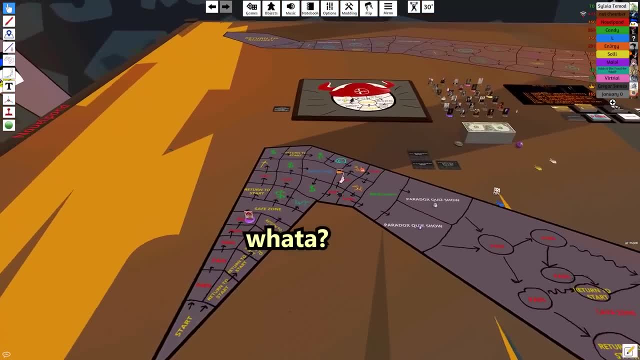 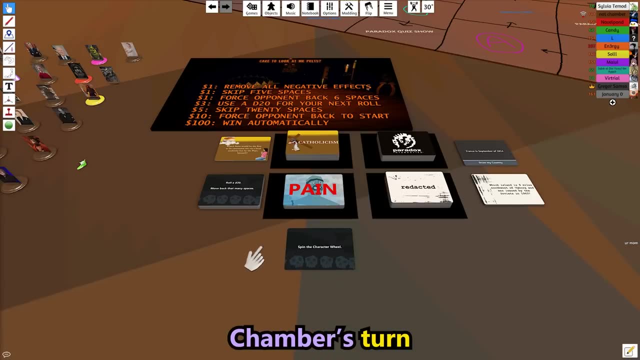 don't start at the game. unfortunate, i guess that sucks. shame. go back to space. they killed my wife and you're going to be a character. you're going to have to sing to the tune of god save the queen while in character. oh my god, i feel like this is actually target. this is targeted towards chamber. 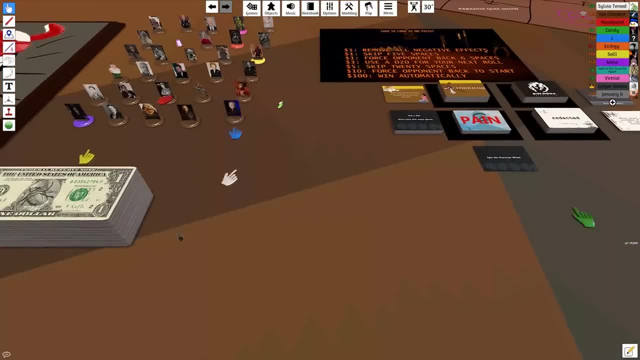 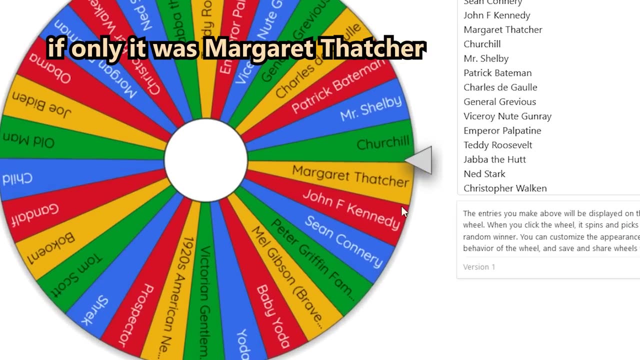 because he just rolled churchill. that's very, very apt for you to be singing god to the tune. it was literally okay. literally, like it's on the line between the two of them. um sorry, boko and juan, it's your turn and you love tinks. 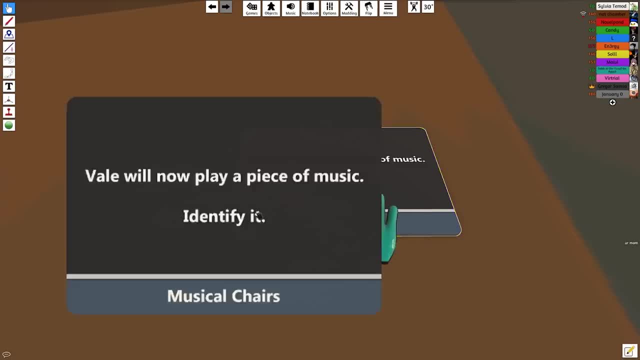 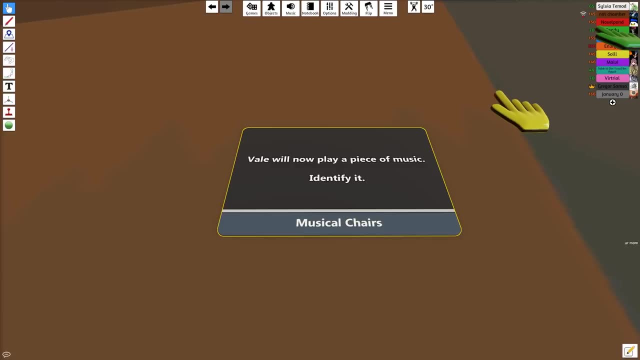 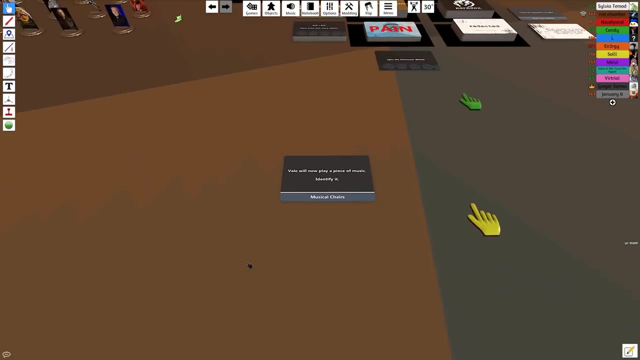 richard. uh, it's time to play musical cheers. this isn't music. can i? can i mention the game? at least that's it, yeah. so what game was that? okay, that was um march of the eagles. sorry, that was the interest in the game, but i'm just gonna hand you the game. 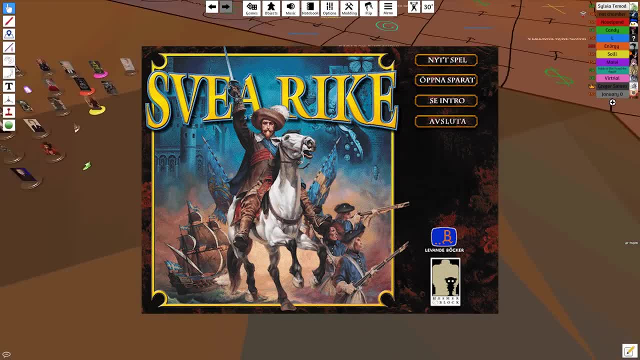 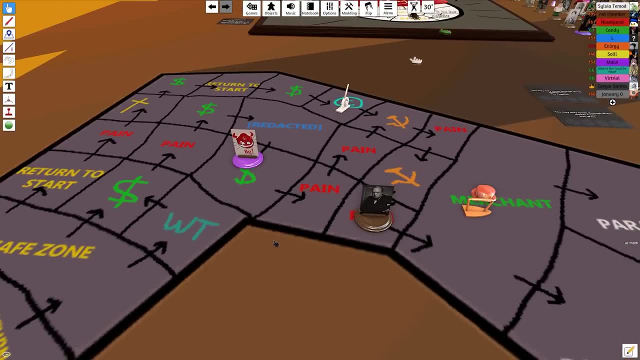 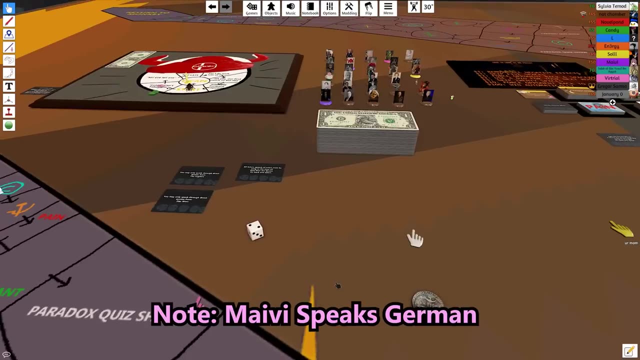 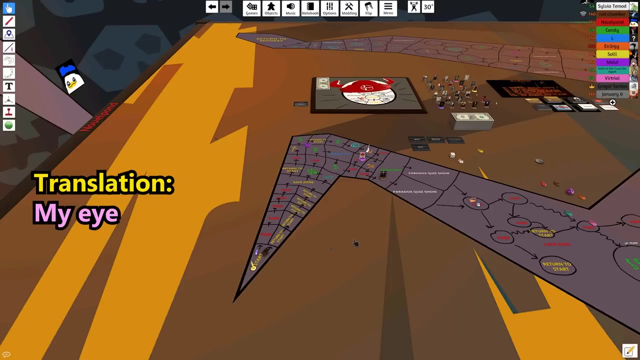 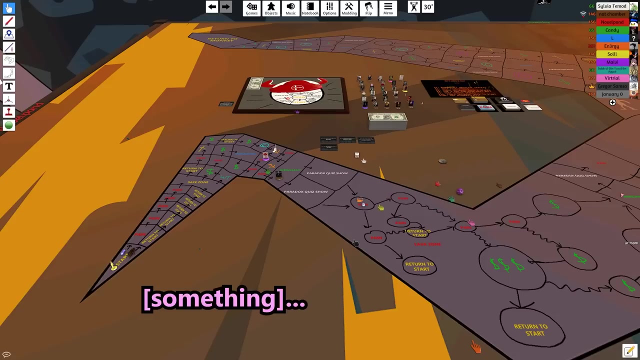 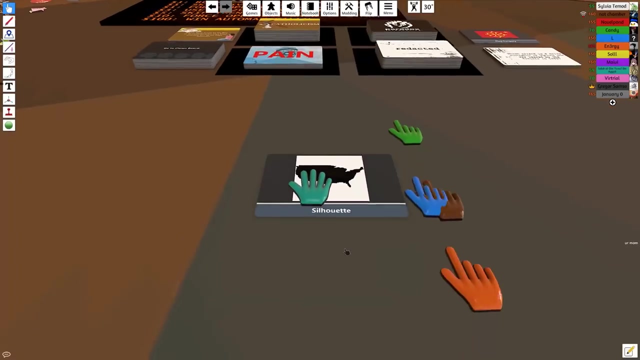 to sphere. right, you go back. it's a book on one, book on one. it's your turn. oh, unfair german accent. wow, okay, you know what. maybe you should have to speak in german. yeah, actually, good, good point, maybe you have to speak in german. okay, what's going on in here? oh yeah. oh god, what country is and which game is this from? 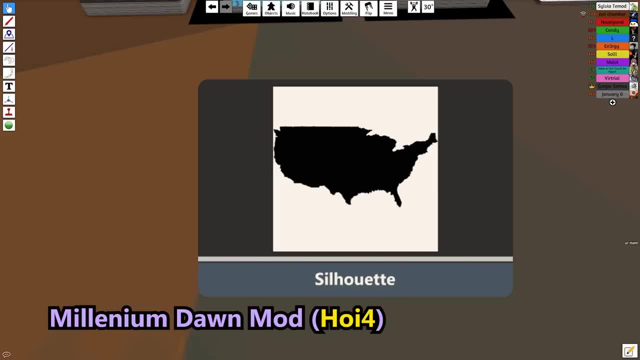 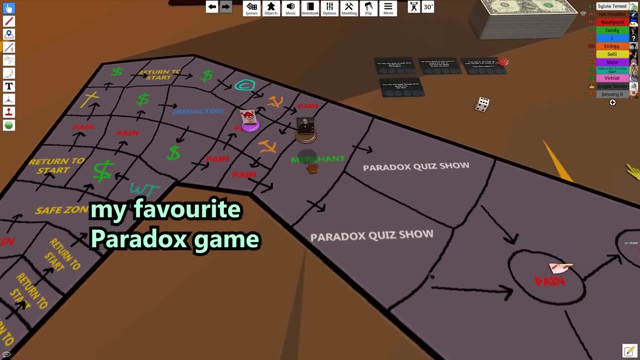 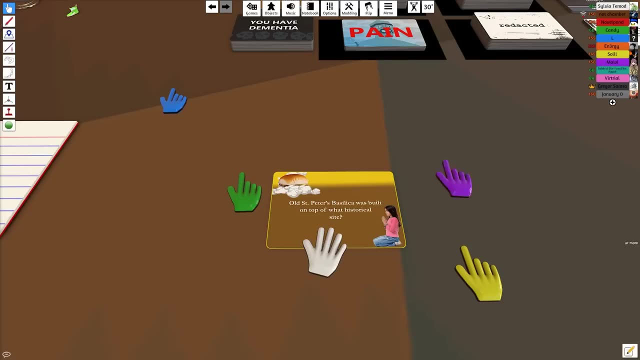 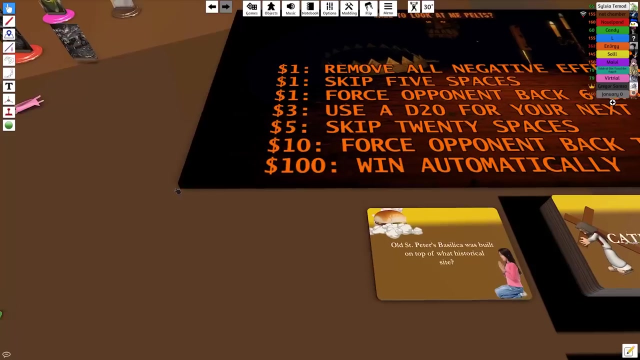 millennium dawn mode. you're very close. it's the united states from google maps, go back a square. my favorite paradox game, old saint peter's basilica was built on top of what historical site? uh, an indian burial site. yeah, it's a scooby-doo episode at saint peter's basilica. yeah, 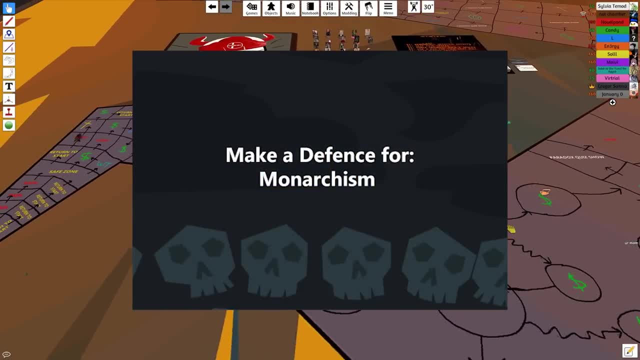 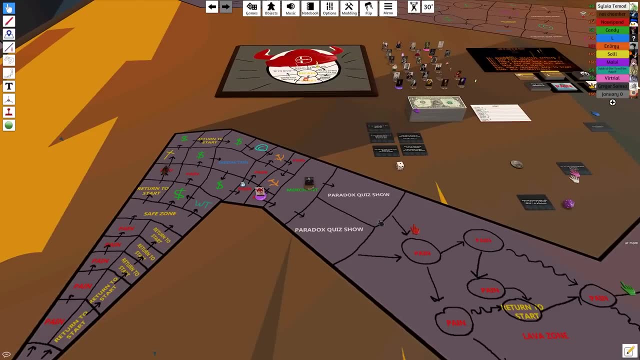 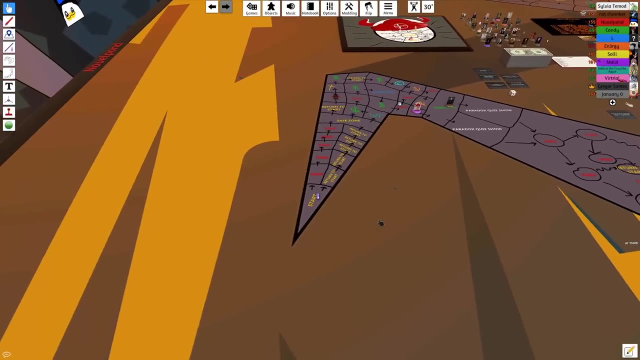 ah, depends on monarchism, depends for monarchism. so we all remember that old guy. he was pretty cool. he went over to russia. he was awesome. i like him a lot. we should be everyone's leader. i don't care what you say about inbreeding, it's a really good thing. it makes you the smarter, see, if you marry. 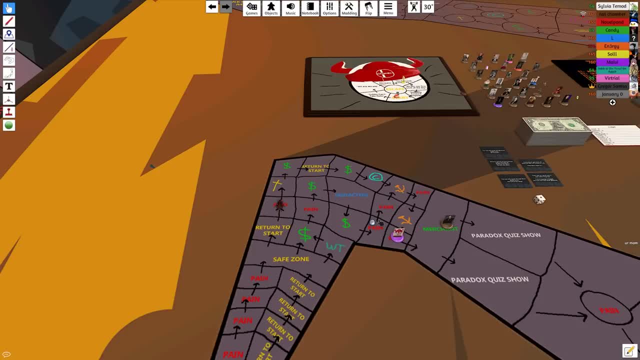 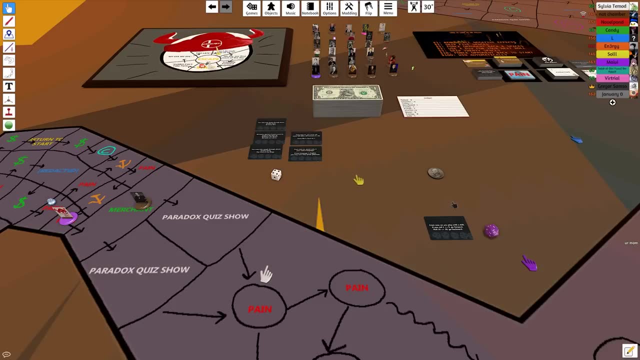 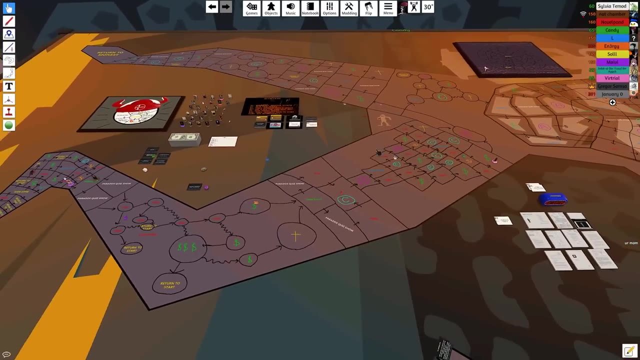 your sister, then you are awesome. if you see my sweetest bloodline, trust me, trust me with this one. i love swedish people. we are all saved mind. can i just be point out that? so god to like here within like under an hour, and then we'd just: yeah, you see. you see what i mean when i say this might. 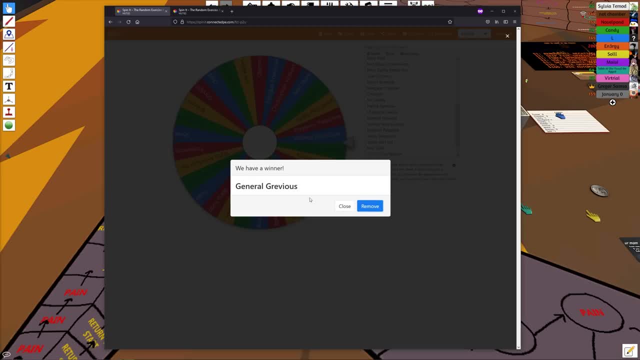 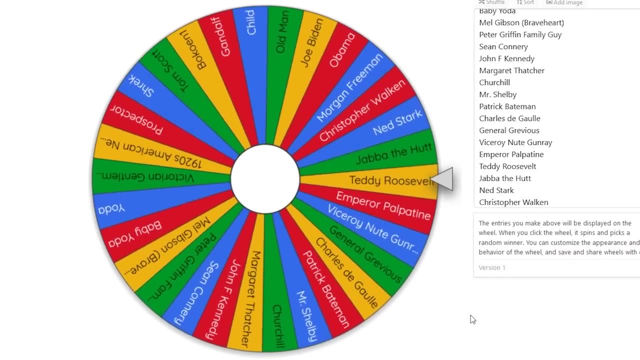 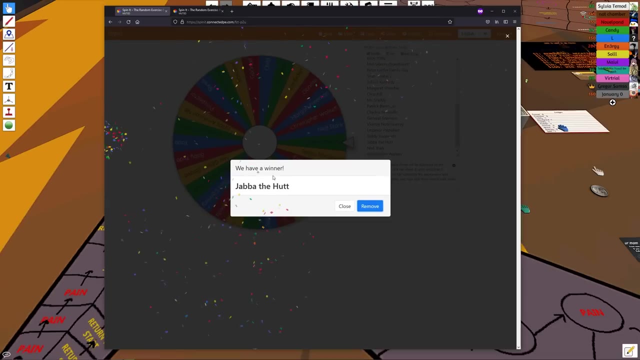 be luck. face candy, that's me character. oh, i haven't been a character in a while. who is this? i hope it's job of the hut. i really hope it's peter. i actually predicted it's job of the hut and i saw i have a recording of it. it's real. 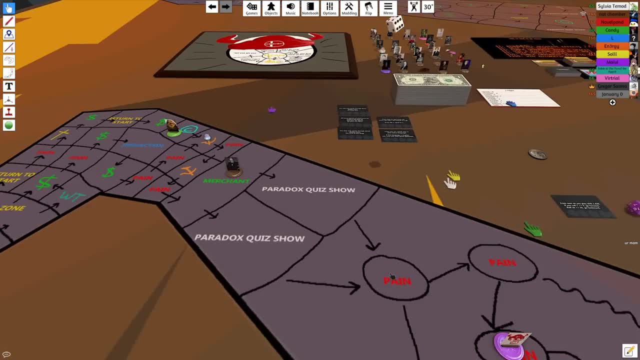 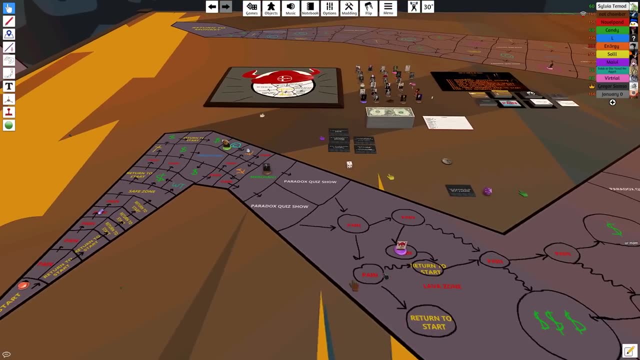 it actually did land a job in the hut. i'm not saying that it's not rigged. when i came home, there was a man in my house. i fought with this man. he had a mechanical arm. you find this man fine. to anyone who hasn't seen the fugitive, it sounds like insanity. so do you go back to start? 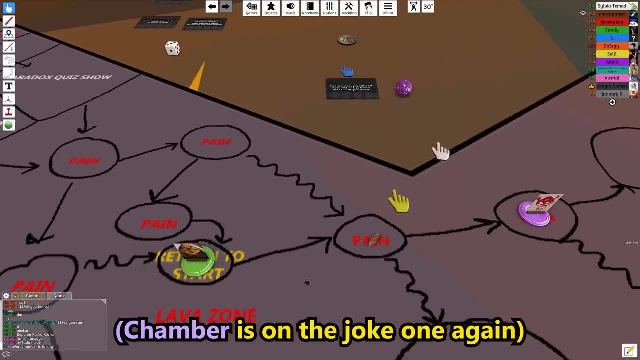 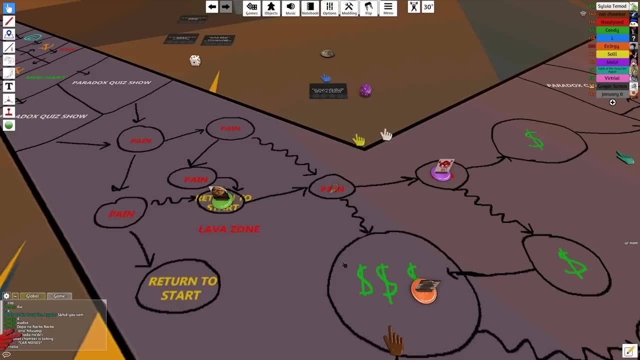 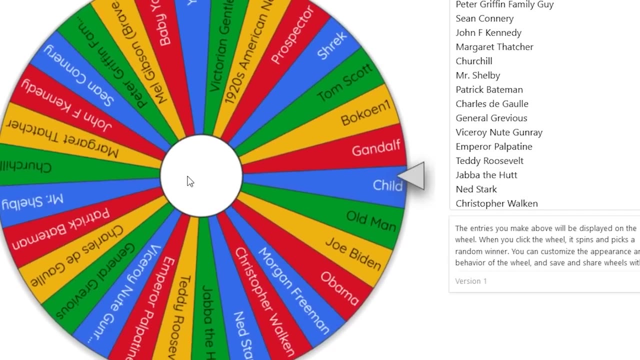 then if you can't answer no, what's the difference between a scottish man and a bench? a bench can support a family of four. yeah, yeah, that's good. uh, peta joe is now a child. you have to do a high-pitched voice. no, no, no, no. i. i said, i said baby, not hoy four player. 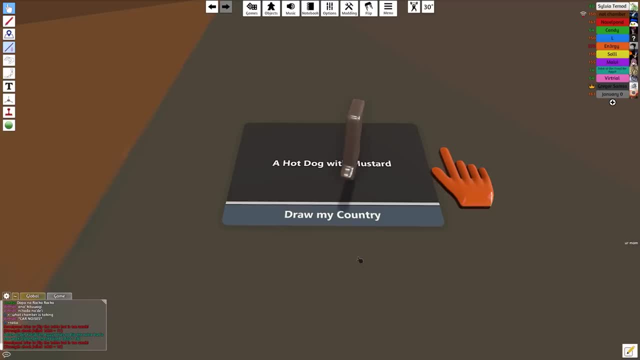 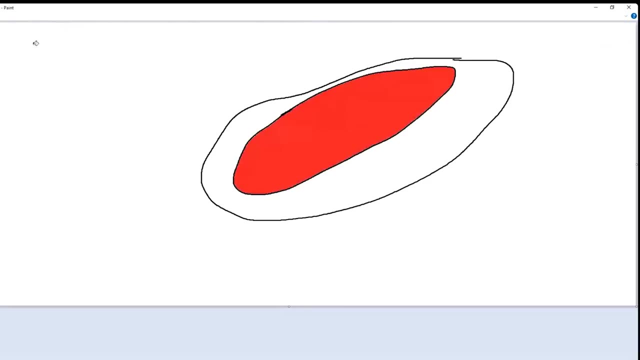 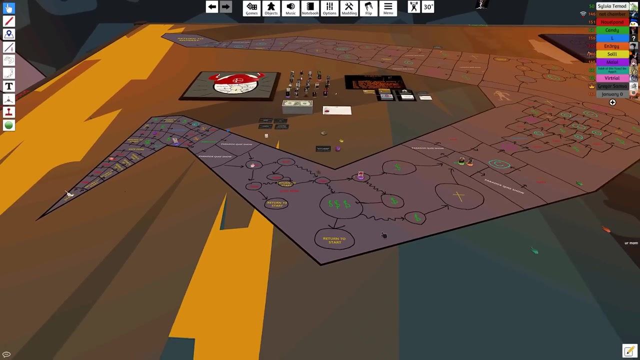 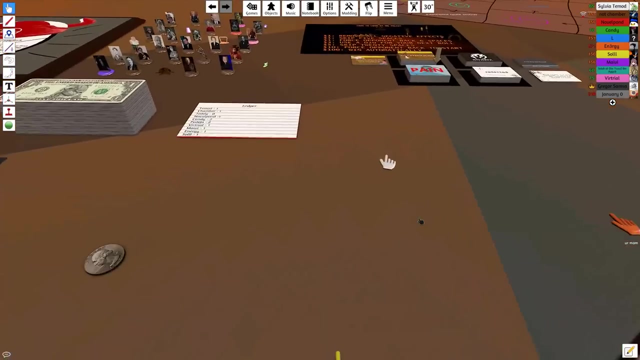 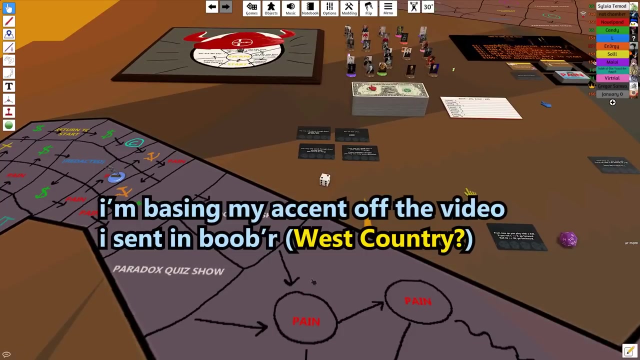 there you go, open, open paint. i want to see a hot dog with mustard. you're drawing my country. now, be advised. the everyone returns to start card is still there. so i i would advise avoiding paying cards at all costs, but it's up to you. no, no. 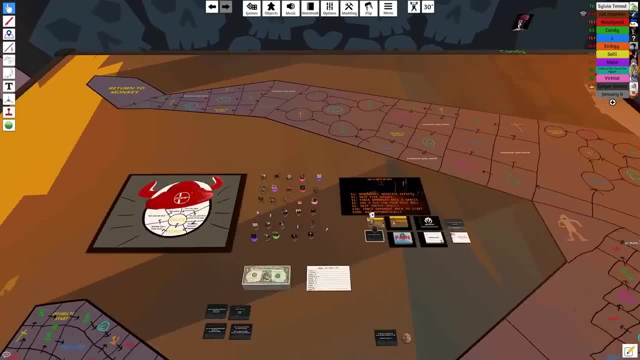 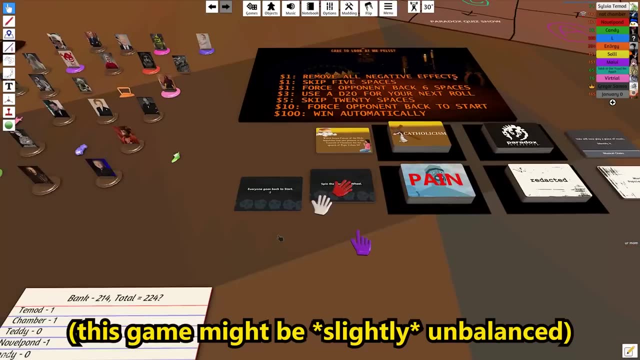 this is hour four and the game has just reset, however, all right, all right, look, because it is hour four, i am now going to remove this card from circulation. i this means the game will end. yeah, because it we're burning through pain cards too quickly. um, yeah, yeah, yeah, yeah, yeah, yeah, yeah. 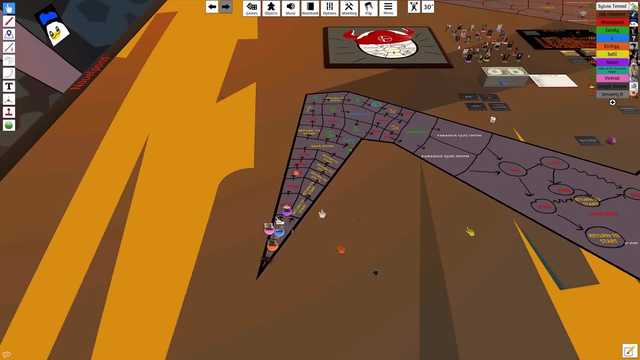 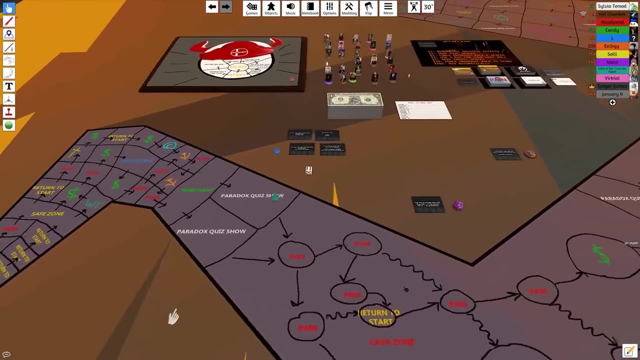 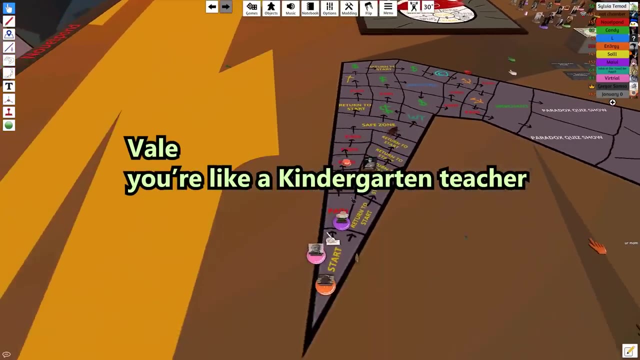 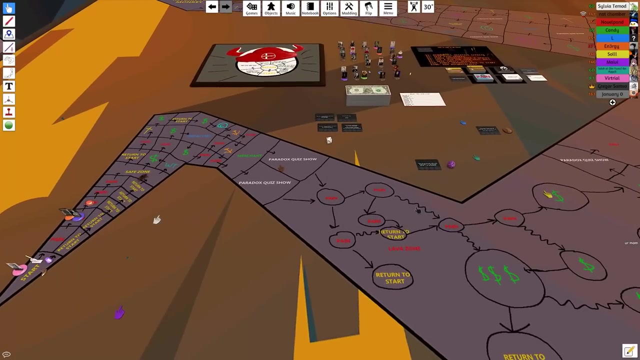 do you want a card down? it's waiting on candy. oh, i deeper anything. why are you making these noise? oh, west country, right, you just rolled charles to call bill. you're like a kindergarten teacher i am. my brain is melting from candy's speech. yeah, i couldn't understand anything. are you ready for something bigger than mine? 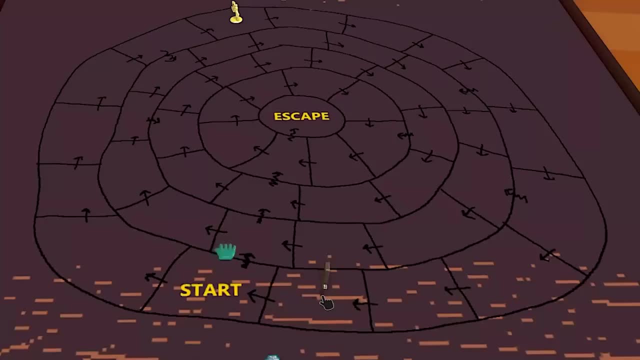 hate room movie chips. Hey, you're here. What you're trolling? Where are you Here? start the crypto. We all went back to start the crypt board- Yes, so I think yeah, and then you went all the way around: No, no, that's not how it worked in the book on board. 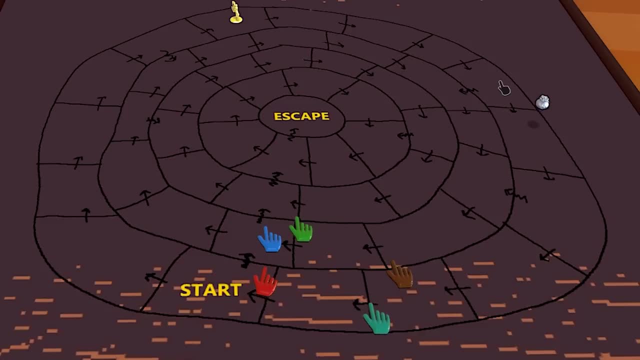 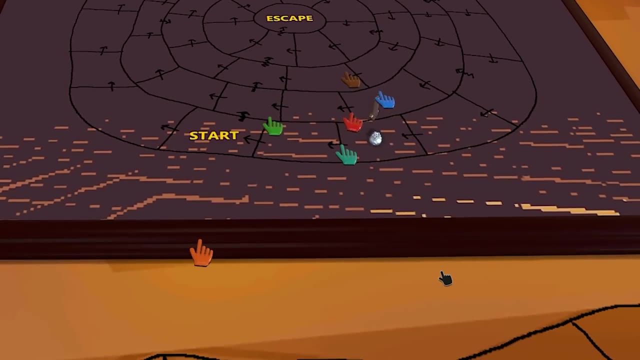 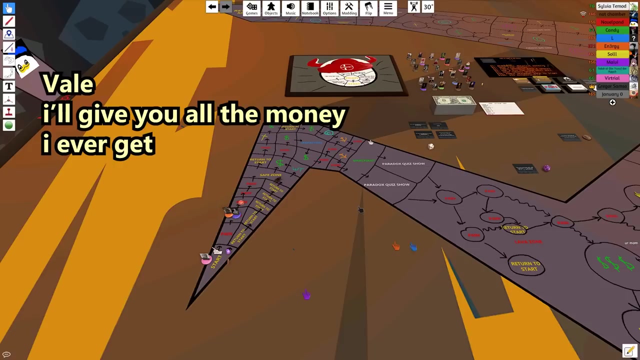 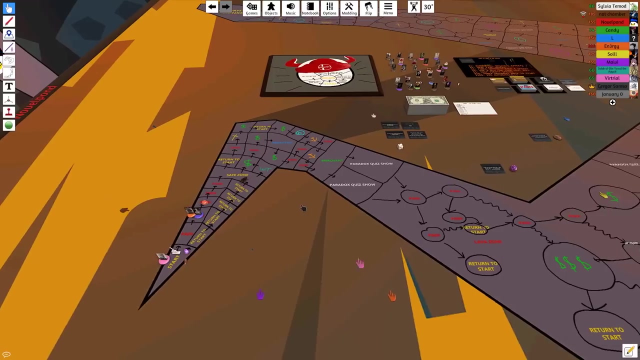 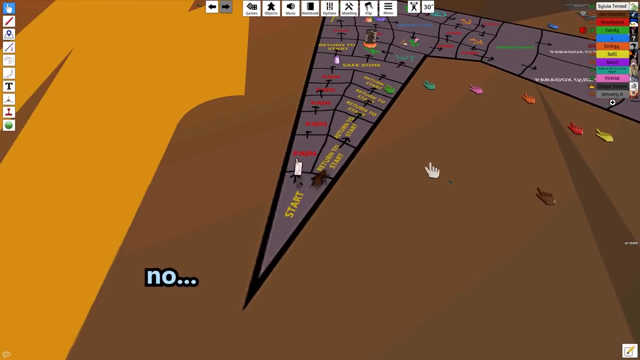 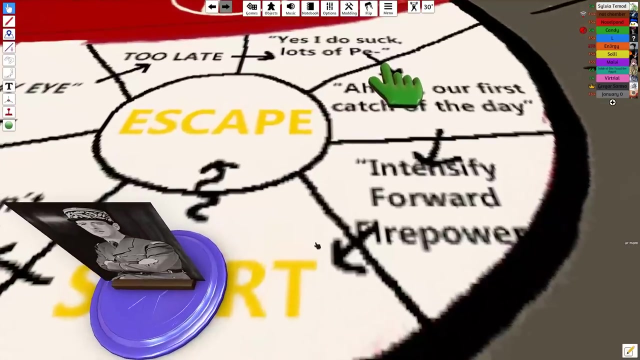 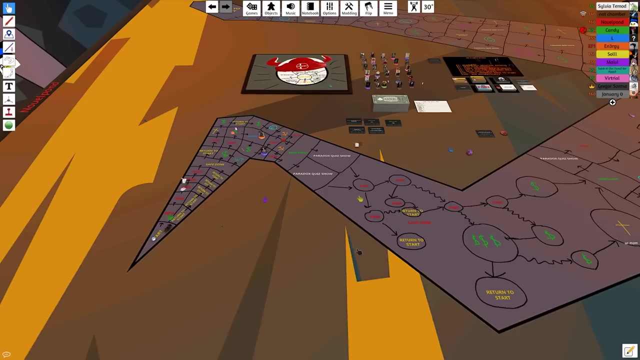 Making it work this way. You have to go this way, All of your fate. it's virtual stern. Yeah, we'll give you all the money I ever get You go to clown board, huh, To clown board. Avid vocal in one subscriber, Charles de Gaulle, I'm not gonna lie, chose the goal is kind of sus. I think it's something. 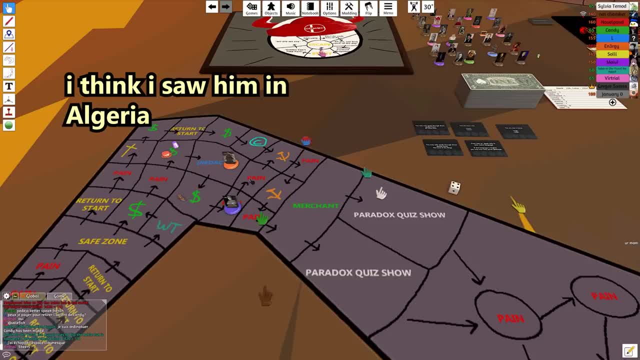 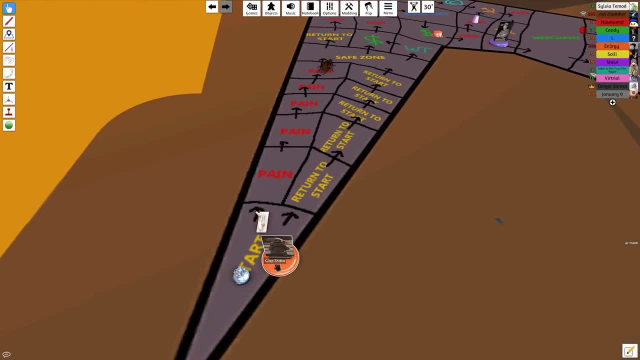 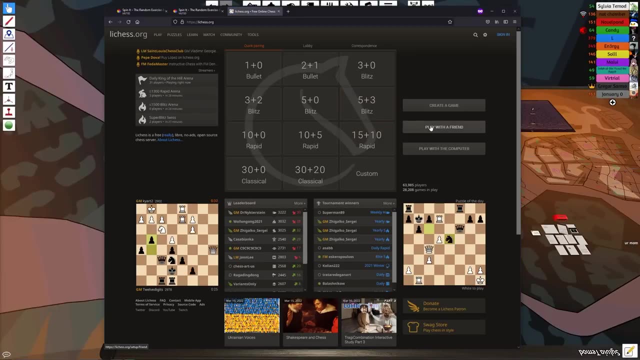 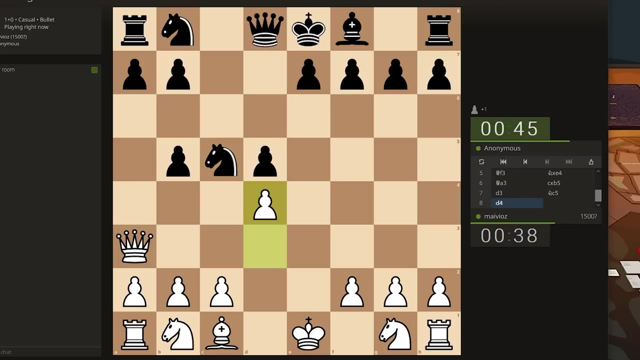 chamber Maybe needs to play a game of bullet chess against either Tmod Teddy or The fear of loss. is a path to the dark side available? Why did you just take it? Oh, whatever, it doesn't matter now. No, you've missed it. You hug your queen. 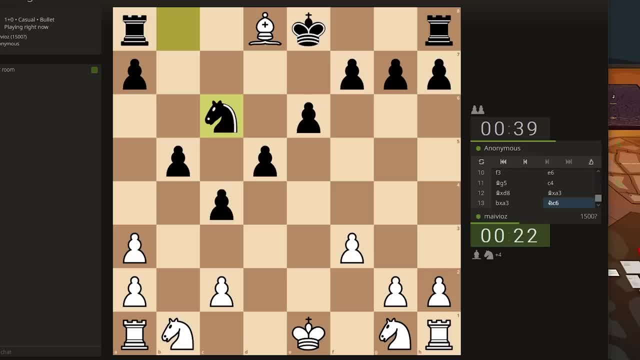 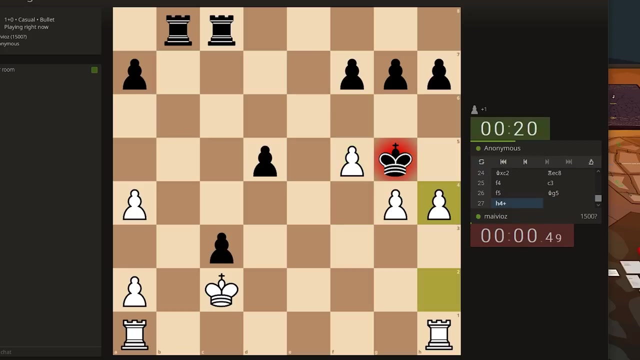 I'm so confused. What's going on, My god, you don't know what I'm doing. all Tactical genius try and flag in. maybe just move really fast. not fast enough. oh you're king. not nearly fast enough. alright, chamber wins swap places. you get to go to the crypt board for losing that. 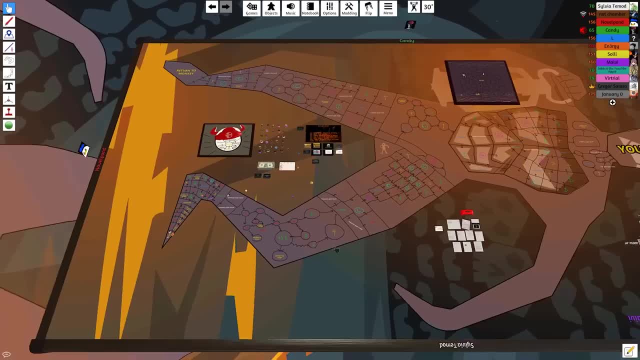 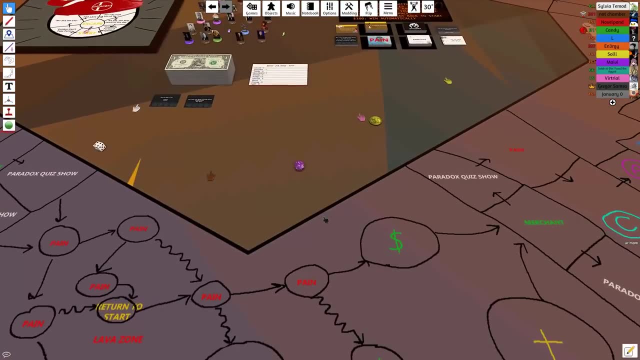 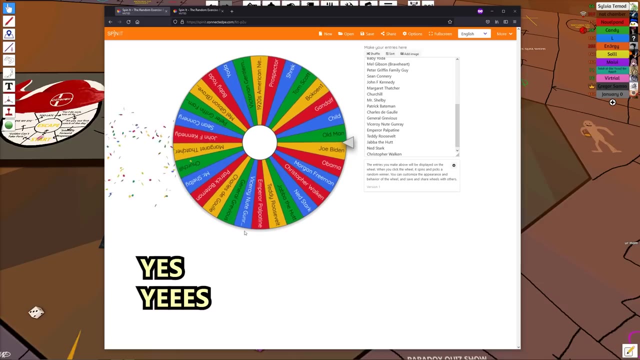 what? yeah chamber was on the crypt board. oh, you swapped places with them. oh, that's so bad. yep, oh god, teddy is spinning the wheel. it's- uh, it's joe biden. yes, sam, just go play 2048. your turn is skipped until you get it. 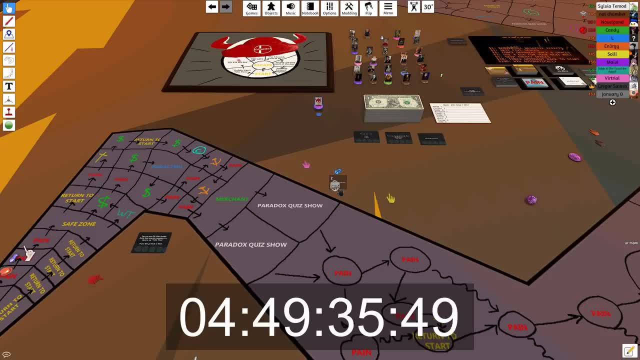 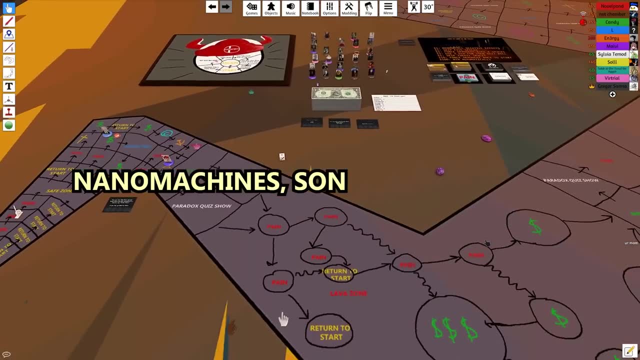 um, sorry, i'm done. i know i'm losing it as well, but we're so close chamber's going to win at this point. unless chamber pulls a last place swap card, uh, he's gonna win. metal machine. son joe biden quote: i'm going joker mode. 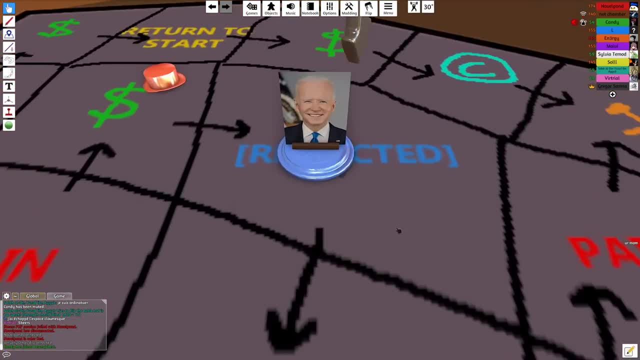 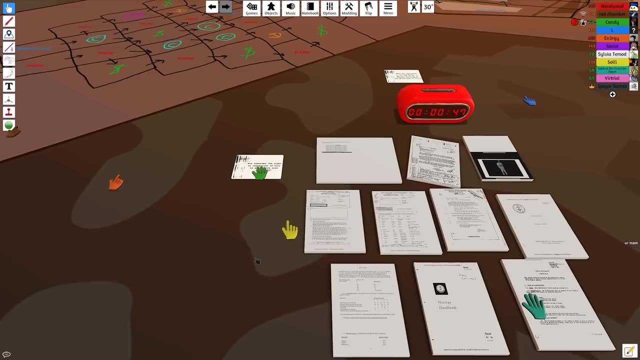 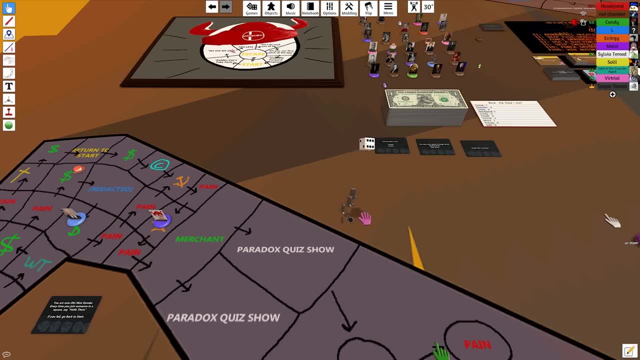 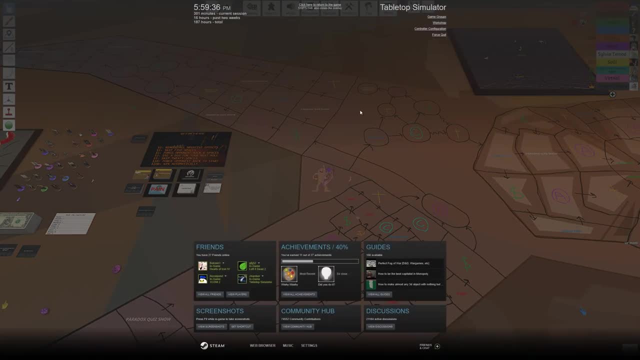 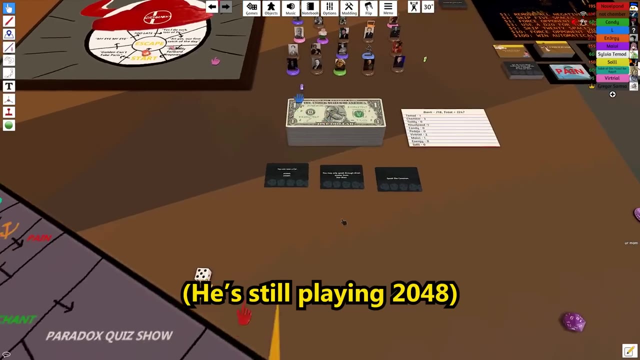 you should try fighting for what you believe in some time. jack, return to monkey, to my crotch. it is it's hour five and he's the first one to get halfway down the board. new joysey, new joysey, new energy. are you done? i'm not done. 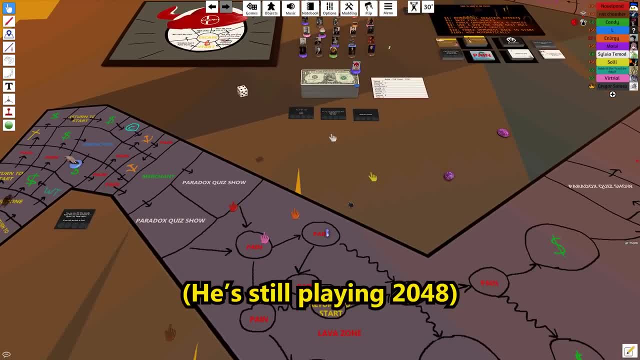 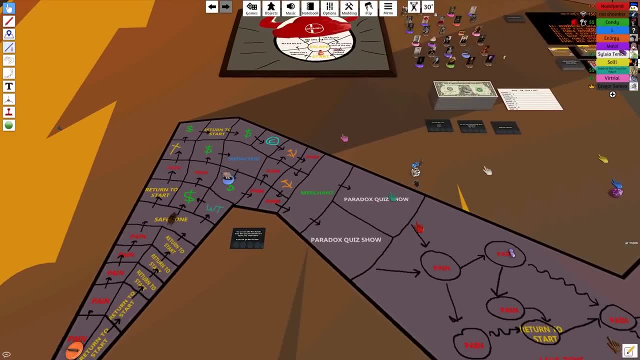 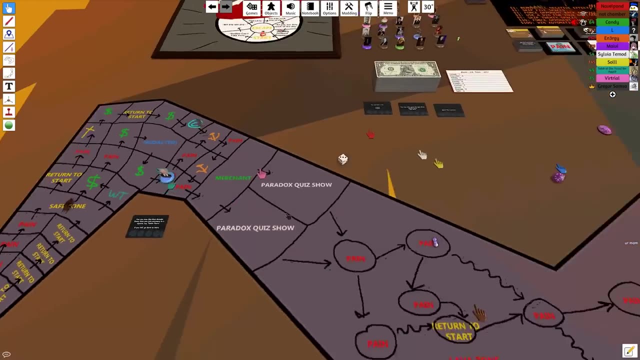 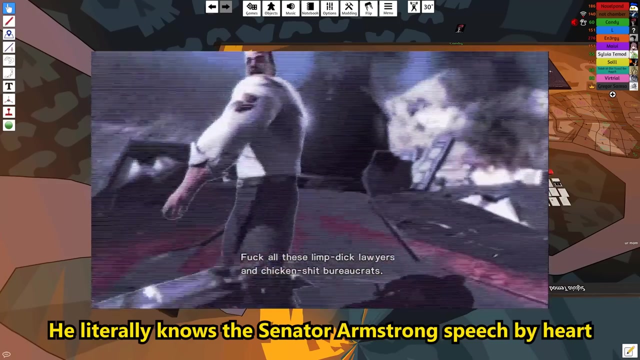 i'm still playing 2048. it's um. i keep losing. it is now teddy joe. joe, university of texas could have gone pro if i hadn't joined the navy. free communism in the hands of the people, where every man is free bureaucrats. fuck this 24 hour internet spew of trivia and bullshit. fuck american pride. 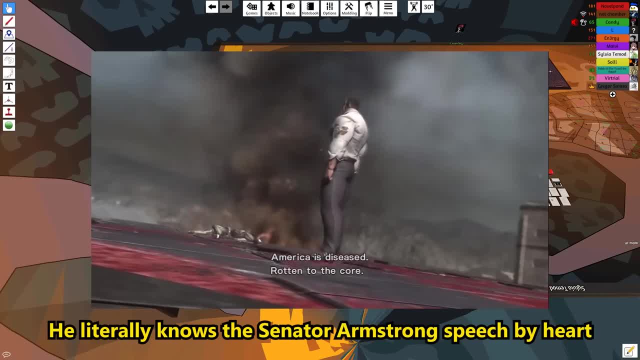 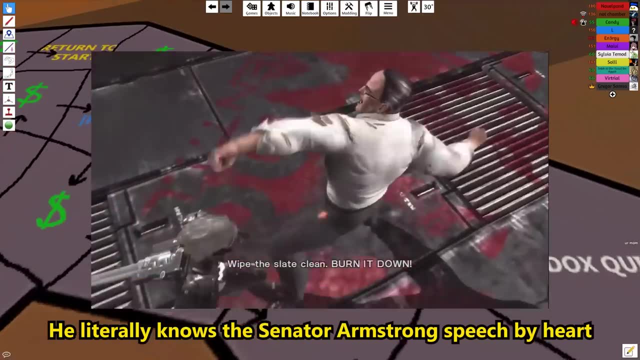 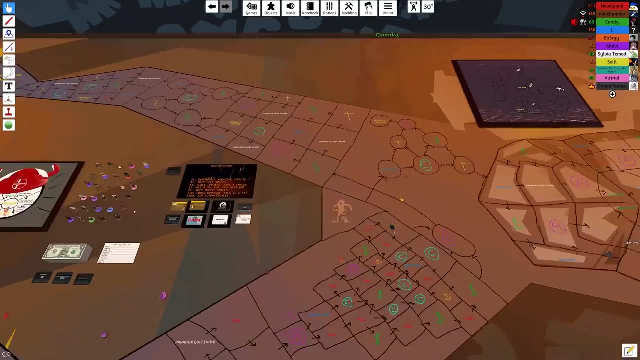 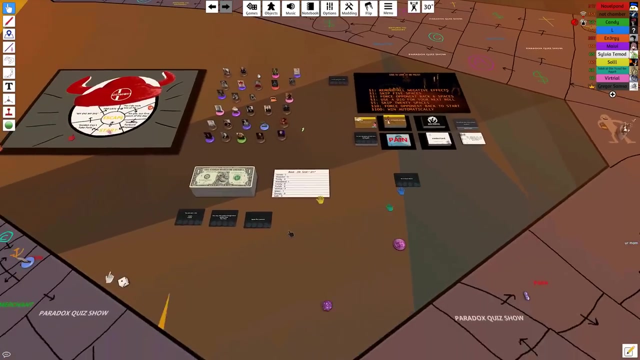 fuck the media, fuck all of it. america is diseased. right into the joe biden, right there, he's just go back. yeah, you still have to get past the two circular things. go to client. good, joe biden has been sent to bo cohen. one is he's in clown land, fuck no. 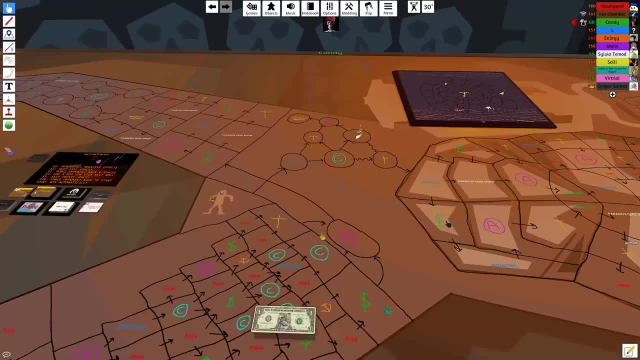 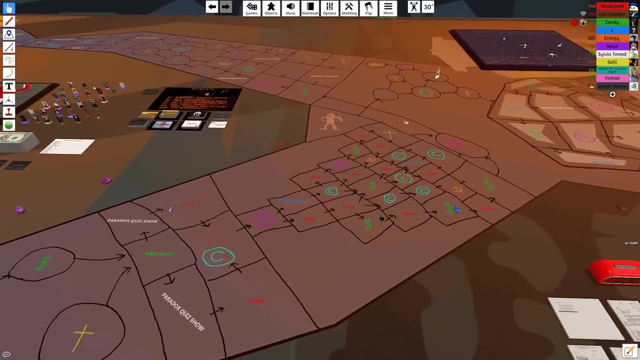 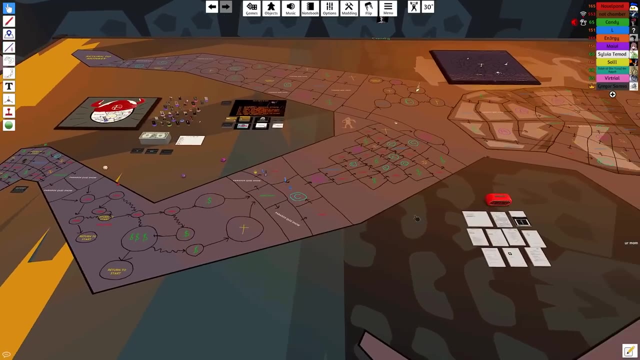 you most aggressive 2048 player. oh, he's sure he's through, he's gonna get through. someone paid chamber to go back six spaces, please, please. no, we're late, we're. let's just have a look at where everybody else is on the board and see if anybody has a chance. uh, pettish is the closest and he's at least a full. he's a full. 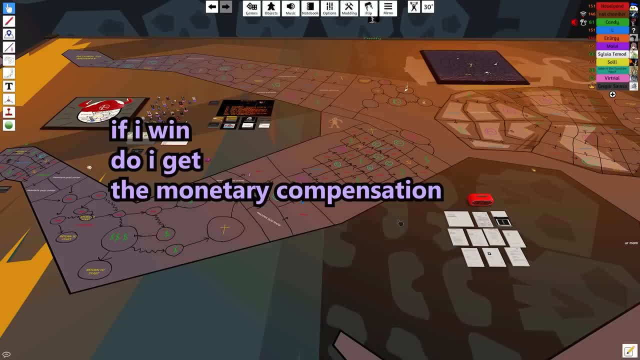 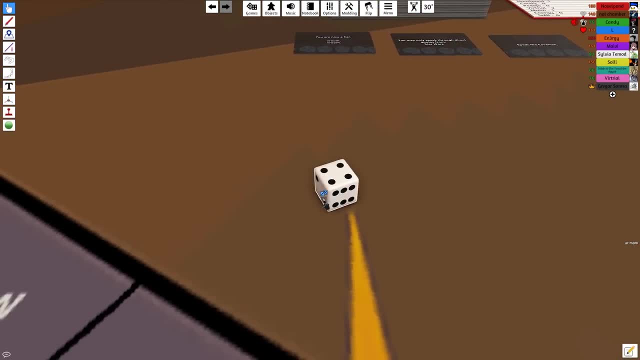 leg and thigh away. if i win, do i get the monetaries compensation? no, no, chamber, chamber. money for playing my board game. you didn't pay for it. do you remember what i told you? the tunnel i don't have you believe? he's still fucking doing this. 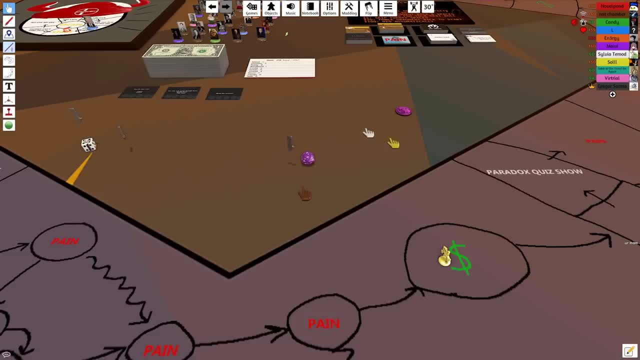 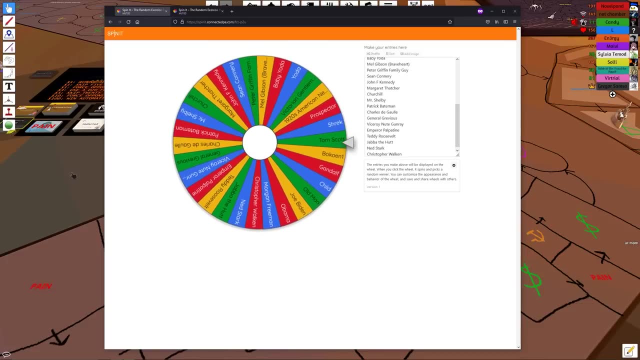 we're coming up in six hours of fucking fugitive quotes. richard, i'm sorry, but i'm in the middle of this speech. i forgot we've got two of you. i know i fucking give up on this piece of shit. okay, sam, stay in here. no, no, i'm not leaving, i'm just not playing 2048.. okay, but you can't. you can't play. 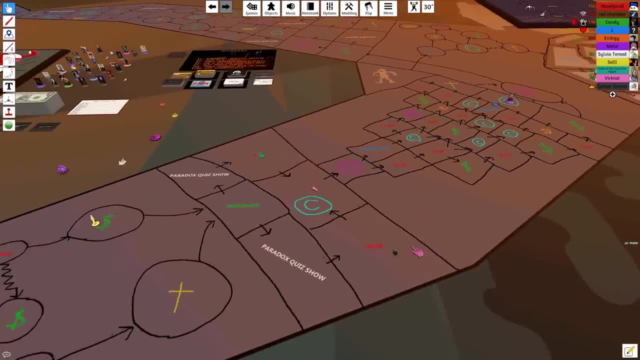 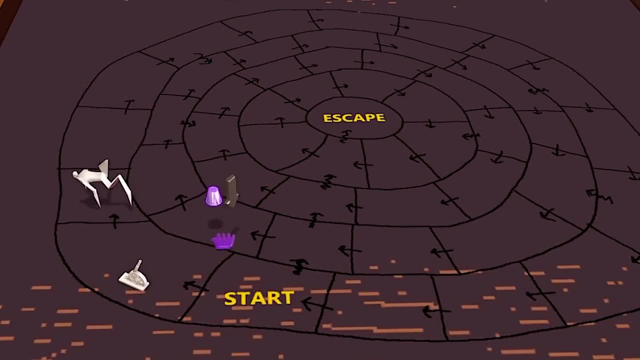 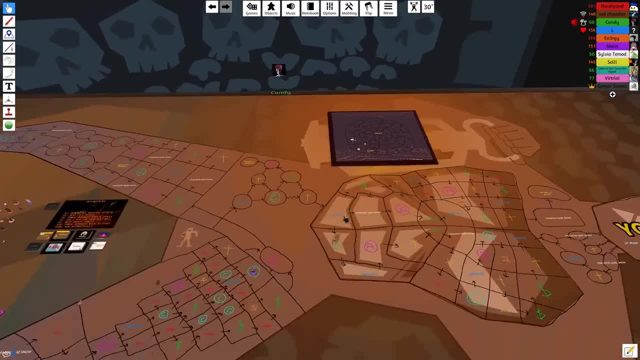 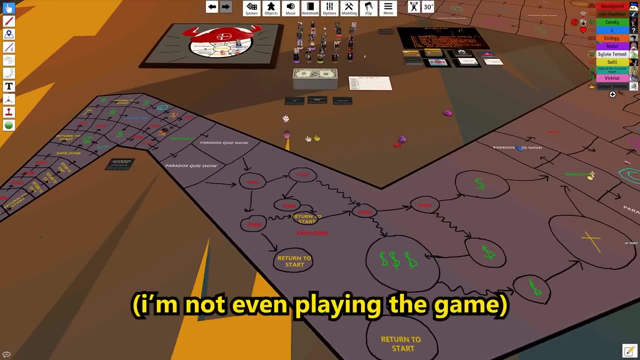 not end. it does not end, it does not end. help me, help me, help me. that's fun will never end the fun. will never end the fun. if you think that's a play, if he thinks this sucks to play, imagine just beat sitting here and trying to keep the game going and that's all you're doing. that's all you've done for. 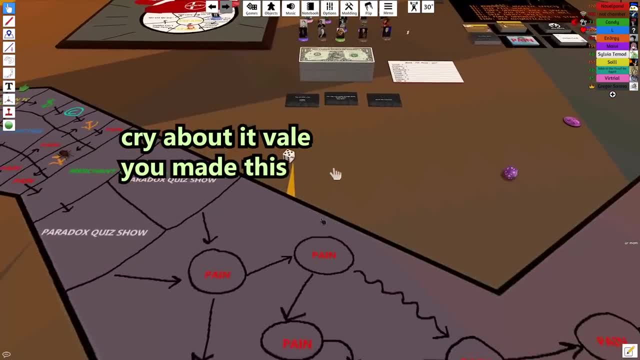 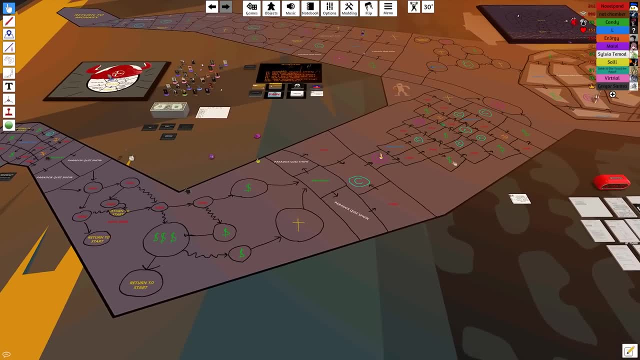 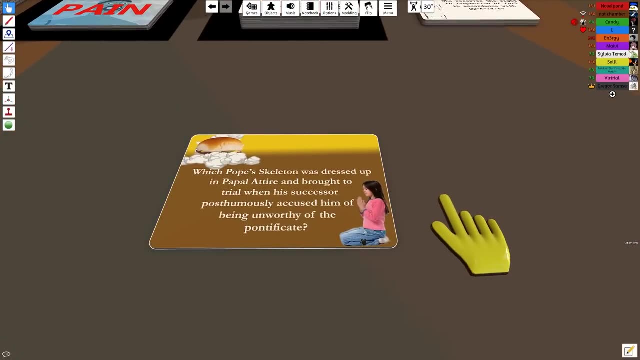 six hours. you made this. i didn't make this plan. no, nope, uh, chamber, chamber, our favorite friend, everyone's favorite chamber. roll the dice, please, please, go forward, please go forward. christ, you are on, christ, i hope you're ready for a good catholicism. which pope's skeleton was dressed? 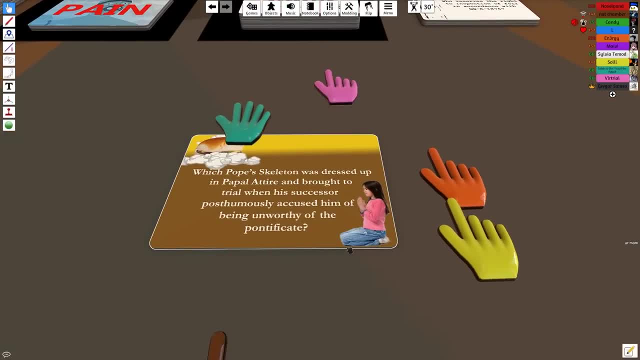 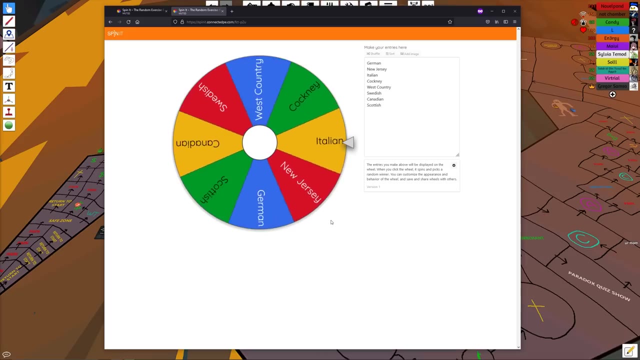 up in papal attire and brought to trial when his successor posthumously accused him of being unworthy. i've mentioned this before, but do you remember his name, john the eighth? no, his name is formosis. uh, moses, yeah, very unique, uh pope name. actually, pedigree you're doing, caught, you're. 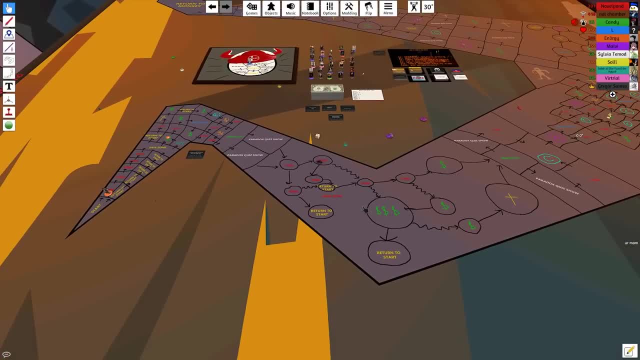 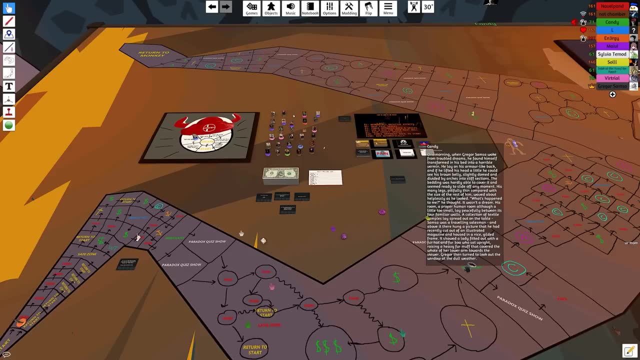 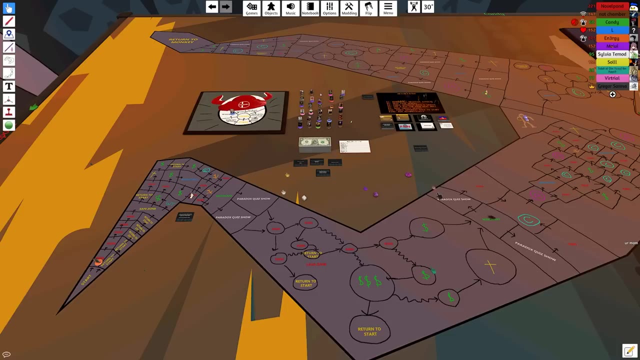 doing cockney again cockney. there's a guy on the phone claiming to be richard kimball. thank you, it's. it is teddy. we cannot let this. we've never allowed any crisis from a civil war straight through. i will- you don't roll the dice, i will one, two, three. you're a character, now candy. 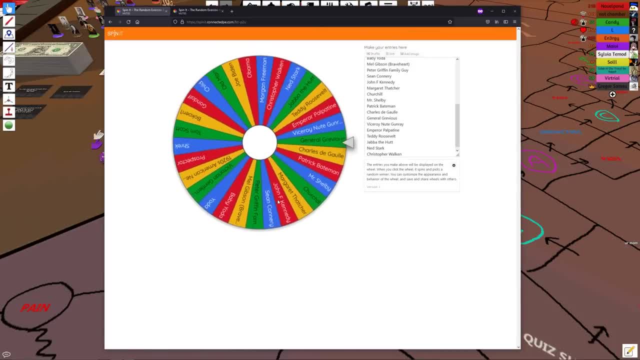 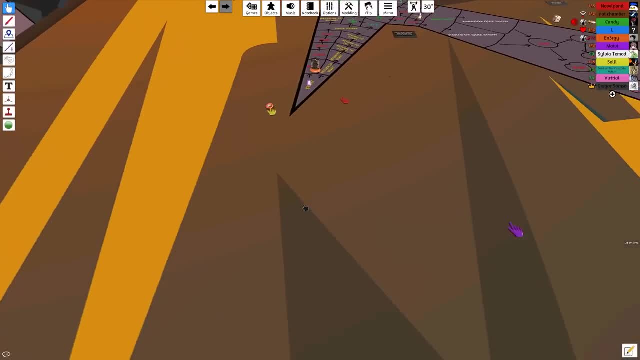 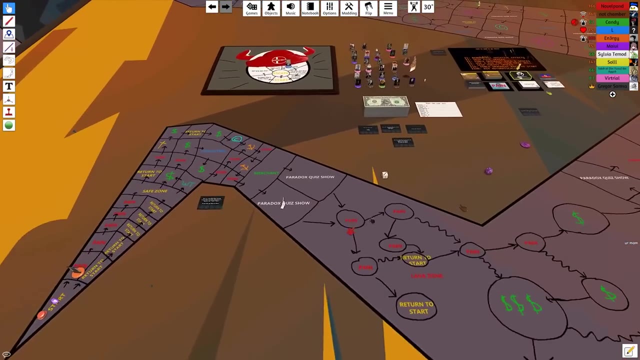 oh, what character i'm rolling the viceroy, newt gunray. yeah, are you brain dead? i'm not going in there with two jedi. i didn't kill my wife. it's so funny after six hours. i didn't kill my wife, it is. did you kill your wife? 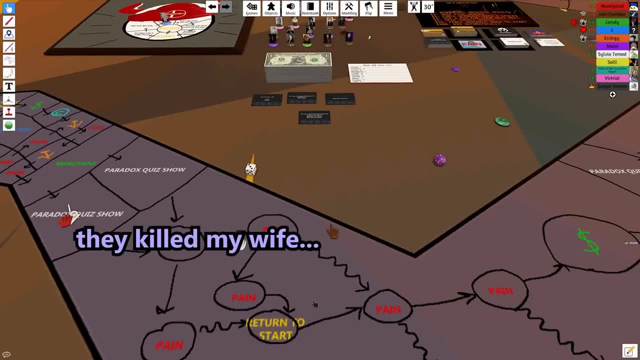 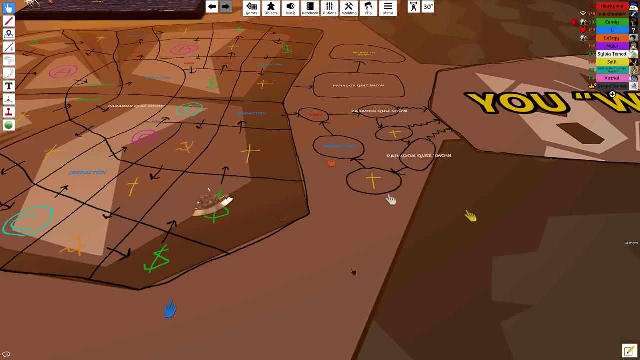 they killed my wife. who's they? it's like: hey, did you kill your wife, yet roll the dice, please, richard. here's the part that gets interesting right, because the ending of the game is different from how it used to be, because jan sent me a funny idea where. 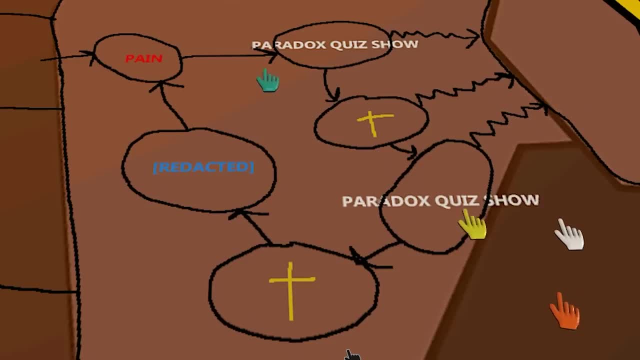 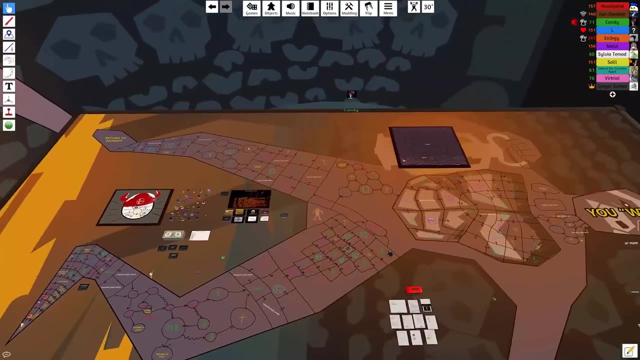 you get stuck in a loop until you land on one of those three. you need to get the person right. hey, we should. we should make it so that he lands on the pain guard and it's the person in the last place. so that means it's me and i go down. 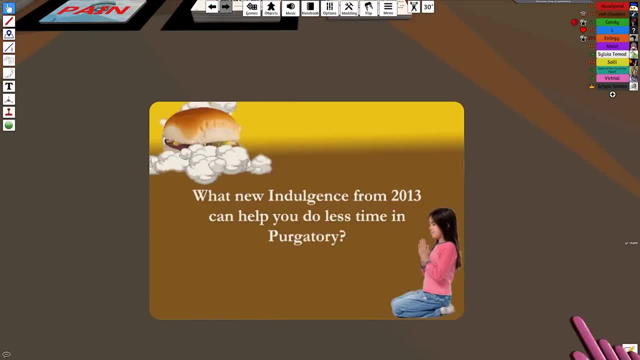 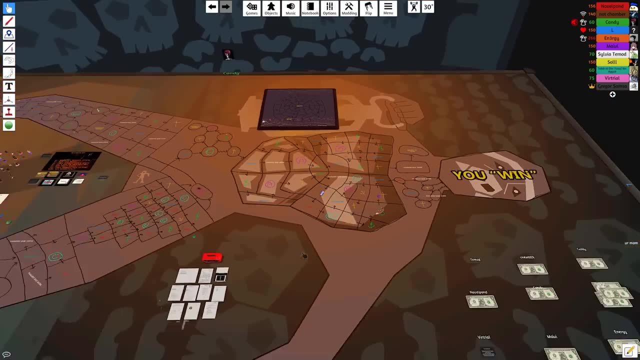 and out. you can answer this. you can answer this correct. what new indulgence from 2013 can help you do less time in purgatory? oh, it's, uh, the twitter account. true, yeah, true, go forward one. uh. if you follow the pope on twitter, you get spend less time in purgatory. 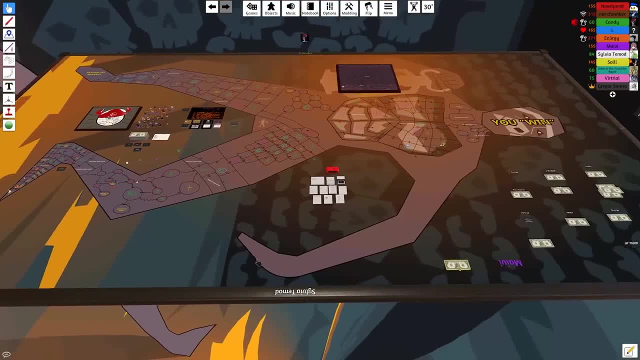 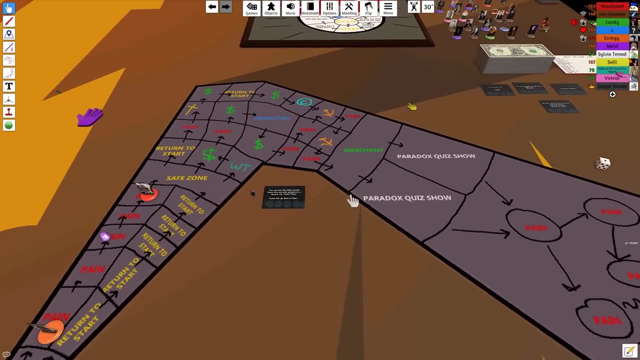 i love the bird. oh, i'm following him right now. i love the bird. oh, i'm following him right now. it's like i'm doing it right now. it's maybe a. you're the clown. you love the coin one. you love the coin one. you love the coin one. 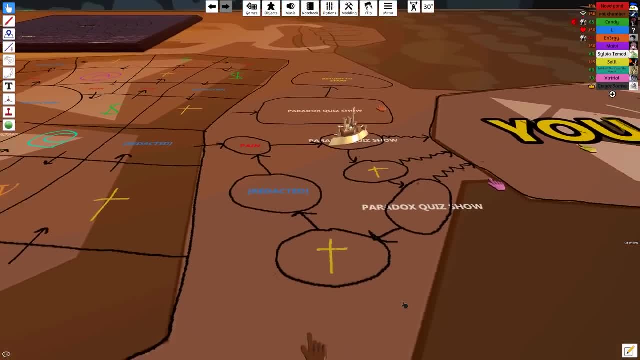 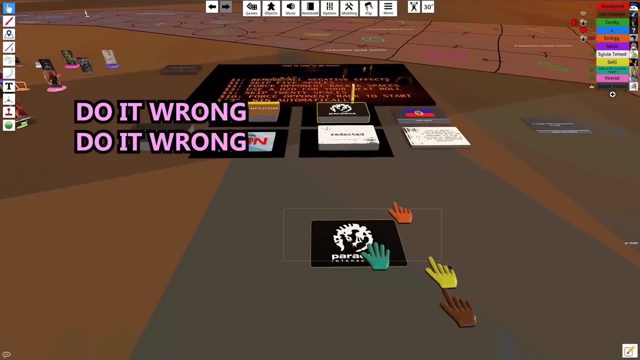 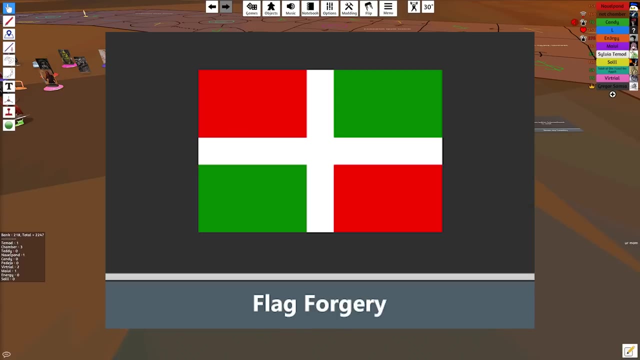 paradox quiz show. okay, chamber, chamber. if you get this right, the game ends. if you get this right, the game ends. all right, you ready, oh god. oh god, it's like a shanty or something. it is not madagascar, is this asapirindi? 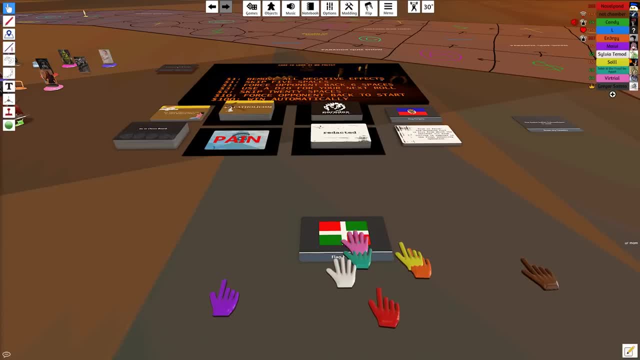 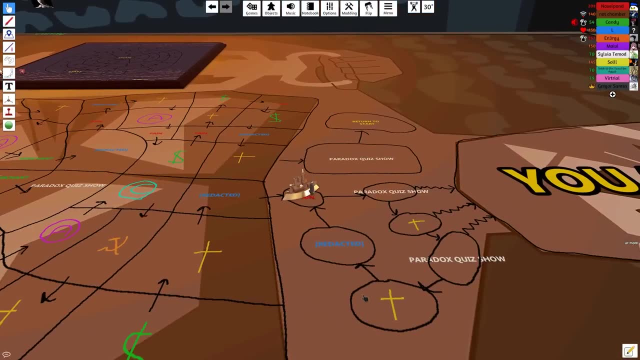 is it this one? yeah, it's um, it's uh betsimissarka. no, betsimissaraka from eu4. unlucky, he goes back. but the good news is he has missed- as long as he doesn't roll a six, we're fine. 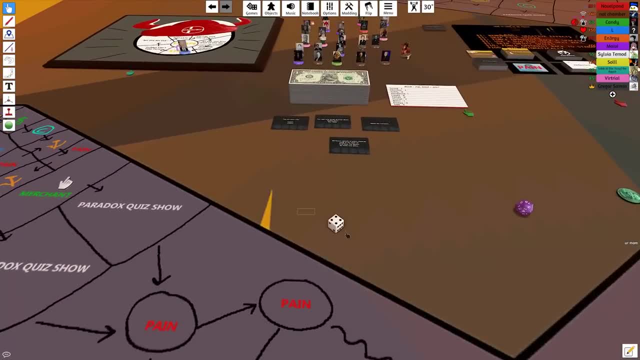 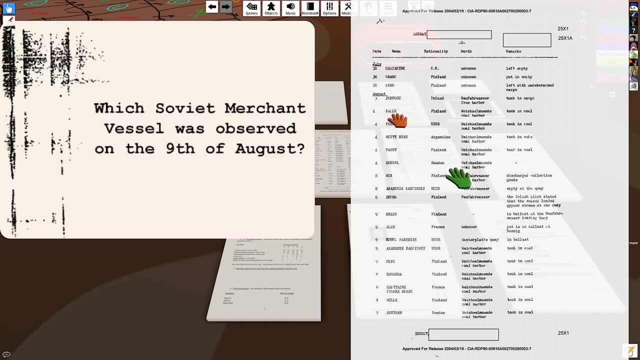 i hope he rolls a six and gets: uh, the thing where i win. i want to win. why are you on that? you're on the wrong page. you can answer any of them. there's multiple answers to this question: what, what, what? It's not a. 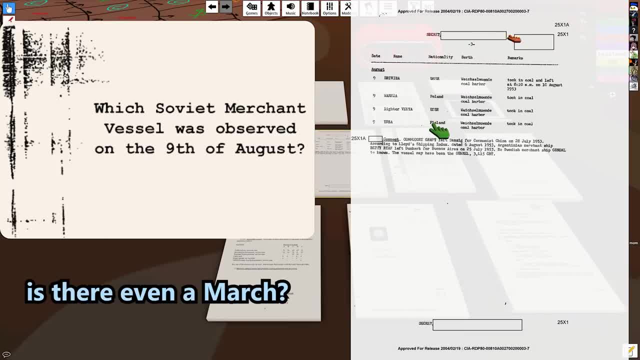 Is there one in March? What March? Where did you get March from? Read the fucking cards. It says August. Oh, 9th of August, March, March. You gotta say, you gotta say No, no, Oh, my God, Candy got it wrong. 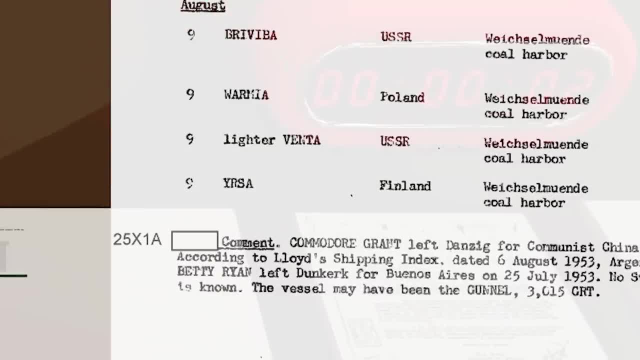 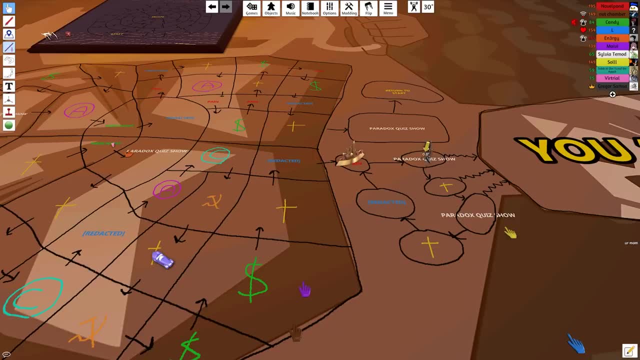 Soviet. That's Finland. It says Finland on it. Oh, I think I am going insane. 15.. Oh nope, Here's one next round, eh, Unless Chamber gets it by day. Chamber actually has to get it right. 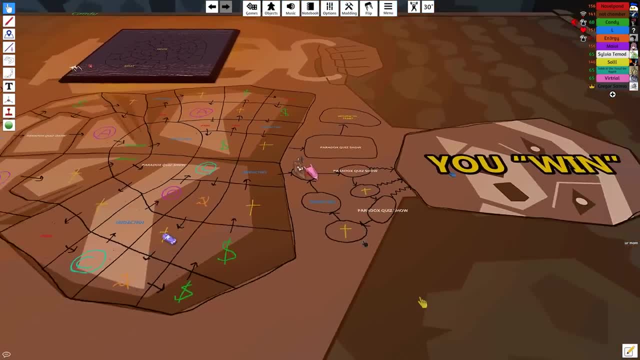 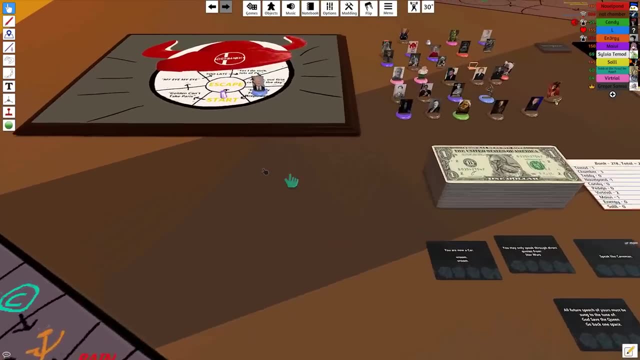 Chamber's been supplanted, Virtual's gonna win. So now they're both within the loop. Joe Biden, Joe Biden, Roll the dice please. Couldn't have joined the Navy if I hadn't gone to the Navy. Okay, if you get this right, you win. 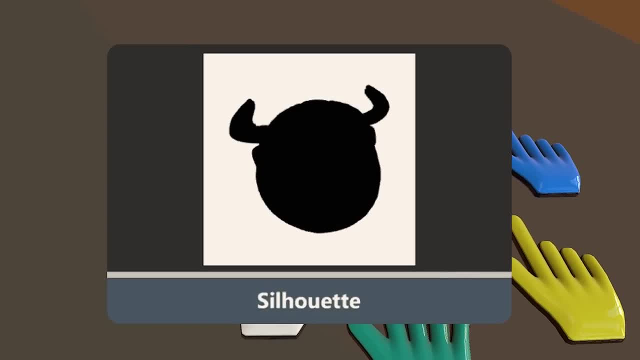 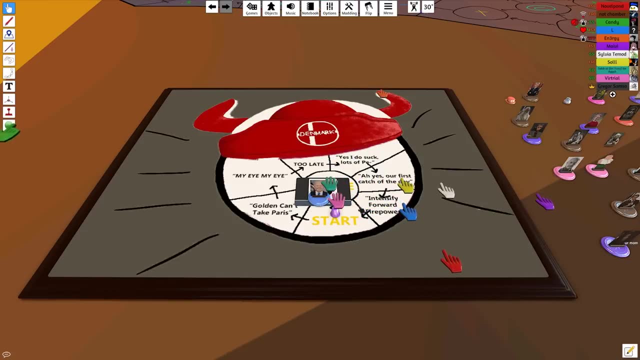 Turn, he can just roll. Oh yeah, that's true. Who is it Virtrail? Who is it Virtrail? I have a sneaking suspicion that this is Bo Cohen 1. I'm sorry that actually was Richard Nixon. 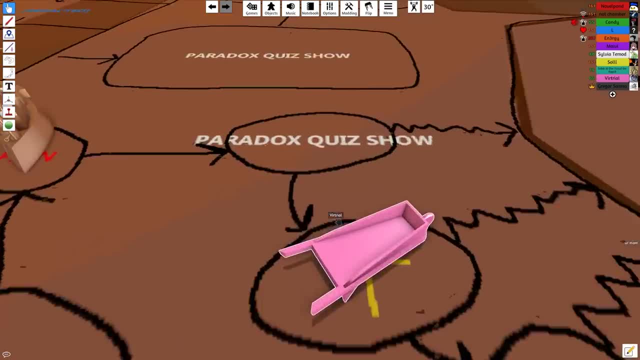 If you peel away the silhouette, his face is in there. I knew it was Richard all along. He's the one who did it. There you go, All right now. Chamber go, Chamber go, All right, this is it, This is it. 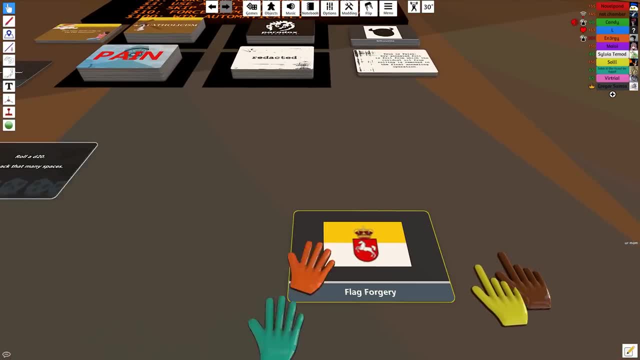 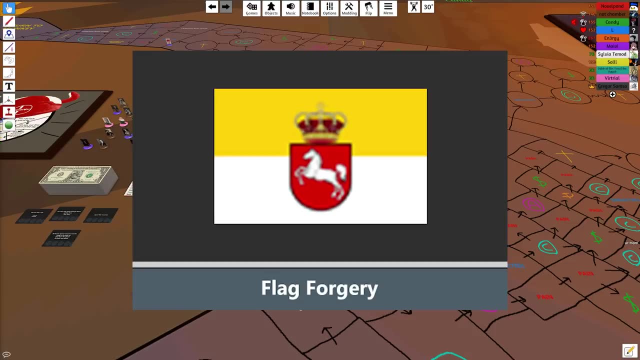 If he can get this right, he goes through. No, he doesn't. What flag? Wait, wait, wait, wait, wait, wait. What flag and what game? It's Hanover. From which day, mate? No, he's already wrong. 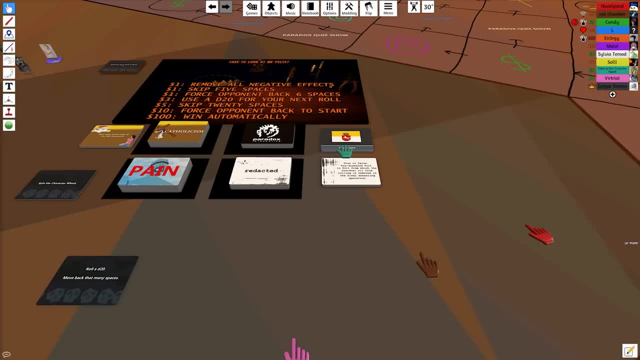 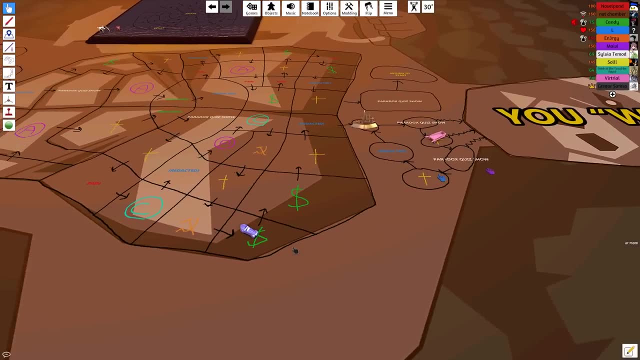 This is the Kingdom of Westphalia from Hoi 4.. You idiot, It goes back to pain. It doesn't make any sense. Kenny, please, We have three contestants in the running right now. We just need the rest of you fuckers to go. 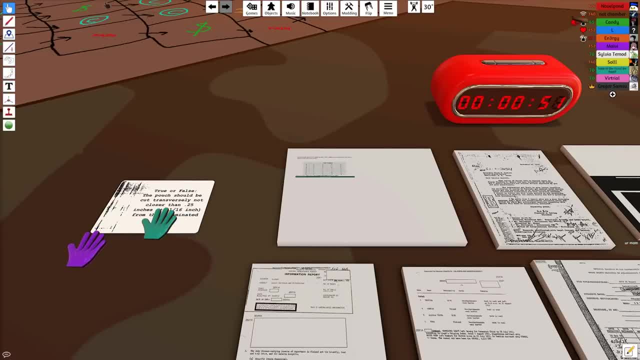 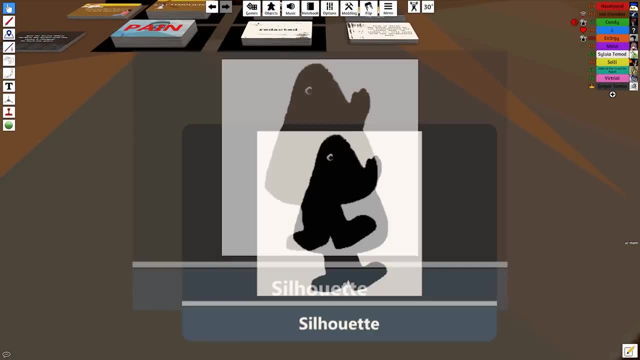 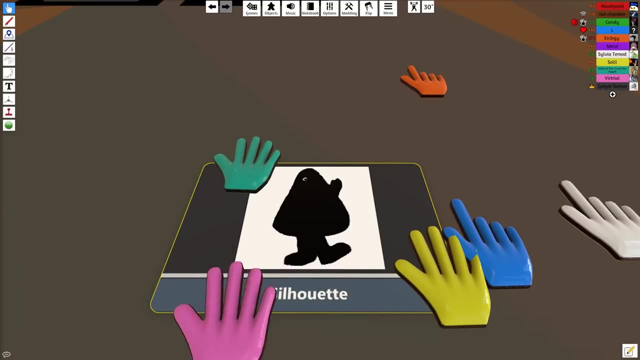 I have a dream That one day, Every person in this nation will control their own destiny. For fuck's sake, This is for the win. You've done it all. The deciding thing, Petitjoe, Petitjoe. I need you to tell me which.